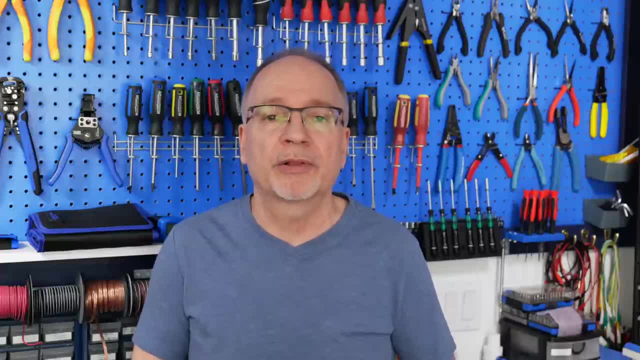 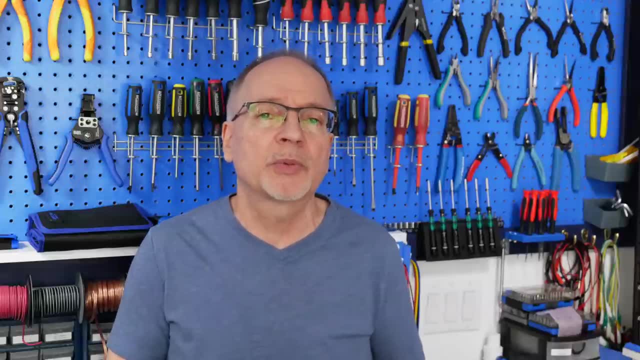 And object detection with microcontrollers is certainly a big part of that. Now, we've worked with this technology before. Several years ago we worked with something called a PixieCam, and this was pretty well the first hobbyist level object detection device that you could use. 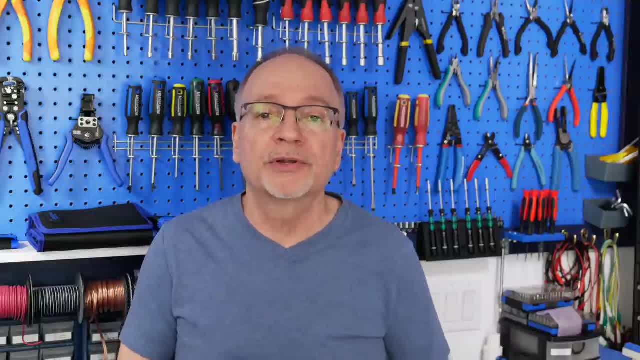 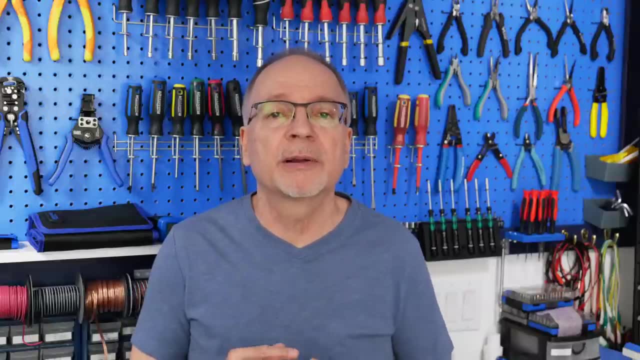 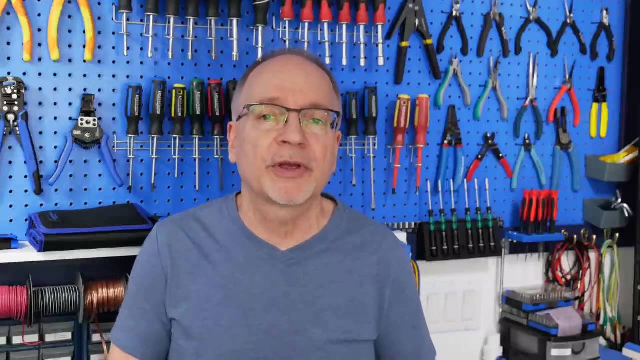 And it worked pretty well. A little while back we worked with the DFRobot Husky lens And this is an amazing product that does advanced object detection, image recognition and a number of other things. It has a little screen on it and it is powered by the powerful Kendrick K210 processor. 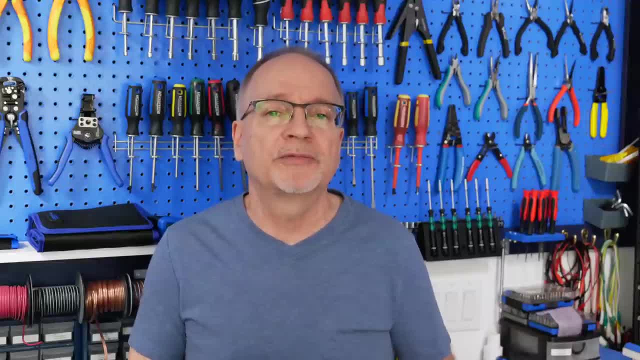 But there is even a cheaper and more simple way of doing object detection and we're going to do that today. We're going to be using an ESP32 cam. Now. the ESP32 is not as powerful as the Kendrick K210. But we're going to do that today. 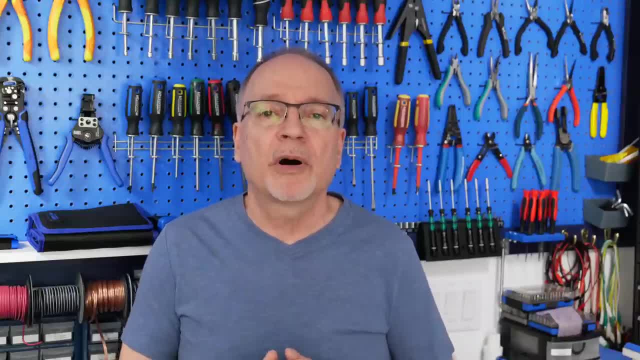 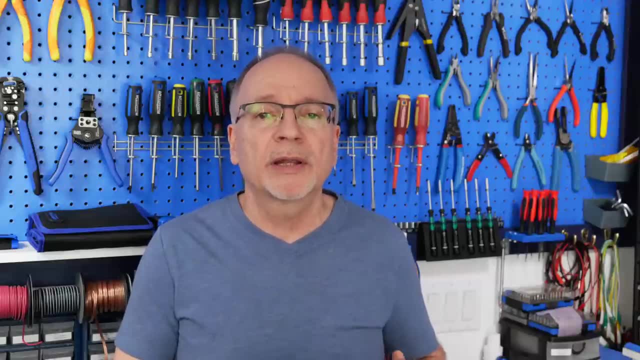 But nonetheless, it is capable of simple object detection. That's exactly what we're going to be doing today. Now, we're going to be building a model and we're going to be training the model using something called Edge Impulse. Edge Impulse is an online product. 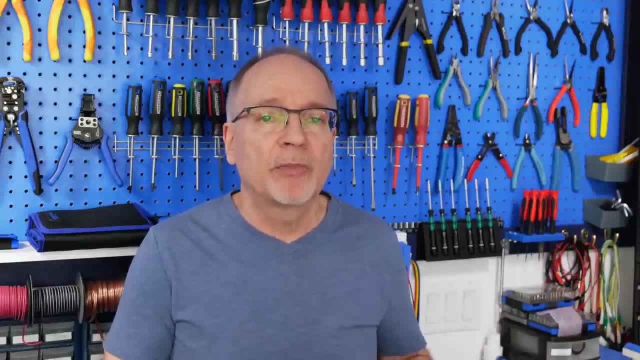 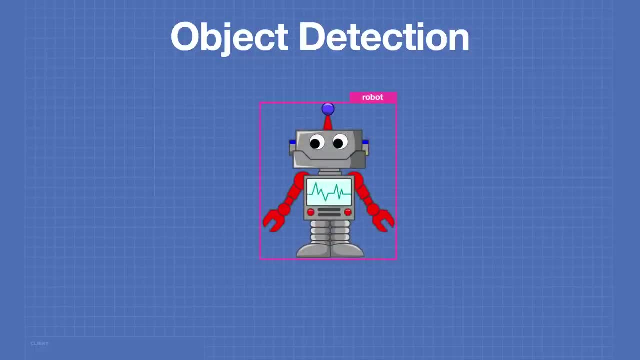 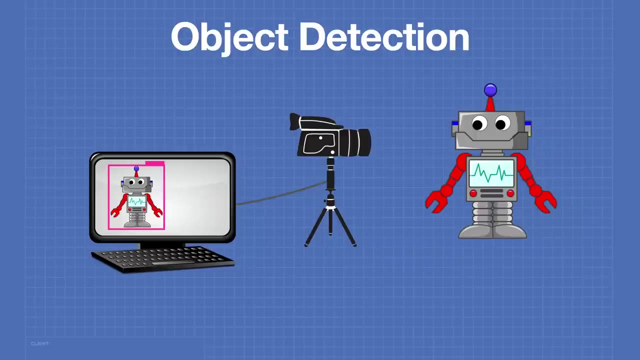 You can use it for free and you can use it to train models which we can then deploy to the ESP32.. So let's get started by learning a bit more about object detection. Object detection is actually a combination. There's actually a combination of two different imaging techniques: image classification and image localization. 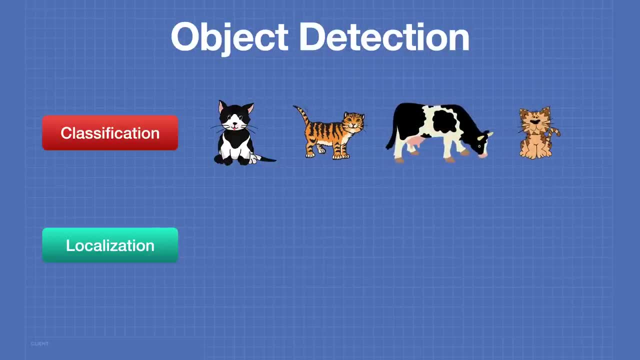 We can use these four pictures to illustrate image classification. Now, here you see images of four different animals, But for an image classification system there are only two classes: cat and cow. An image classification system would make no distinction between the different cats. 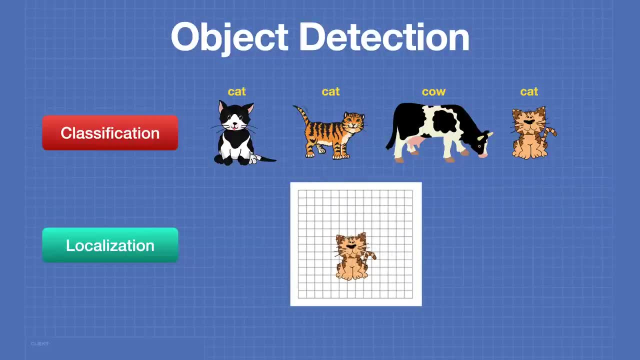 Image localization techniques are used to determine the position of the object of interest within our field of view. In many localization systems, this will be illustrated using a bounding box, which is a box that surrounds the image. In many microcontroller-based systems, we simply use the XY coordinates of the top left corner of the bounding box. 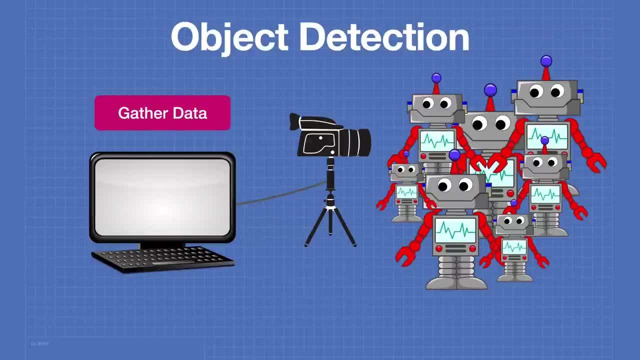 The first step in any object detection project is to gather data. This involves gathering a number of images of the object to be detected. This can be done using a camera or it can be done using an image bank, and it is not uncommon to need a hundred or more images of an object to get an accurate fix on it. 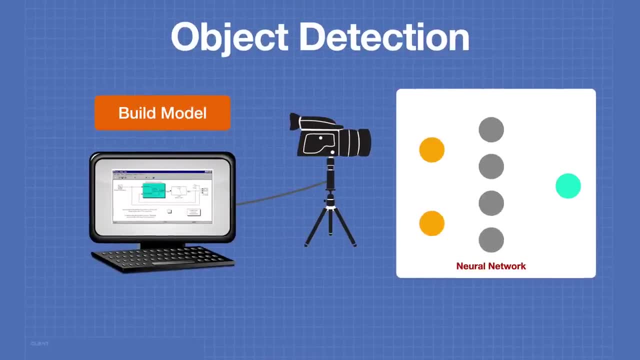 After obtaining and labeling our images, we'll use them to build a model which we can use to recognize the object in the future. We'll be building our model using a neural network, which is a network that consists of a number of nodes. 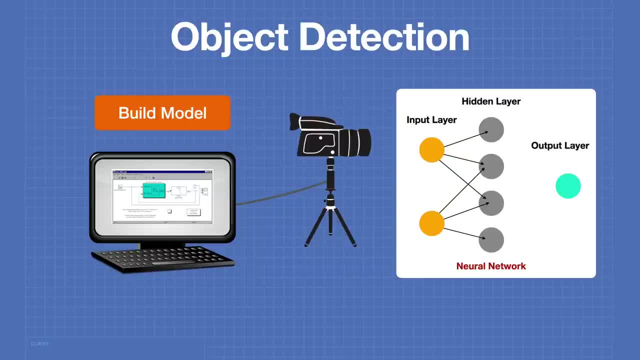 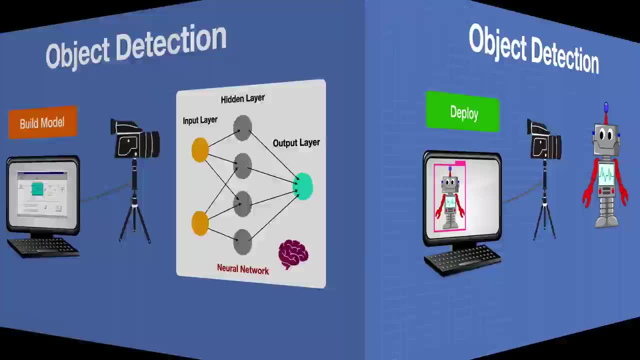 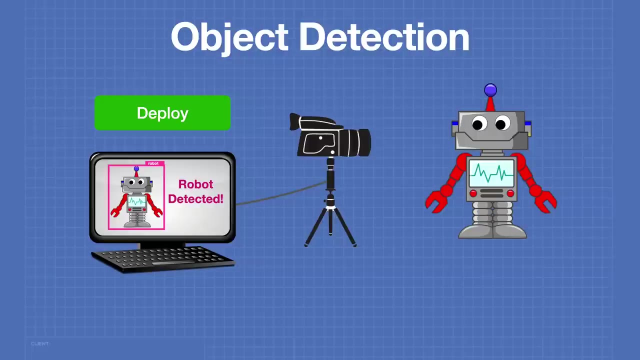 and neurons that have multiple outputs, which are then weighed to determine a response. A neural network functions in many fashions like the human brain. Once our model is built, it can be deployed into production and used to recognize the object. We can continue to train the model in order to improve its accuracy. 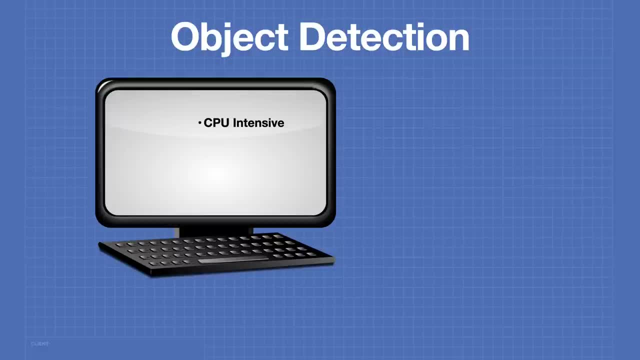 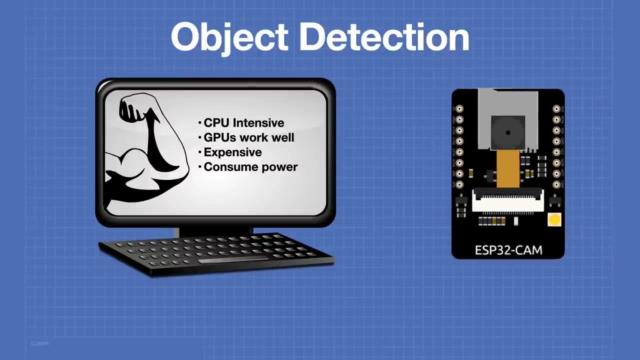 Object detection techniques can work quite well, but they are very CPU intensive. In many cases, GPUs are employed for this sort of work. This can result in a very expensive piece of equipment that can also consume a lot of power. Now, with all of those requirements, how could we possibly do this with an ESP32?? 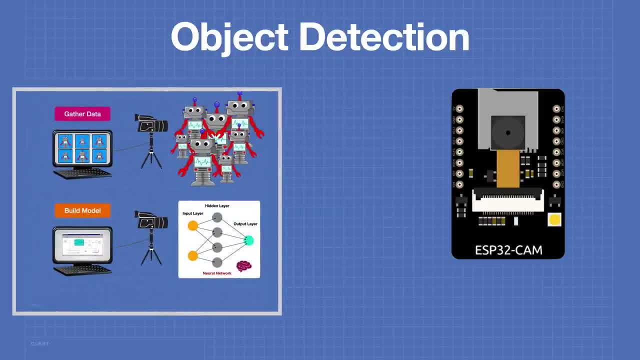 Well, the answer is that we do our data gathering and model building offline, on an online service or a local machine, and then we export the results to a tiny ML or machine learning code. We can use that tiny ML code to build an ESP32 library and some code that we can then run on our ESP32 CAM. 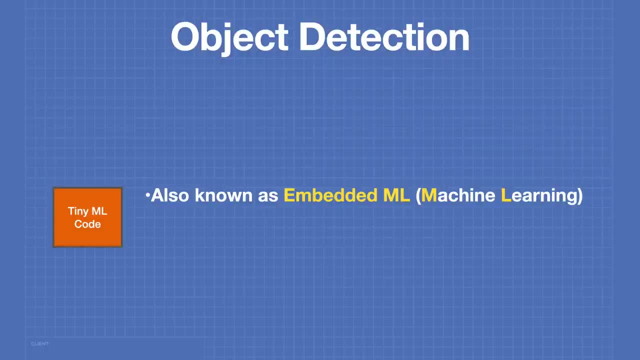 Tiny ML is also known as embedded ML, with ML meaning machine learning. Tiny ML allows you to run machine learning workloads on a microcontroller. This technique is used with edge computing and IoT devices. There are many methods of creating tiny ML code. 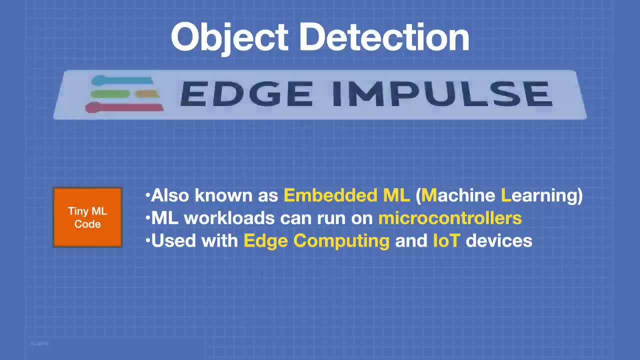 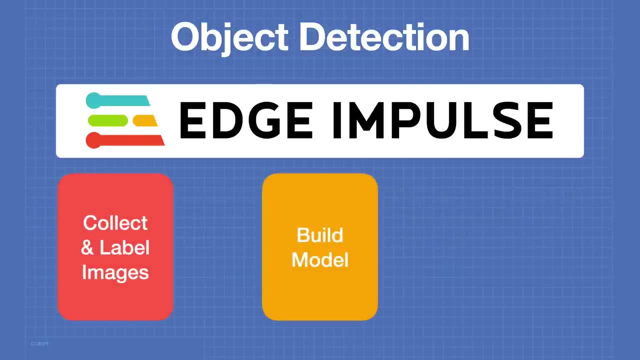 and the method we're going to be using today is a product called Edge Impulse. Edge Impulse will allow us to collect and label our images, build a model using a neural network and deploy that model to an ESP32.. Edge Impulse accepts multiple data sources, such as video, audio and analog data. 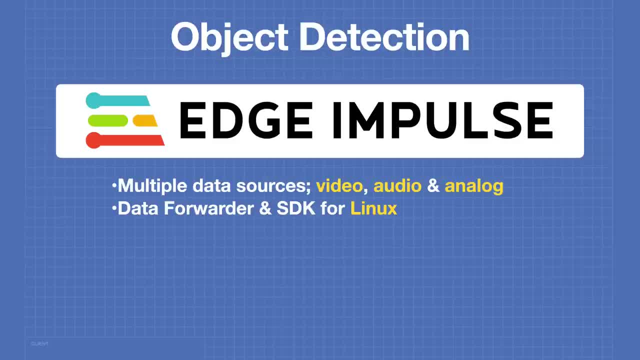 It has a data forwarder and SDK for Linux so it can be used with a Raspberry Pi. It also exports to an Arduino library with sample code and this is what we'll be using with the ESP32.. Edge Impulse supports several different development boards. 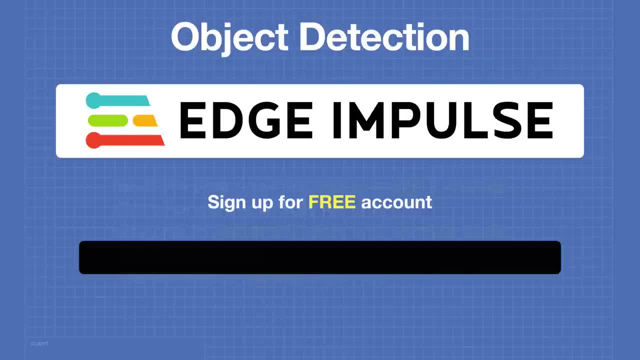 It'll also work with a computer or a phone. To run the experiments we're doing today, you'll require a free Edge Impulse account. so go and sign up for one and get some objects out that you want to detect with your ESP32.. 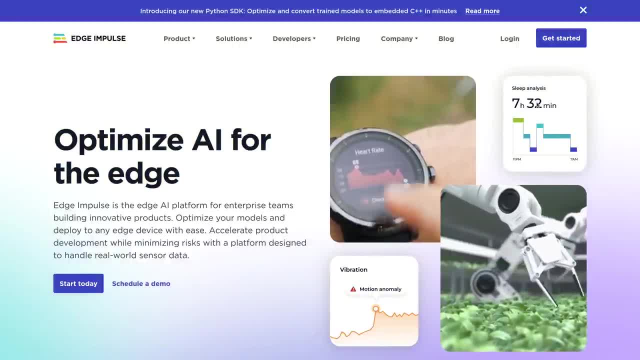 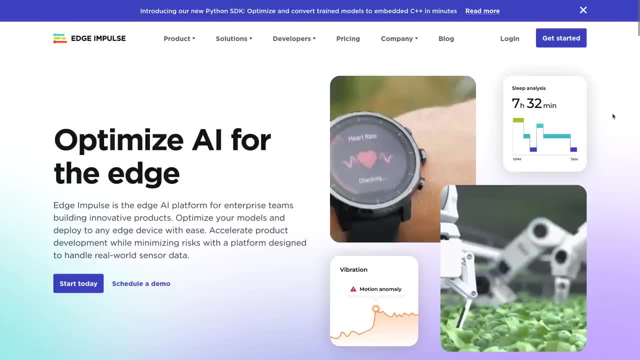 Now, of course, the first step in working with Edge Impulse is to go to their site and create an account, and that's what I'm going to do here right now. I've gone to edgeimpulsecom, where they show you a number of different features of the product. 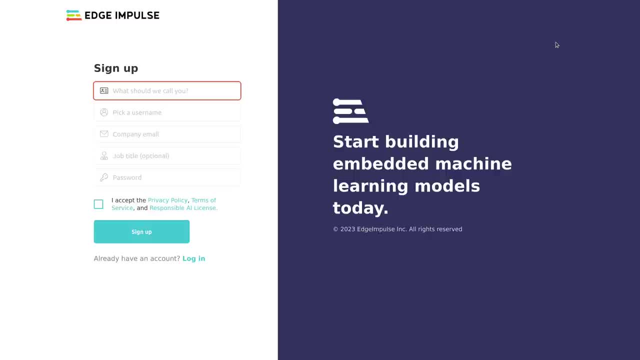 and I just click the Get Started button. And after clicking the Get Started button I open up another window where I have to give a bit of information. What should we call you? That's basically what is your first name. You pick a username. You'll need to put your email in there. 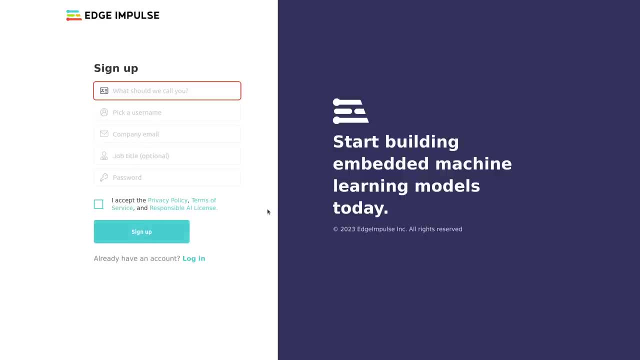 and a password. accept the agreement and hit the Sign Up button. You'll get a confirmation message in your email. Click on the link in that and you're all set to start using Edge Impulse Now. when you log into your Edge Impulse account for the first time, 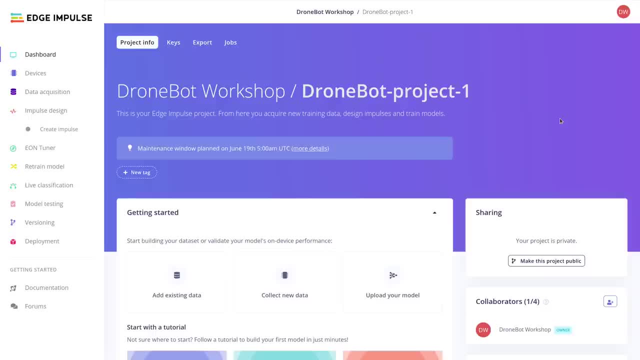 you'll be presented with a pop-up window that offers to run a wizard in order for you to do some data acquisition. I would suggest just closing that, because we're going to do everything manually, and when you close it, you'll arrive at a screen very similar to this: 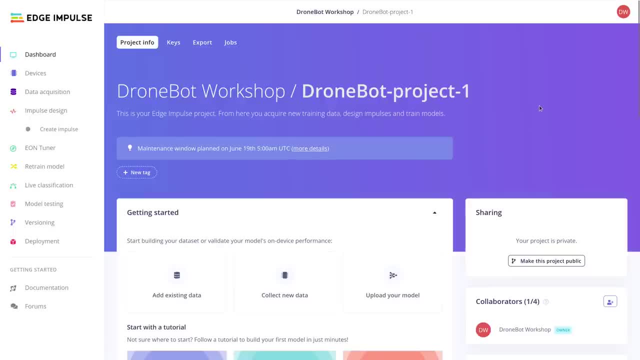 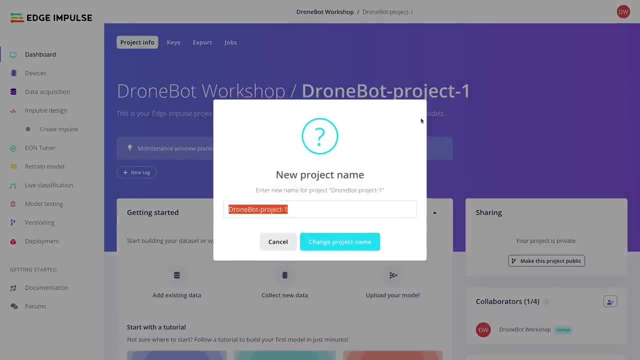 You are actually in your first project. It creates your first project for you and it gives it a name. In my case, it gave it DroneBot Project 1, but I can click on that to edit it and I can give it a different name if I wish. 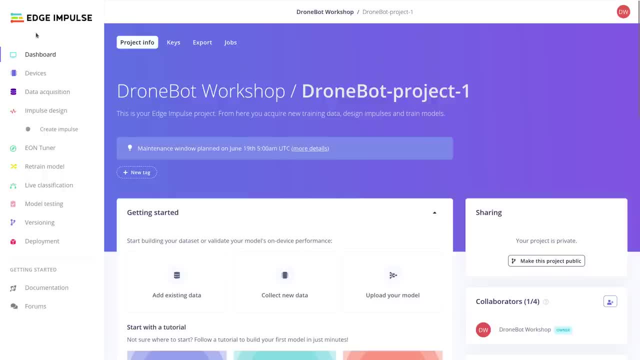 I'm going to just keep that for now. Now, down the side over here, you'll see a number of different menu items. Some of them won't make a lot of sense to you at the moment, but that's okay, We will be covering them. 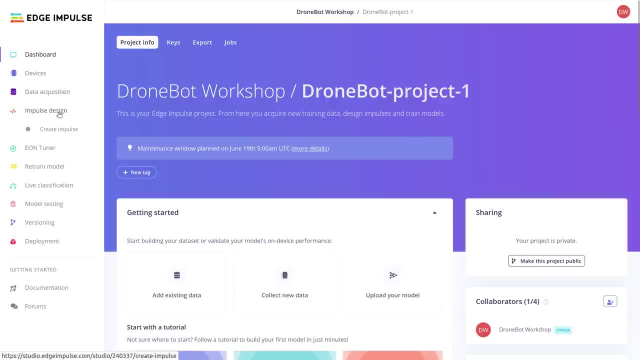 Data acquisition and impulse design are the two areas that we're going to spend the most time in, And up here in the corner you can go and change some of the aspects of your account. You can give yourself an avatar, change your account name. 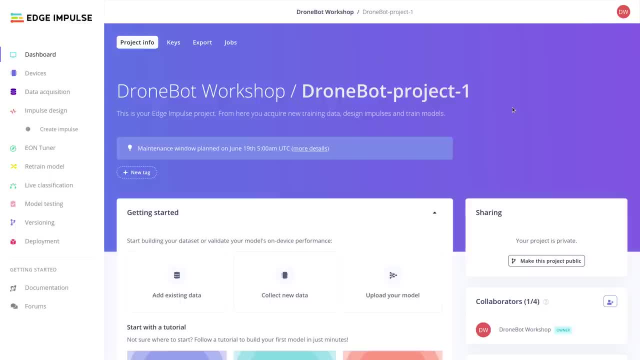 et cetera, et cetera. Now, this may seem a bit overwhelming, but it actually is pretty simple to use, And I think, in order to understand how to use it the best, we really need to look at the workflow that we're going to be using with Edge Impulse. 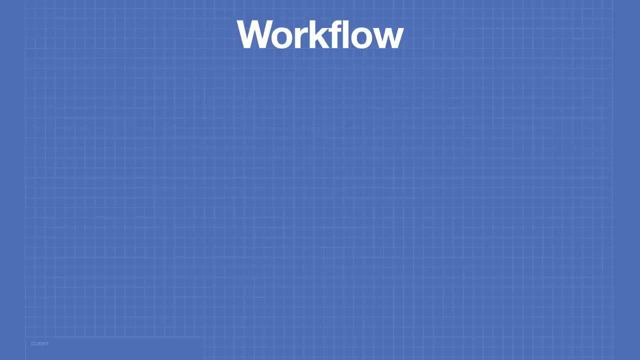 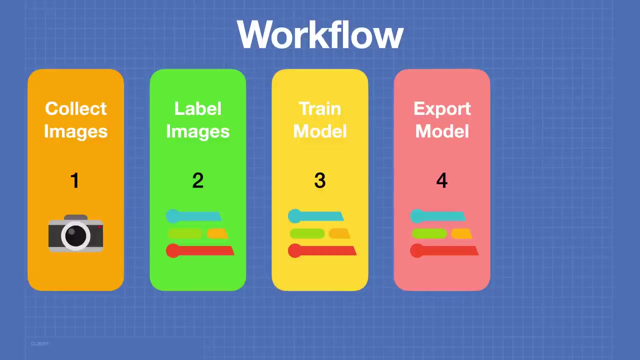 Now our workflow is going to consist of five different steps. The first step will be to collect the images of our object. The second step will be to label those images. Our third step is to train a model using those images. The fourth step is to export that model into code that we can use. 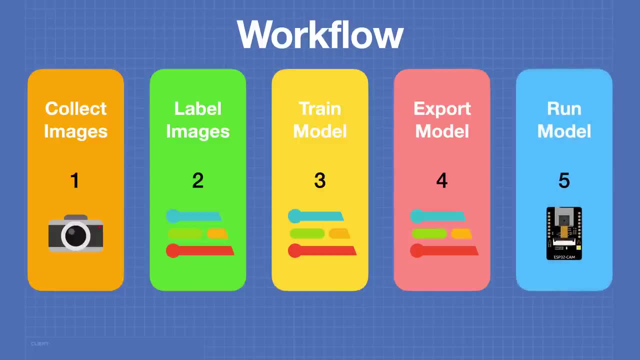 And, of course, the fifth step is to actually run the code on our ESP32.. Note that we'll be using Edge Impulse for steps two, three and four, and we can even use it for step one as well. In our first step, we're going to collect images. 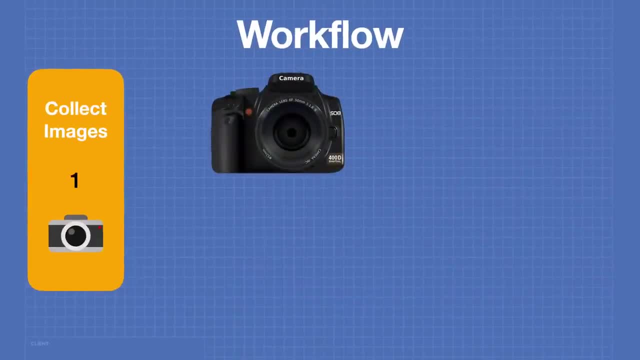 and there are many methods we could employ to do this. We could, of course, use a camera or some existing images in an image bank. A great method of collecting images is to use a webcam. A really easy method of doing it would be to use your phone. 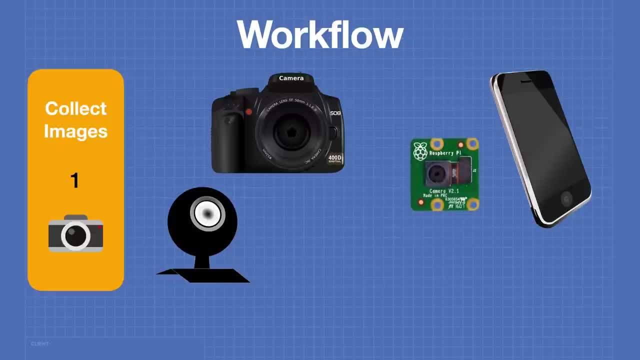 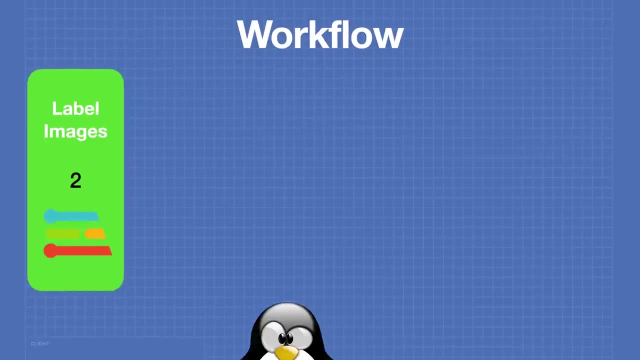 You could also use the camera on a Raspberry Pi or a single-board computer And, of course, you can also use the ESP32 cam itself. Today, I'll be showing you how to use both the ESP32 cam and the webcam. Now the second step is to label the images. 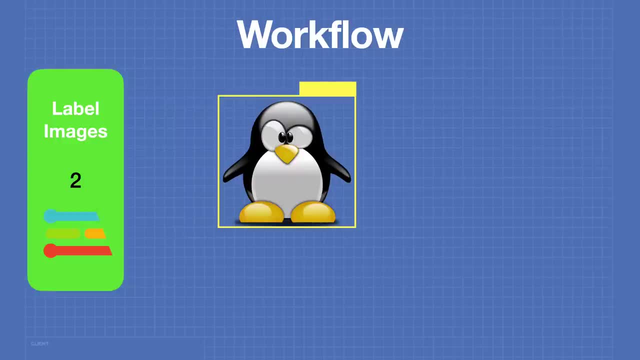 and we'll be using Edge Impulse to draw bounding boxes around the images and to give them a label. This, admittedly, is the most time-consuming step, but the more of this that you can do and the more accurately that you can do it. 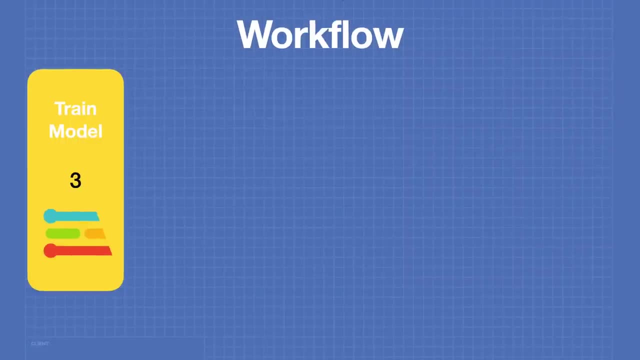 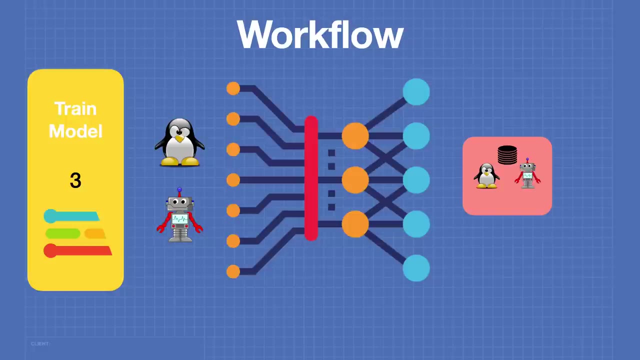 the better results you're going to achieve. In step three, we'll take the images that we collected and use them to train a model. We can run tests on our model to determine how accurate it is. Once we're happy with our model, we can export it. 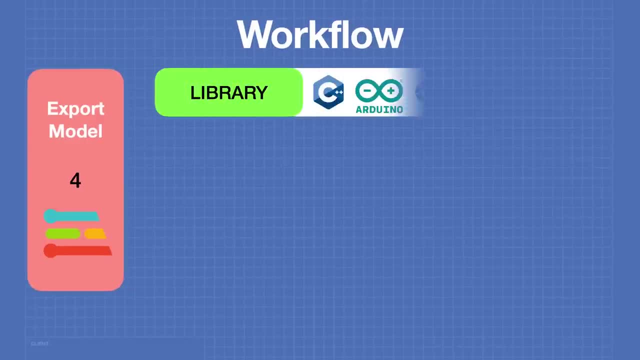 and we have a number of options here. We can export it to a code library, and this includes an Arduino library that we could use with our ESP32 cam. We can also export the model as firmware for a number of popular microcontroller boards. 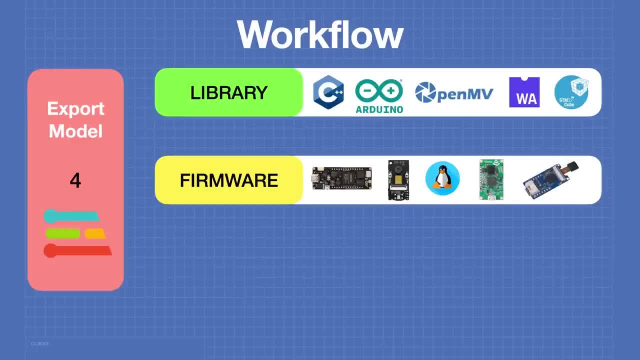 including the ESPI board. It can also be exported as Linux firmware for a number of different single-board computers. We can also use hardware to test and work with our model, and in this case we don't need to export anything at all. 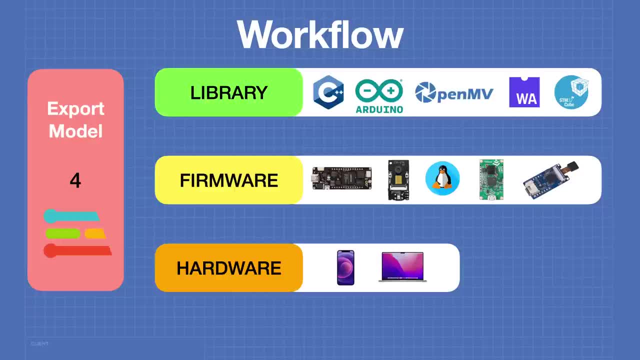 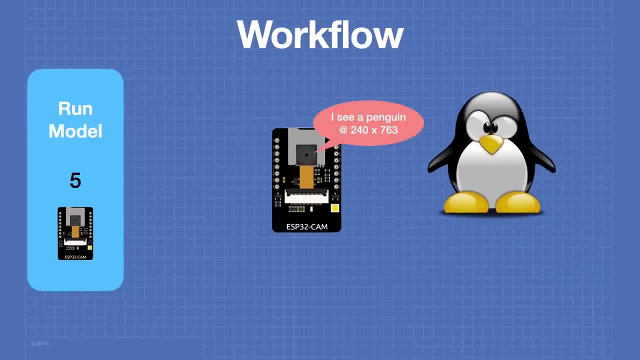 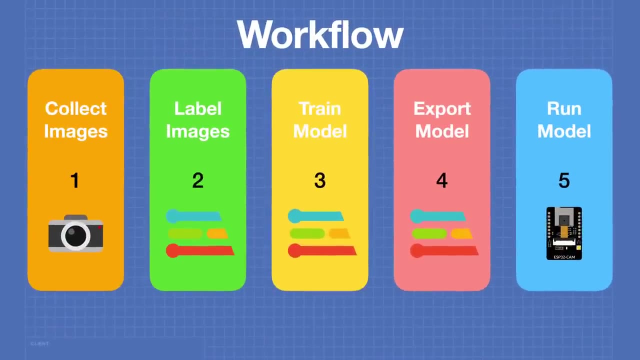 It can just be used directly on your phone or on your computer And finally, we can export our model to our ESP32 cam and test it out. So keep this workflow in mind while we begin by collecting some images of our object for our ESP32 cam project. 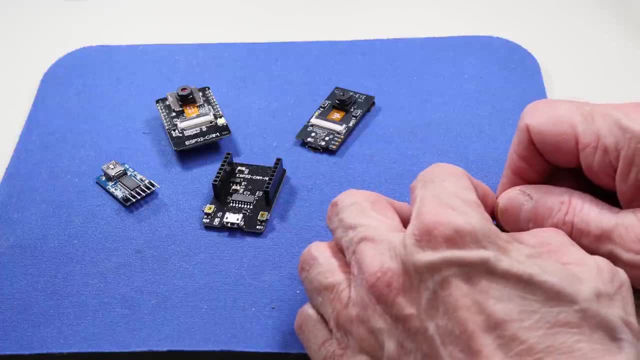 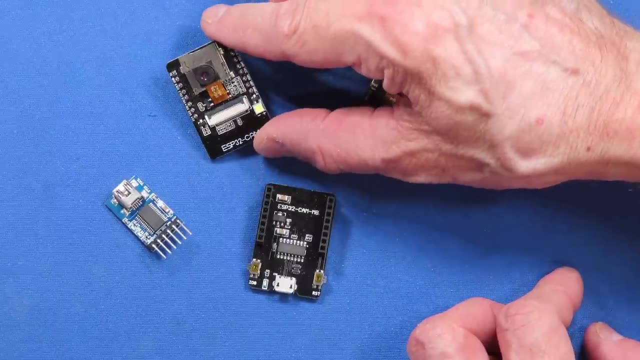 Now here's a quick look at the cameras that we could be using for our experiment today, And, of course, the classic one is this: the ESP32 cam board. This is the $9 camera board with the ESP32 cam. It also has a micro SD slot. 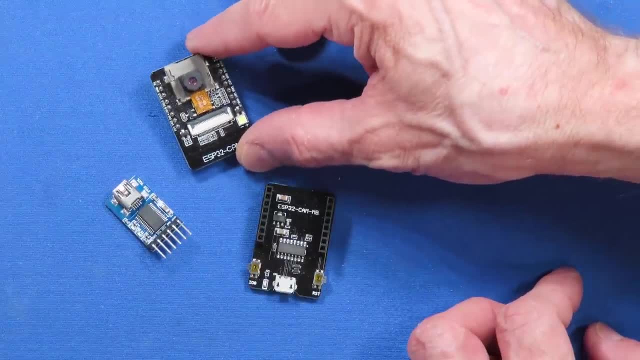 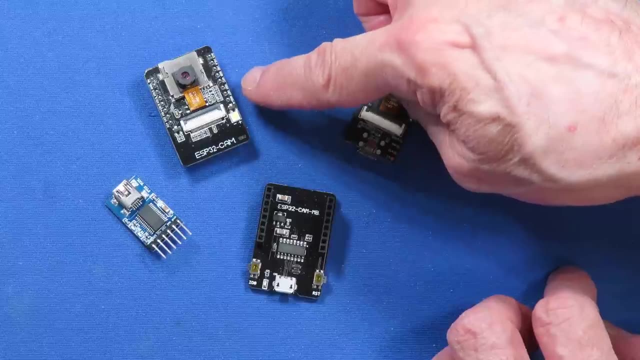 And we've used these in a number of different projects. Now, if you've used it before, you will know that there is no USB connector on this, And so you're going to need to have a method of programming this board, And the most common method is something called an FTDI adapter. 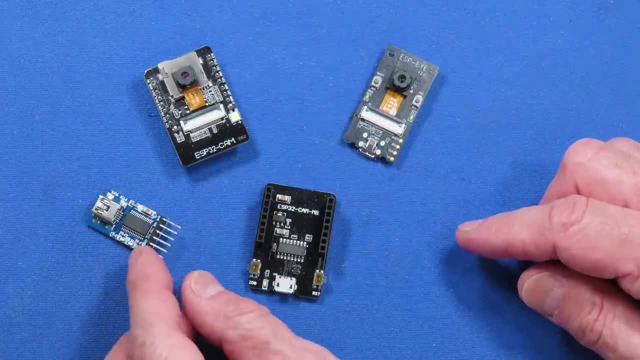 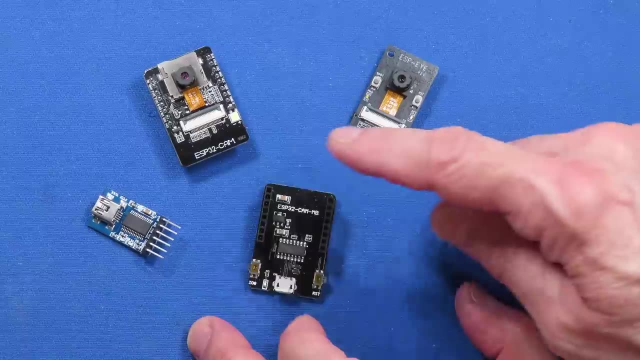 I've got one over here And you can use this with the ESP32 cam. I'm not going to show you how to do that today. I've already shown you that in the video and article I did about the ESP32 cam, So you can use that. 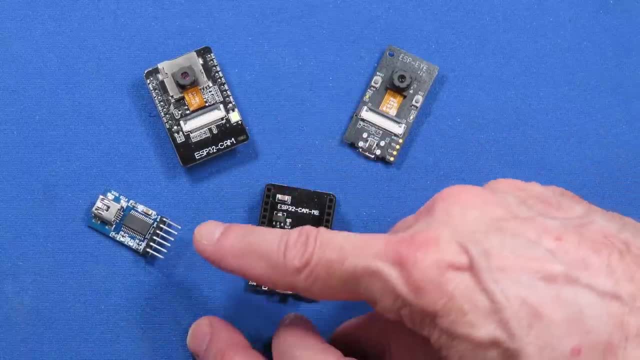 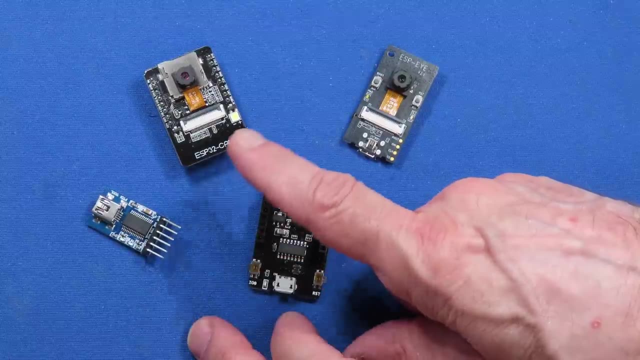 So you can check that out. if you need to know how to hook that up for programming purposes, There's also a jumper you're going to have to use to GPIO pin 0. You're going to need to ground it during the programming process. 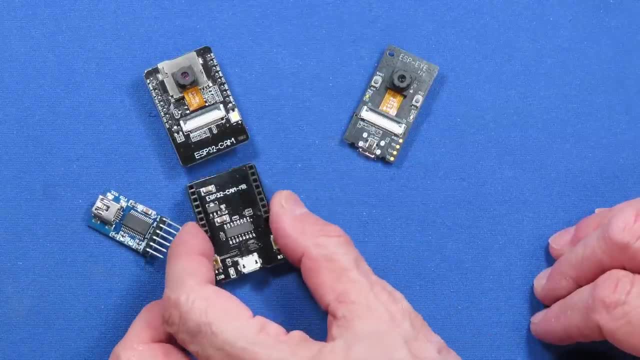 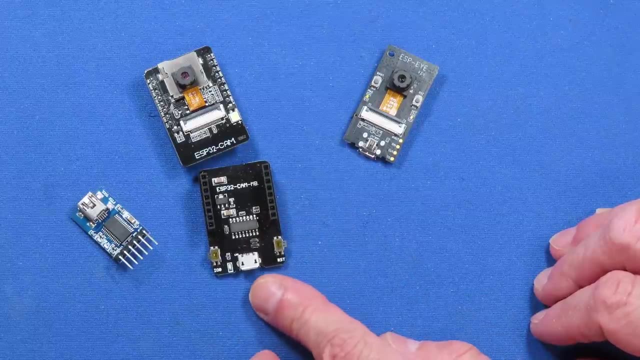 An easier way to work with it is to use one of these boards, And this is just a board that accepts the ESP32 cam board directly and provides a micro USB connector and a couple of switches as well, that you can use for boot and IO. 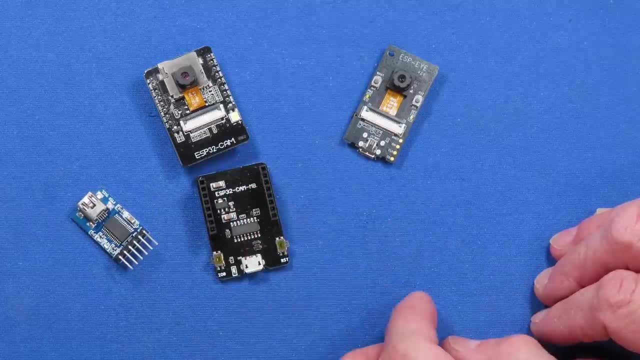 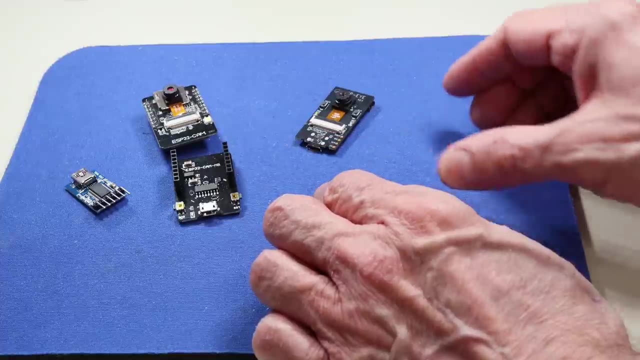 And you can often get these boards with the ESP32 cam board on Amazon or on eBay, So I'd advise you check it out if you're going to go that route. Another route you can go is this board, And this is a board by Expressive themselves. 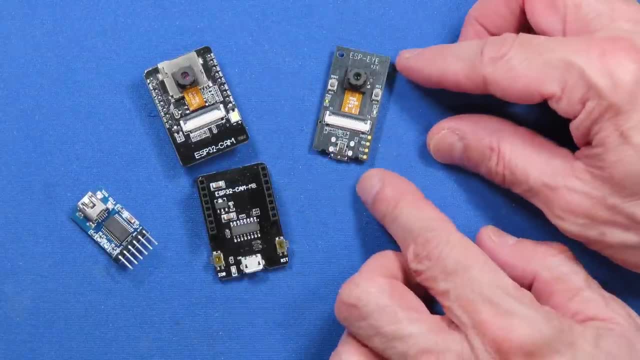 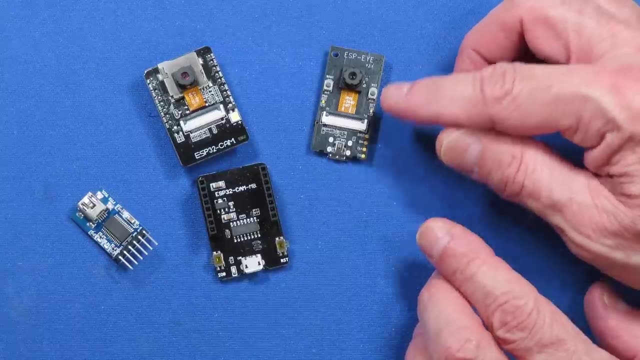 And this is a very nice board. It's called the ESPI board And it's got the camera on it. It also has a MEMS microphone And, remember, Edge Impulse can also work with audio data. So in your future experiments, 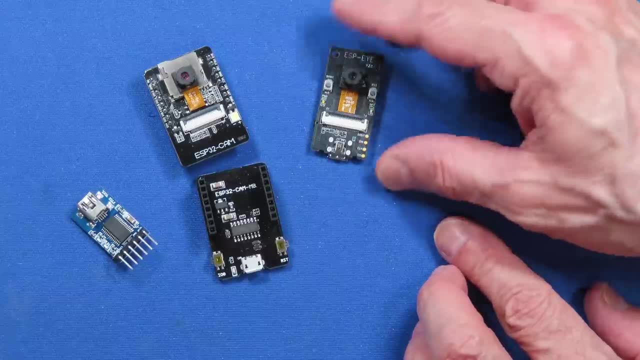 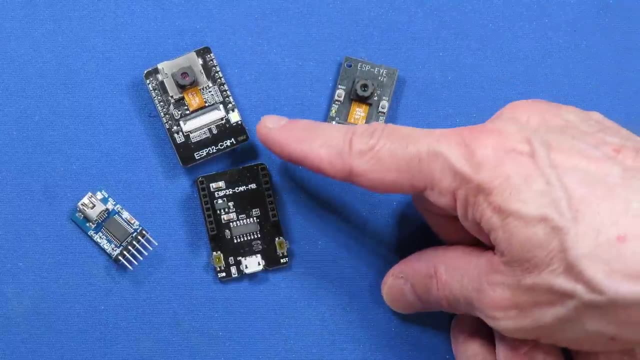 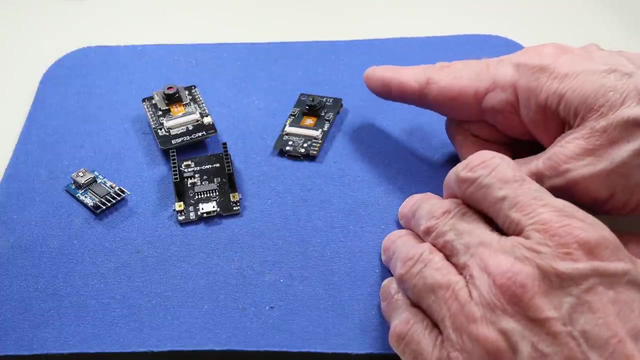 you could also add voice recognition into the picture, And it's got a built-in micro USB connector on it already, And so it's a lot easier to work with than the ESP32 cam board raw, And so either this board and this adapter or the ESPI would be my recommendation. 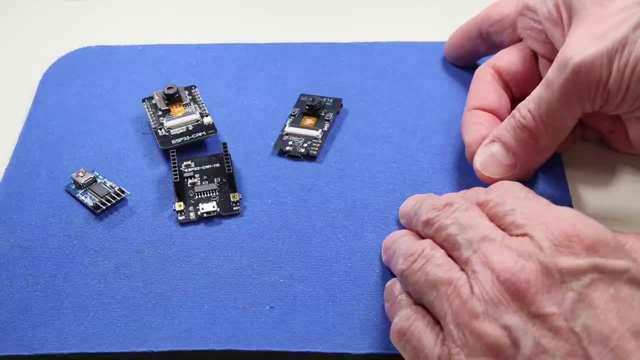 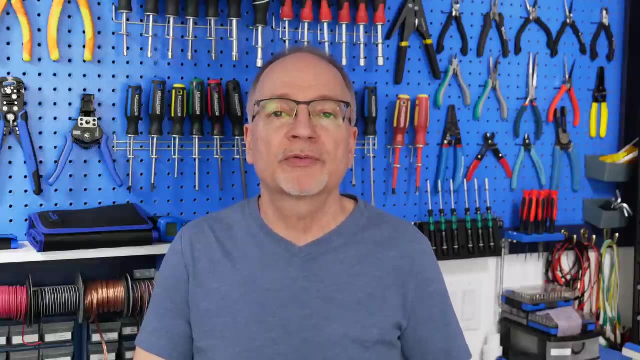 for a camera to use for the experiments that we're going to be doing today. Okay, now that we're all set up, we can begin by capturing some images And, as I showed you in the workflow outline, there are many different methods we can use. 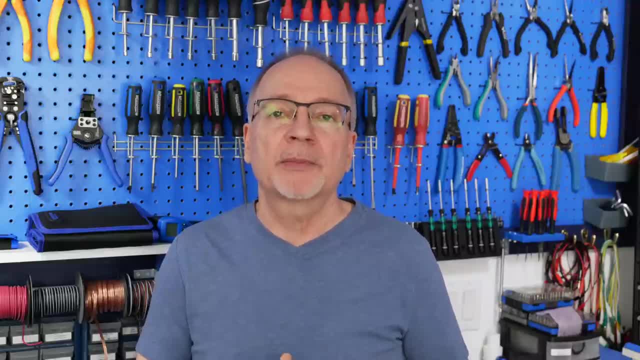 to take images of the object we want to detect. The method I'm going to be using right now is to use a webcam, So let me show you how I've got my webcam set up and we'll start taking some images of some objects for our model. 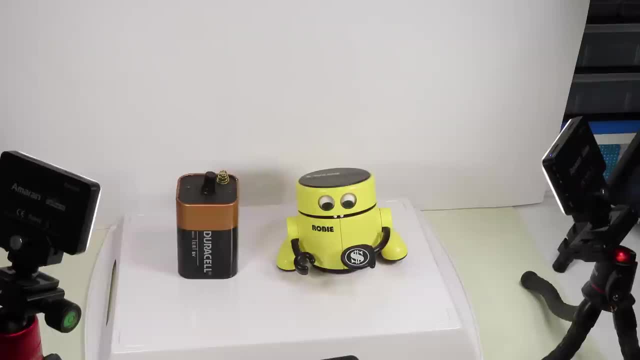 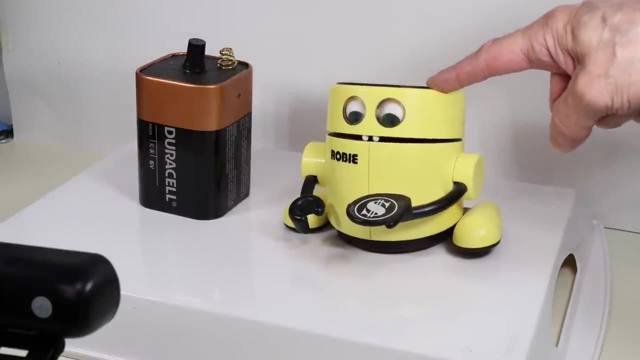 Now here's the setup that I'm going to be using to take the photographs, to train my models, And these are the two objects I'm going to be photographing. I've got a lantern battery over here, And over here we've got Robbie the Robot. 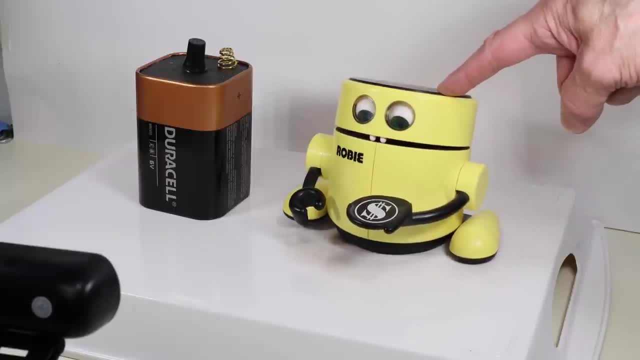 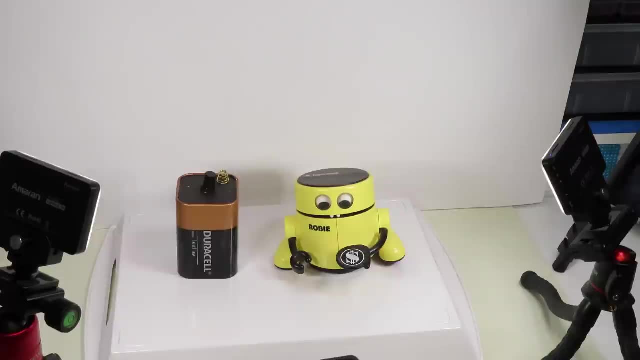 This is a Radio Shack piggy bank robot that I purchased way back in 1975. And he's going to be my second object. I'm going to be taking the photographs using a webcam, And this is the webcam that I got. It's a relatively inexpensive webcam. 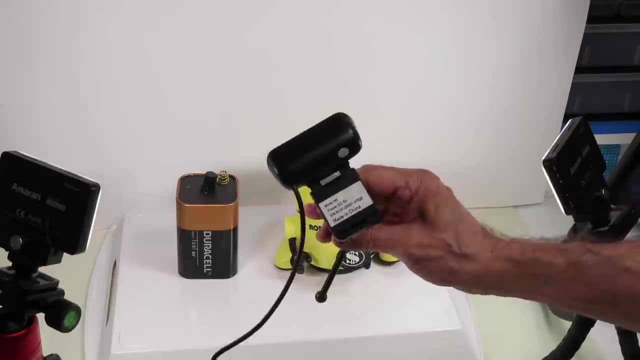 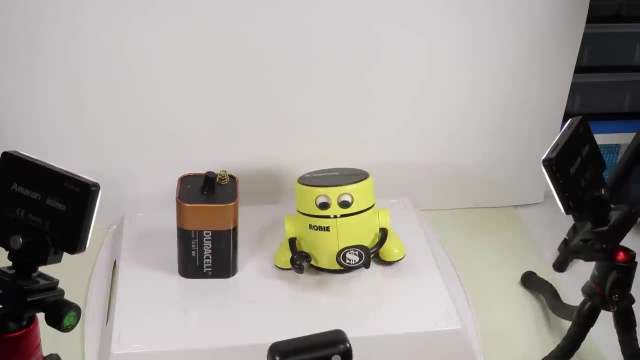 that I picked up on Amazon. The reason I picked up this webcam is, as you can see, it's got a tripod on it. It's got a quarter inch mount, so you can mount it on any photographic tripod. I thought that would be pretty handy. 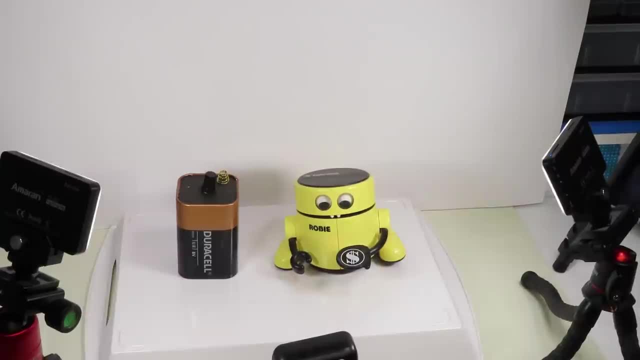 But of course you can use any webcam that you happen to have. You could also use the camera that's built into a notebook computer, if you can come up with an arrangement to keep the lid steady so that it's always in the same position. Now I've also added a couple. 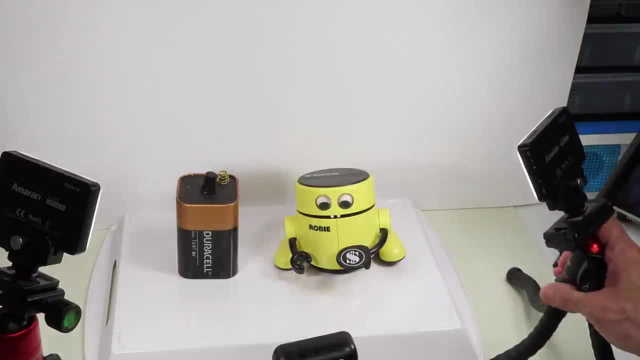 of video lights over here. I've got a couple small video lights And this is just to give consistent lighting on my objects. There's also another light that you can't see. that's up on the ceiling of the workshop that I use for video photography. 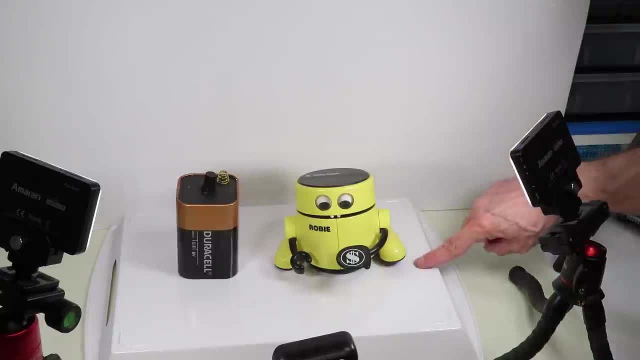 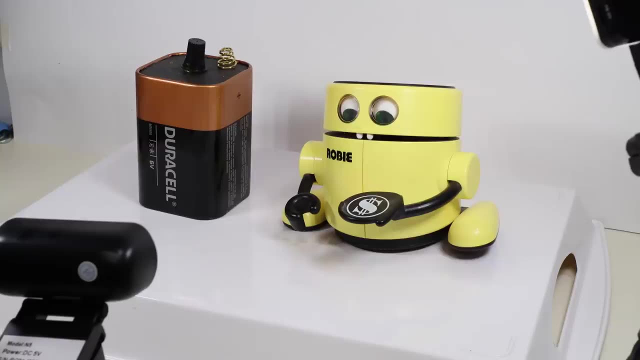 And it's on as well, And I've put a white background over here just to eliminate any other distractions so that we can just train ourselves on the objects. So now that you've seen my setup, let's go and start to work with it. 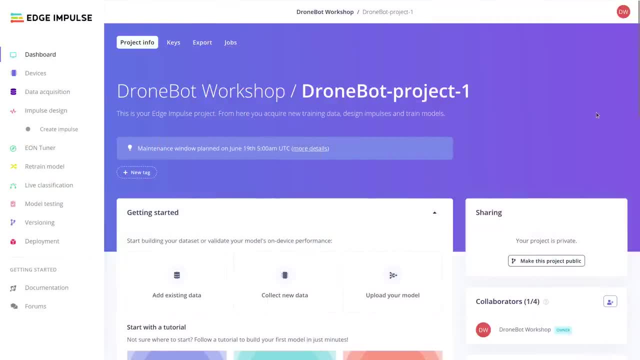 So, now that we're set up with the webcam, it's time to use it to collect some data, And so I'm back in the project on Edge Impulse, and there are a couple of ways I can do this. There is a data acquisition item. 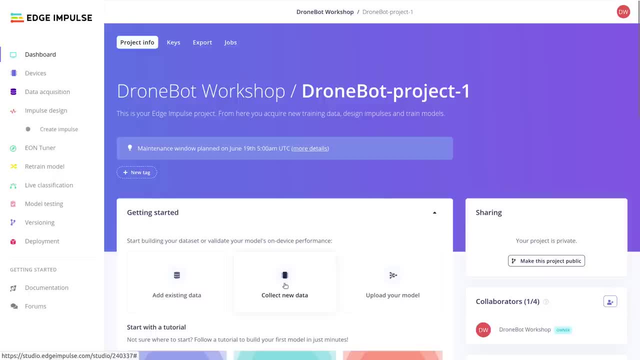 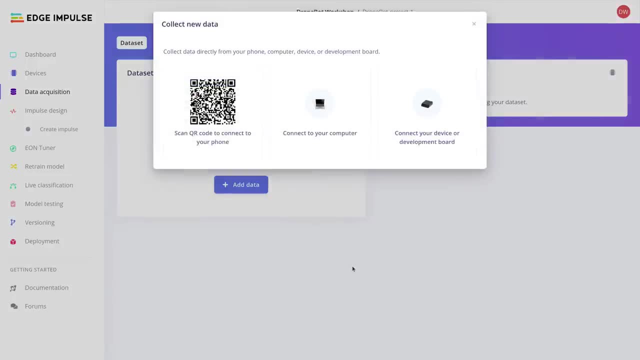 on the menu on the side, But the easiest way is to go and collect new data from this box over here And I'll click on that and it brings up a pop-up And I can see the methods I can use to collect the data. 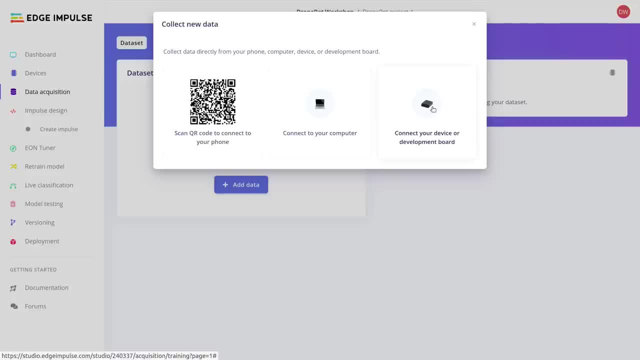 I can use my phone and they have a QR code that you can scan. You can connect the device directly to Edge Impulse, to your computer with Edge Impulse and start using it, Or you can just connect directly to your computer and use its webcam. 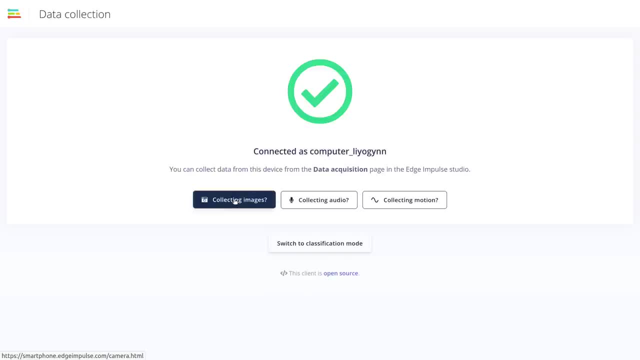 And that's what I'm going to be doing now. So I'm going to be connected to the computer here. I want to collect images. I need permission to use the webcam, So I'm going to click on that And let the webcam set itself up. 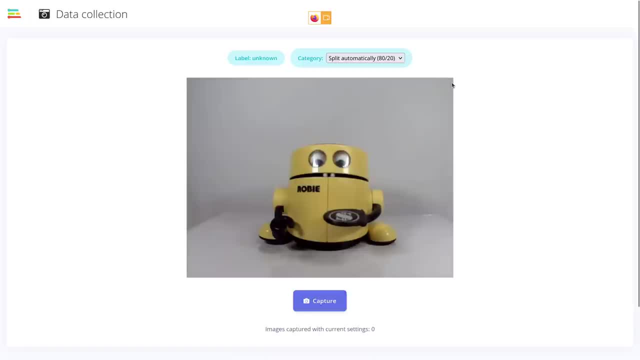 It's got some auto settings that seem to be adjusting itself, But right now you can see that I've got Robbie in my image and I'm ready to start doing my captures. So now we're ready to capture some images of Robbie over here. 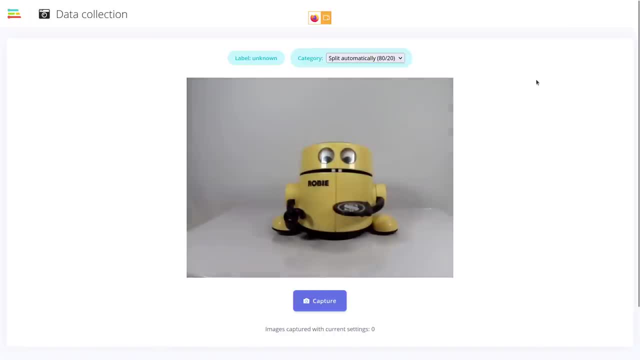 There's a couple of things at the top: The label and the category, And in category you have training data and testing data, And it automatically will split your data 80-20 between the two of them. For a label, though, we're going to have to give it a label. 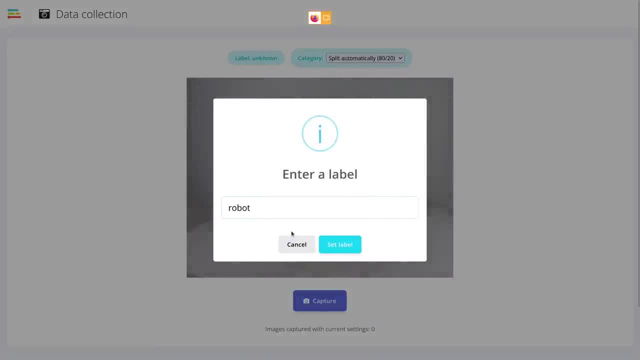 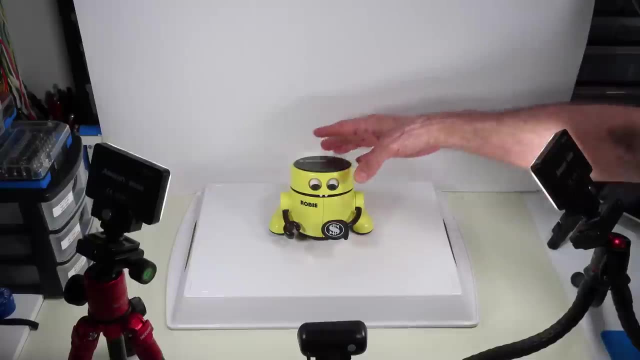 So let's give it a label. Right now it's unknown. I'm going to call him Robot And we'll capture a picture of it. And we'll capture another picture of it And we'll move Robbie around a little bit so we can give him. 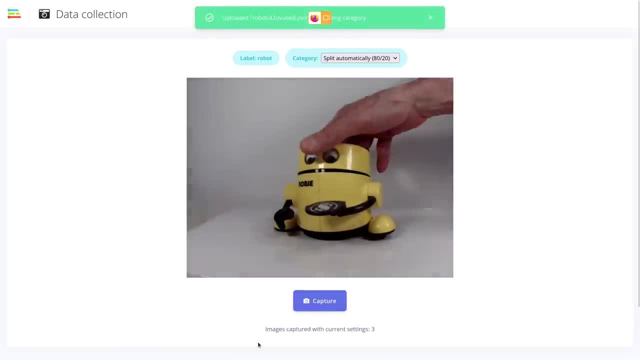 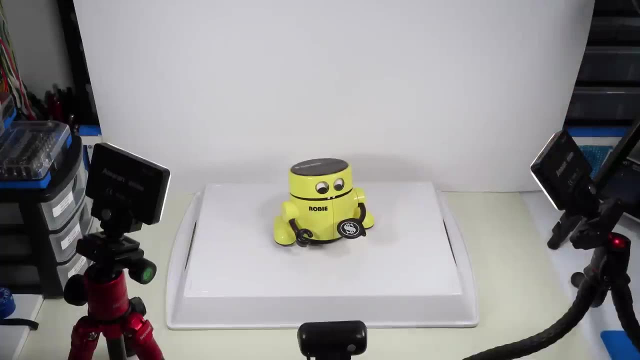 a couple of different angles. Capture another picture, Get a side view of him, Move him again. I think you're getting the idea. I want to take a number of images of Robbie and I want to take them using different angles and different shots. 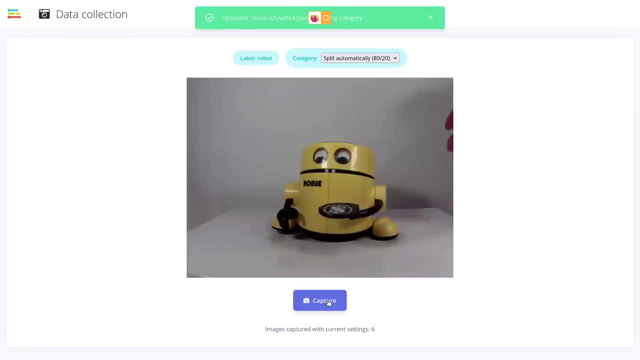 I'm going to move Robbie back and forth a bit as well. Get him closer to the camera at times, Get him further. I want it to get a lot of different images of Robbie that it can use for training. Now, of course, I'm not going to make you watch me. 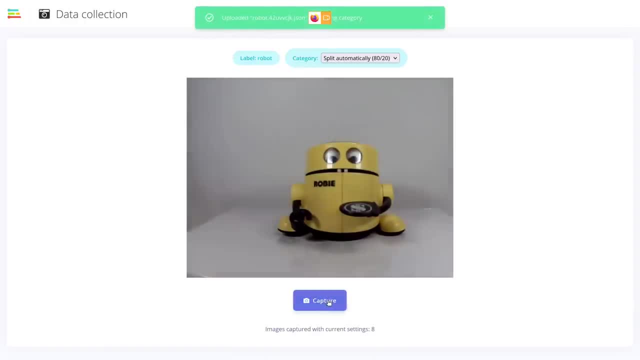 collect all these images. So I'm going to go and continue to collect some images And I'll meet you back here. So now I've taken 75 images of Robbie. You can see the count down over here And the more images you can take. 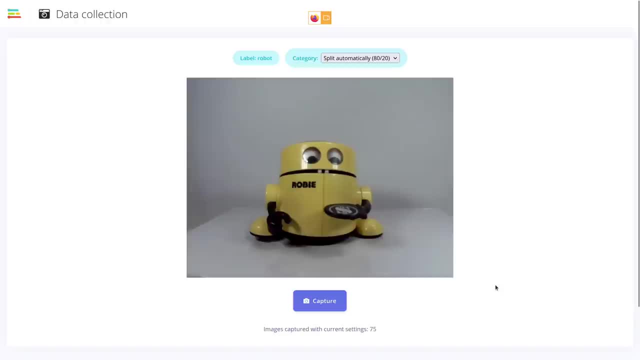 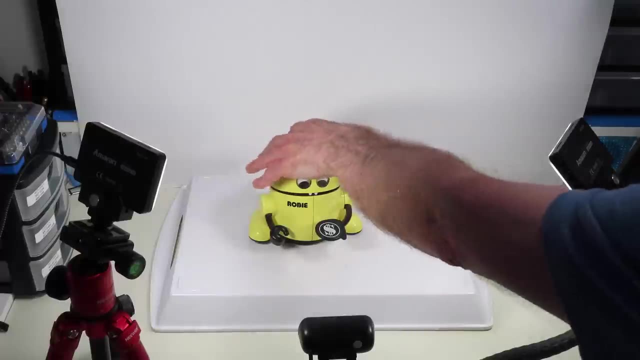 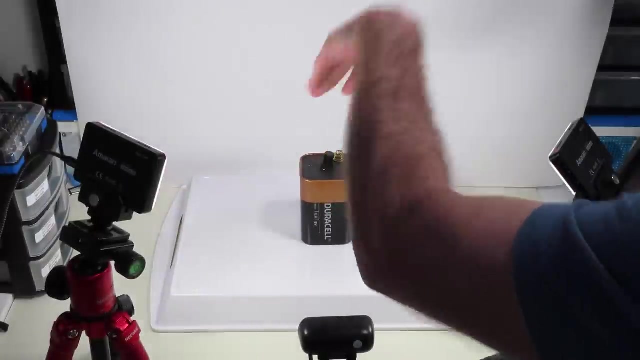 the more accurately you can train your model 75 should be a good amount, But I could have taken more. But I want to move on to my second object, which is the lantern battery. So let's take Robbie off the stage And replace him with this guy. 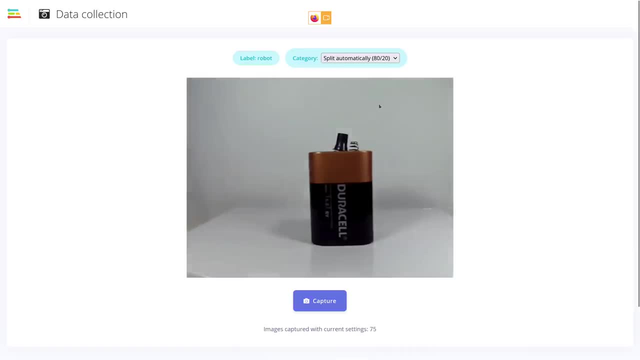 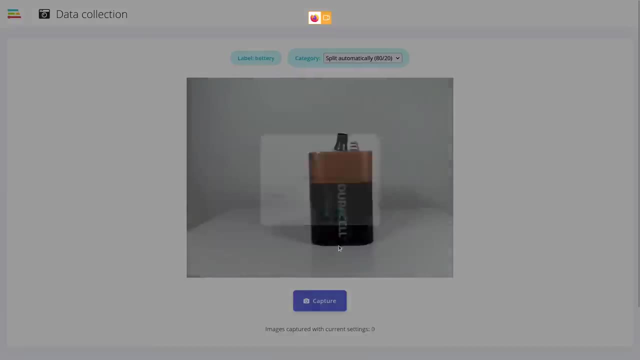 Now, before I hit capture, of course I've got to go up and do my labels. I've got to change my labels. So here I'm going to change the label And we'll set the label for that, And now I can start capturing my battery. 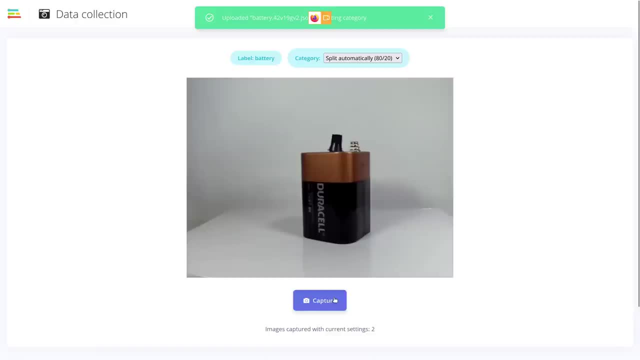 And it is, of course, the same procedure that I used when I was capturing the pictures of Robbie. I just move it around to different spots, different angles, and try to get a bunch of training data for it. So, again, I'm not going to make you. 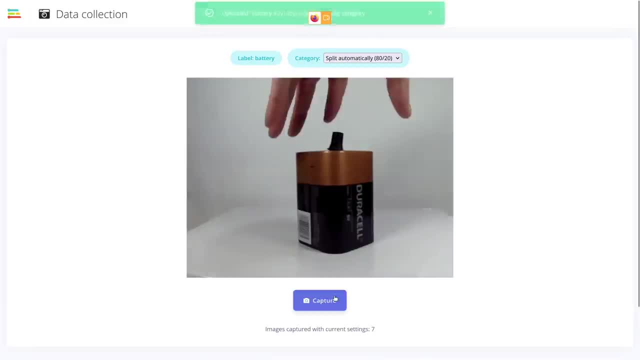 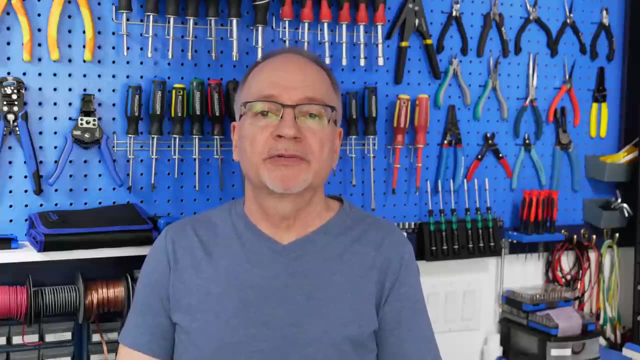 watch me do all of this. I'm just going to do it and gather some data And I'll show you the next step after that. Okay, now that you've captured a large bunch of images, we can move on with our workflow And the next steps in the workflow. 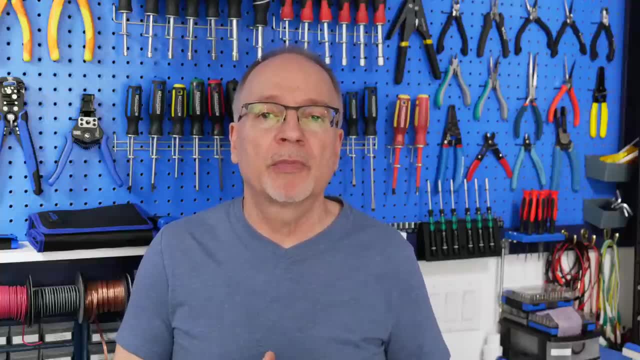 were to label our images, to train the model and then to deploy the model to a format that we could use with the ESP32. And we can do all of that within Edge Impulse. So let's start off by labeling the images that we've captured. 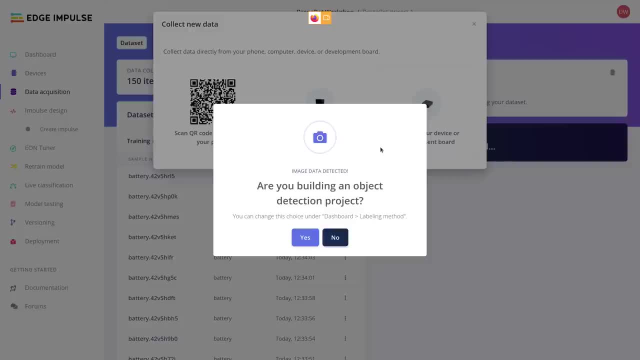 So I've got the images of both my objects. I've moved back to the main screen and I have a pop-up window here that asks me if I'm building an object detection project, And it sees that because it's already detected some images. 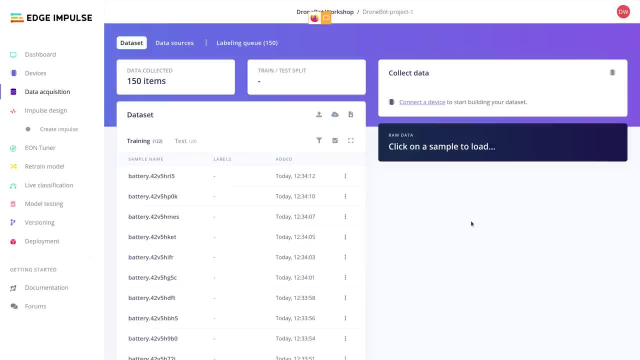 And obviously I am, so I'm going to say yes, After I clear everything. you can see the screen that I'm on right now with a list of all the different photos that I've got, And I can look at them over here if I wish. 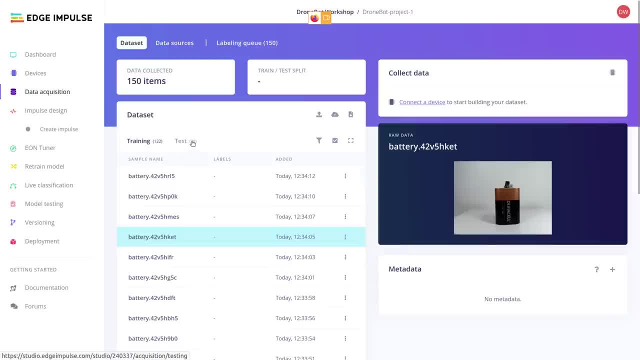 And, as it says, on this one, I have 122 training ones and 8 test ones. So now that I have 150 images, I'm going to need to label them. Yes, I'm going to need to go through 150 different images and label them. 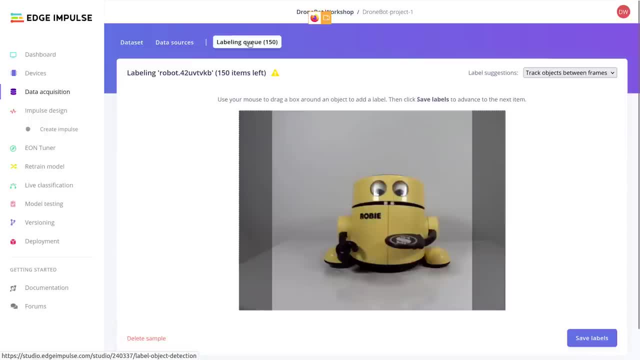 And let me show you how you do that. You go into the labeling queue and there are 150 objects queued in here right now And you can see I've got a number of lines over here when I'm moving my cursor. What I want to do is I just want to draw. 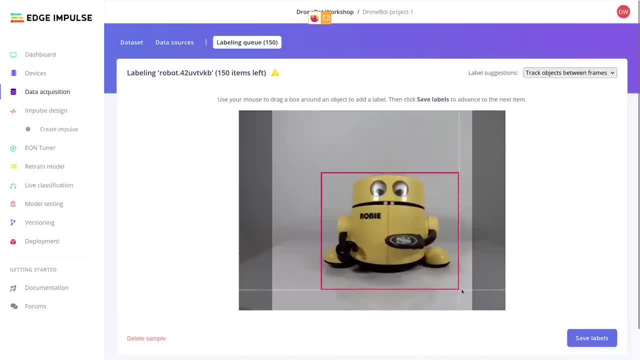 a bounding box around Robbie. So I'm going to go and press my mouse down and draw the little line into the box And if it asks for a label, I'm going to call him a robot And, as you can see, it says robot up in the top corner. 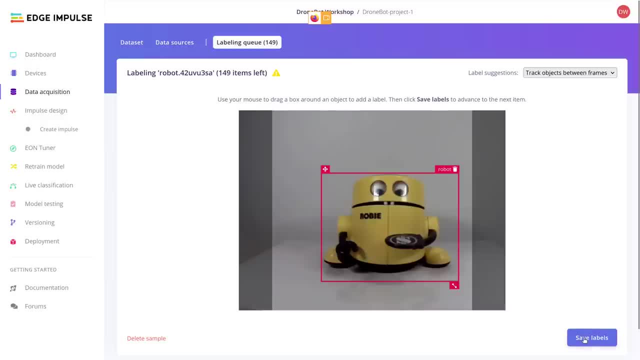 And I can save the label And it advances to the next item And you'll notice that it actually has already put a bounding box around that item and it's not too bad. And as I go through you'll see a few cases where it isn't bounding correctly. 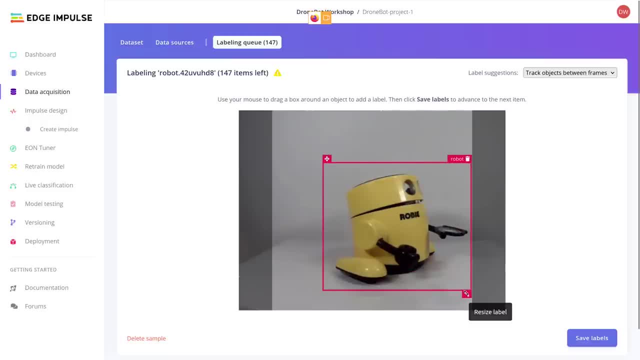 And what you can do is you can grab the box and you can resize it- and that indeed is Robbie- And as we hit save labels, it'll continue to advance And you can adjust that, And, of course, I'm going to have to go through this. 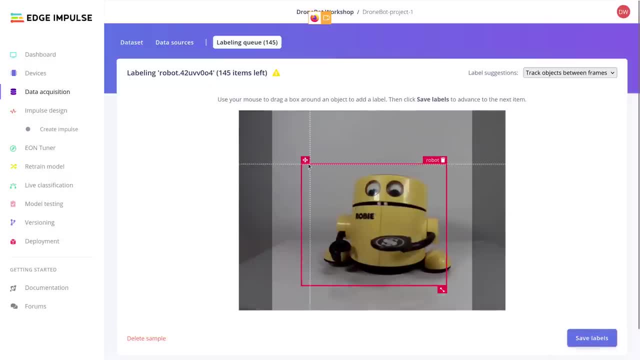 145 more times, And I don't think you want to watch me do that. So let me do that, and I'll meet you back after this. One thing I need to note, though, is that you will need to change the label when you come to the battery. 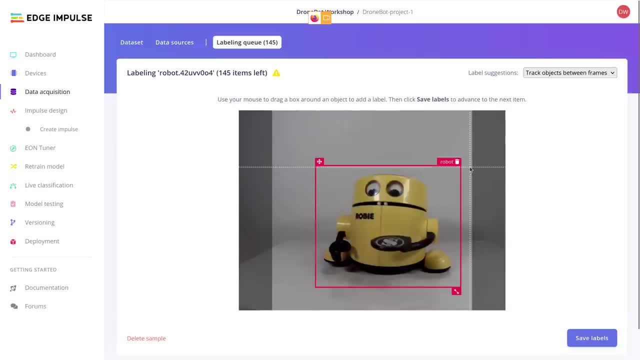 and re-label that one battery, And you'll do that just by clicking into the label thing here. You'll hit delete label and you'll do another save label and it'll give you a box to put the name battery into it. So I'll do all that and I'll see you after that. 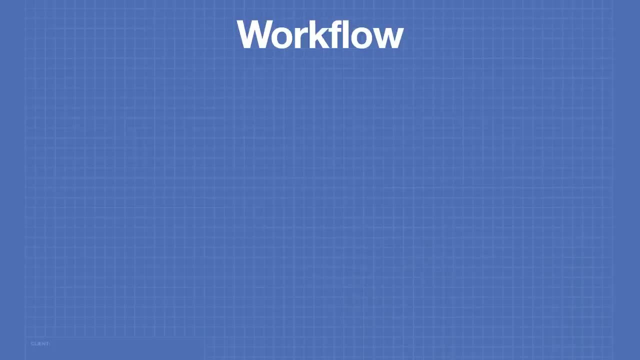 Now, before we move on, I think it's a good idea to take a look at the workflow diagram and see where we are in the process And, as you can see, we've done step number one, which is collecting our images, and done step number two as well. 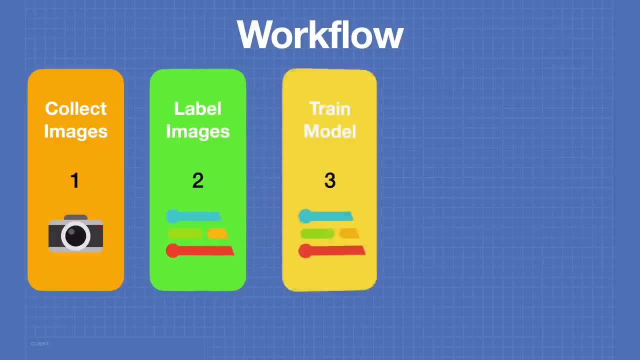 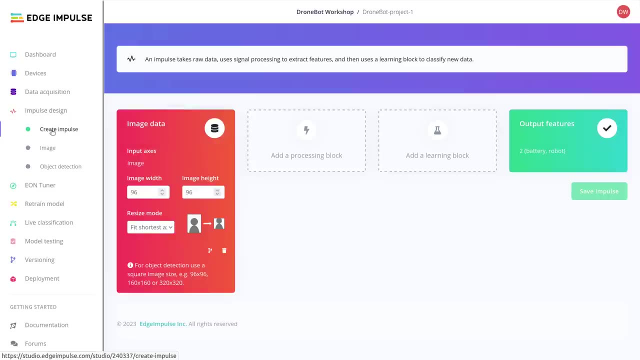 which is labeling the images. So now we're on the third step, which is to train the model, And where I've gone to in my screen is under impulse: design, create impulse. Now I have to confess I've been messing with this a little bit. 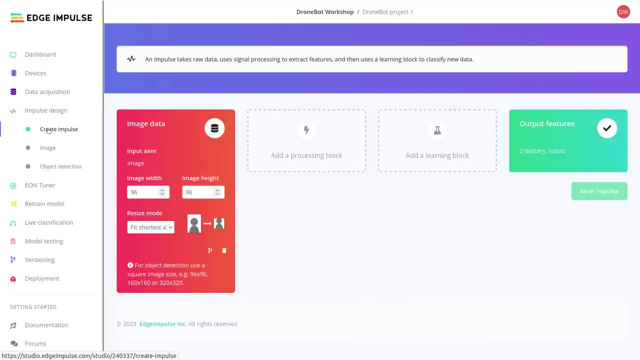 So on your screen you probably won't see the image and object detection items below it just yet, until we complete this step. But it's actually the same thing, so don't worry about it. Now, the first thing you'll note here is my image data is set to 96 by 96. 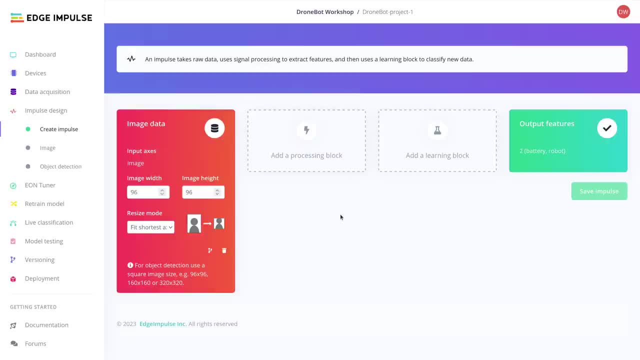 and while that might seem a little bit small, you actually want to create as small an image as possible, because that will mean less processing time on your ESP32.. In fact, if this doesn't work well for you, you could go through it again and train it as 48 by 48.. 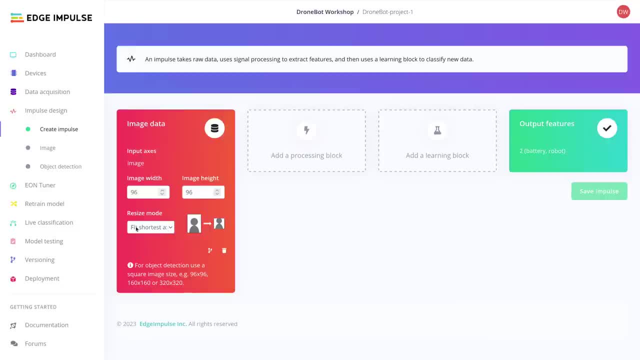 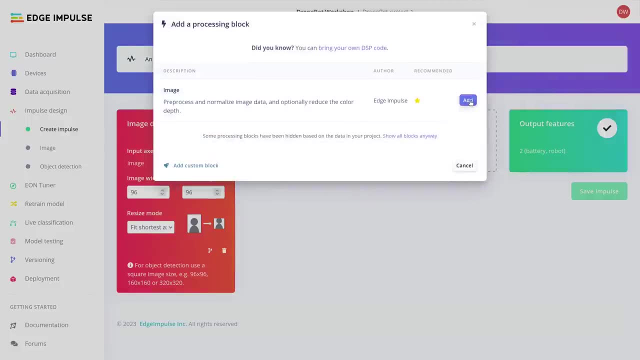 The resize mode will save this fit- shortest access- and we'll add a processing block, and the processing block we're going to add is the only one available to us- the image processing block- And we'll also add a learning block and the learning block will be: 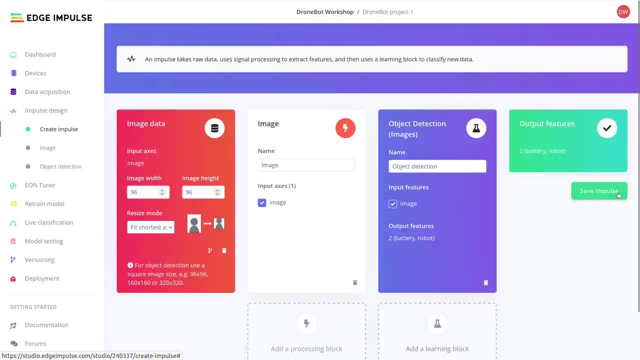 the object detection, the one on the top over here, And then we'll do save impulse And we've saved our impulse. And so now what we're going to do is go down into the image tag over here and we're going to do one thing over here: 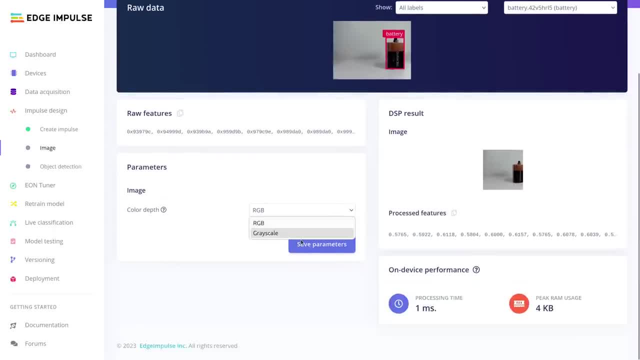 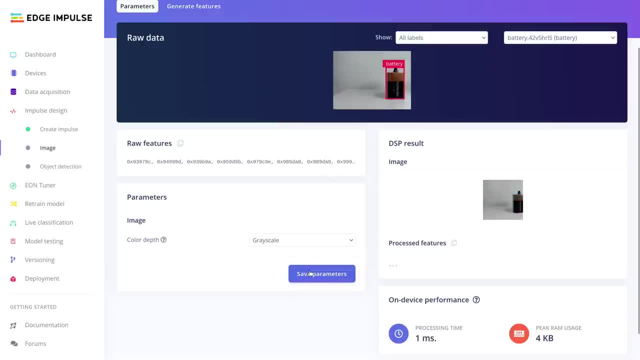 in the image tag We're going to set the color depth to grayscale. Again, this will be a lot easier for our ESP32 to process, And so we'll set that to save parameters. And then we're going to click on generate features. 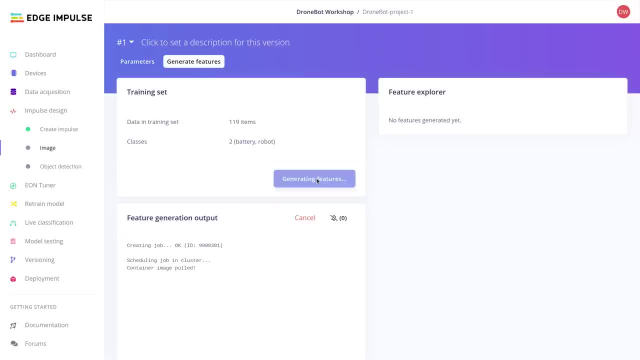 And this may take a moment or two, And now we've finished generating the features for the reference. that did take about two minutes on my machine And we actually have a pretty good diagram over here because we've got all of the samples for the robot in one section. 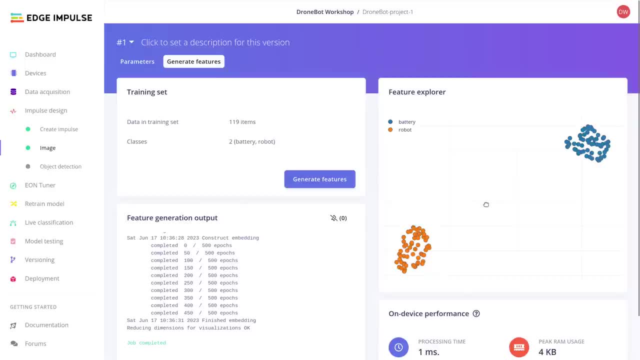 and all of the ones for the battery in another section. That's really a good sign, because if the two of these are mixed up in the feature explorer, you're bound to get a lot of errors, But right now it looks like we've got a pretty good one. You'll also 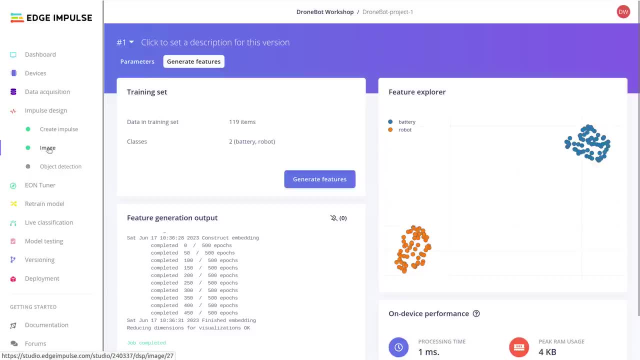 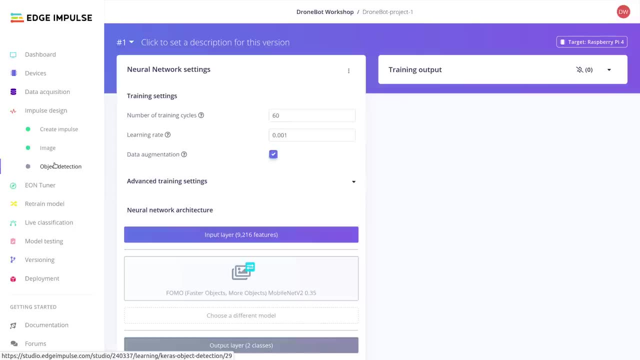 notice that now image on the side is a green light And we can go on to the next thing, which is the actual object detection. Now, on object detection, there are a few things that you might want to change over here. Now you might want to experiment. 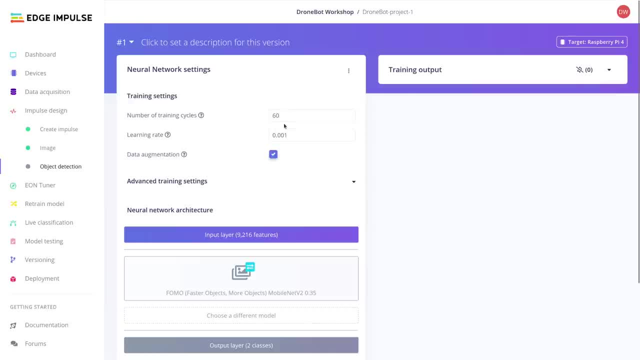 with these The number of training cycles and the learning rate, And the higher these numbers are, the larger it's going to take, The longer, excuse me, it's going to take to do this. What we actually want to do over here is: I'm going to leave these. 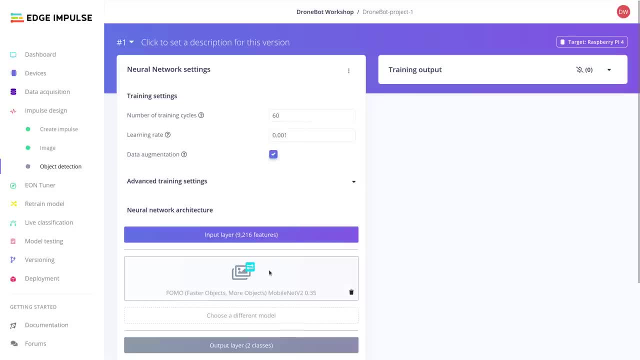 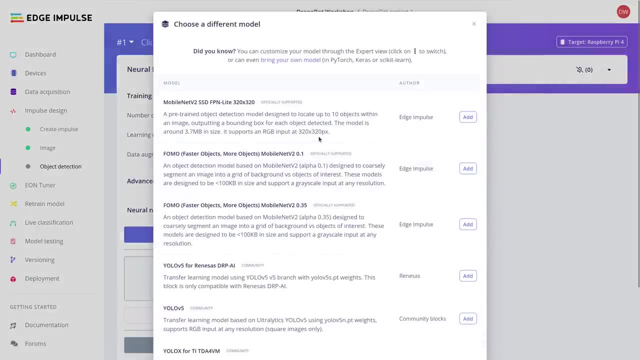 as they are, But we're going to go down and take a look. this over here, The model that we're using. We'll choose a different model And this is the one we're going to choose: Faster objects, more objects. mobile net version. 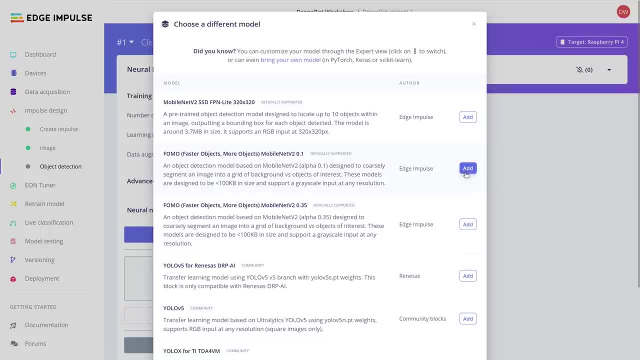 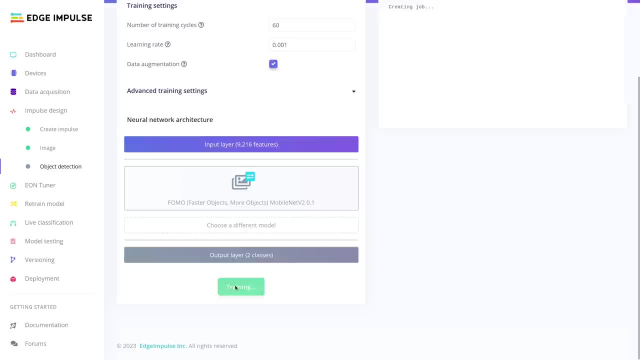 2.01.. And the reason we're going to choose this is it's the only one that will actually work with the ESP32.. And now we can just hit the start training button, And this is going to take a few moments as well. 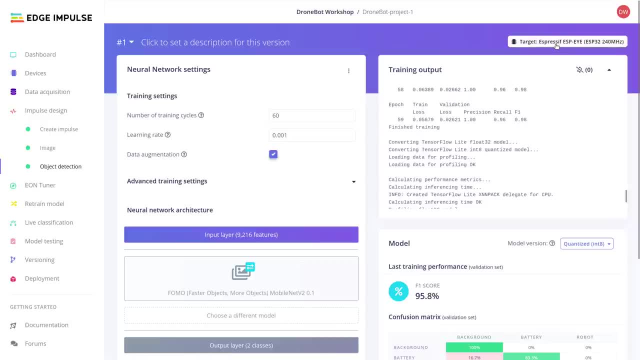 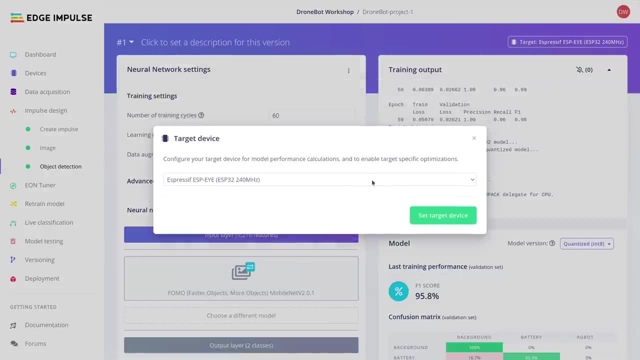 Okay, the training is finished and we've got the results over here. Now I wanted to show you something in the top over here. You may have noticed that this had previously said: RASP, Raspberry Pi 4.. You can change the target to anything you want, And I set 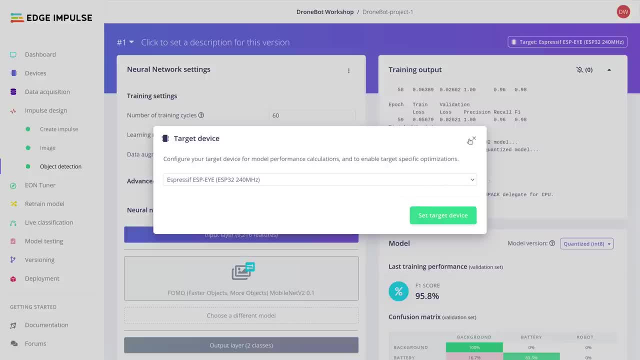 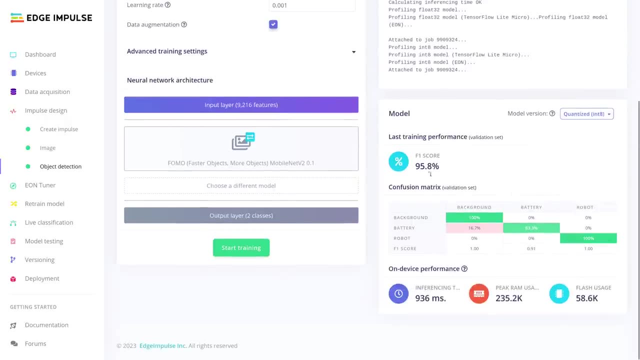 it to ESPI, which is the only ESP32 device they have here. Now what that does is this: gives you the specifications for how this is going to work on the ESPI, And it's good, but it's not perfect, It's not 100%. So this is 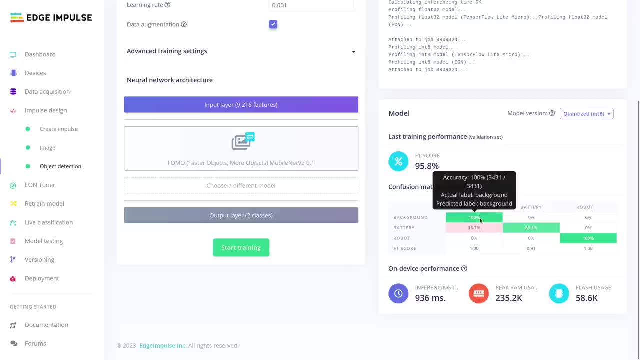 what's called a confusion matrix, And it looks like I might have some confusion between my battery and my background over here, And you can see that over here, That the battery is not being detected 100%, Whereas the robot seems to be just fine. So we can. 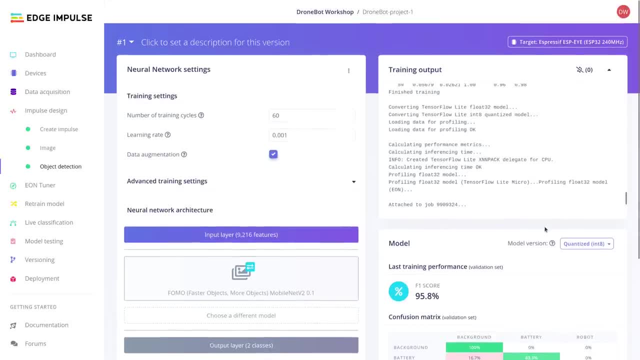 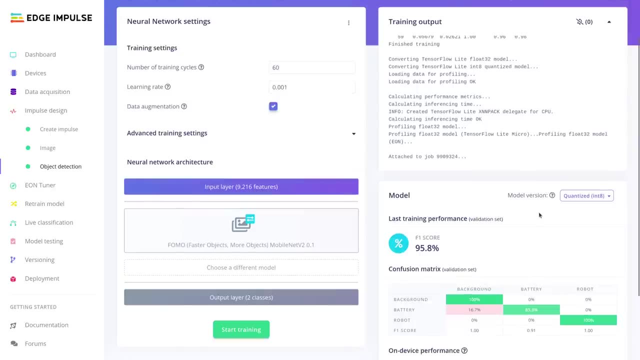 expect we might have a few flaky results with this, And the way to improve this, of course, is to go back, collect more images, put the bounding boxes as close as you can and run this through again. You can also experiment with changing these. 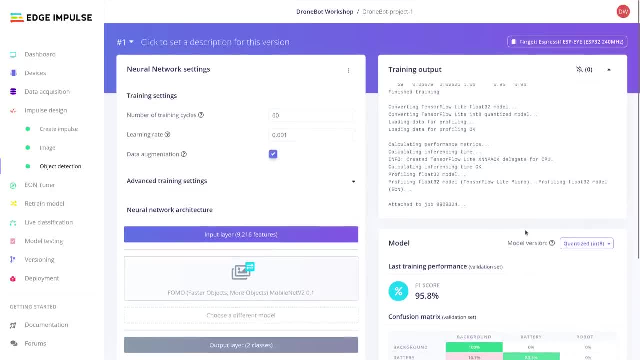 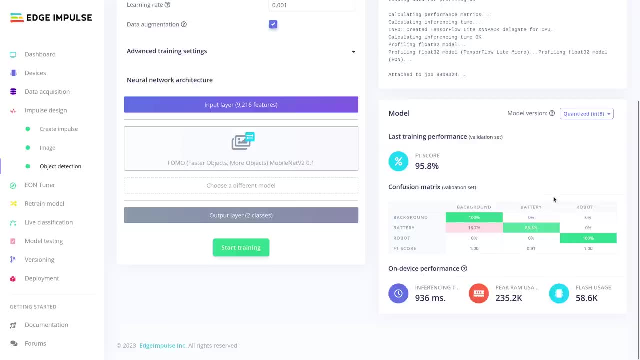 training cycles and learning rates, if you want to, To try to get these numbers better. But we're going to go with these ones anyway and see what the results are, Knowing fully well that we might have been able to do a better job. Now our next. 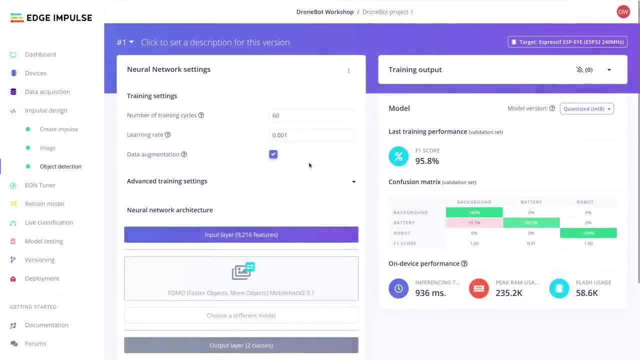 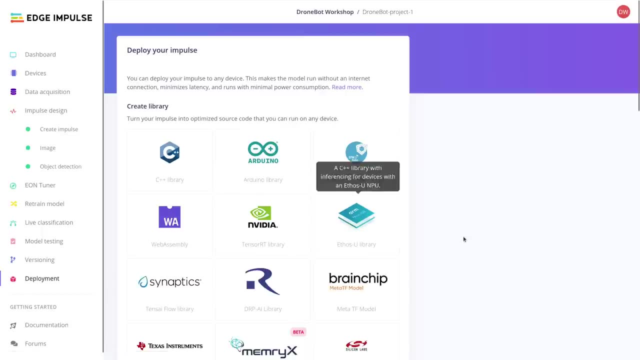 step is to export our model, and that's actually a pretty simple step over here. We're going to go down to the deployment tab over here And open that up And, as you can see, there's a number of places we can export the model to, But we 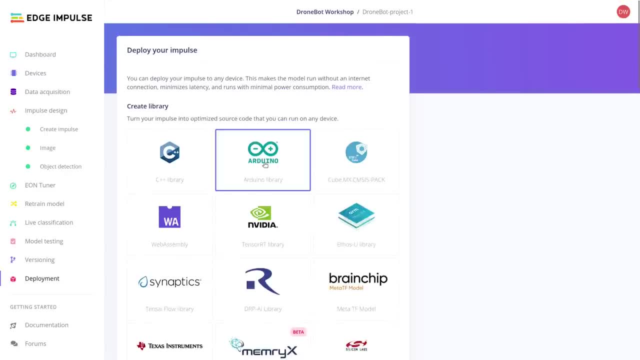 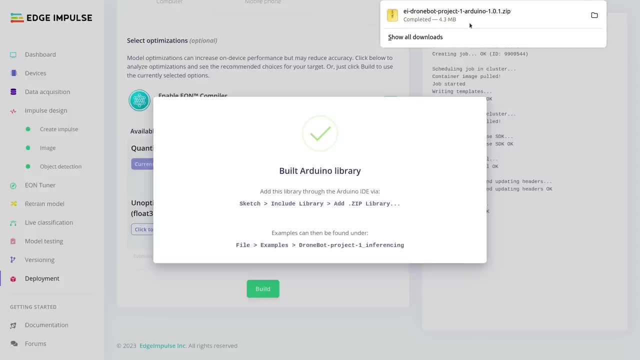 want to make an Arduino library, So we're going to click on this And we'll do a build. And it has built an Arduino library and it has also downloaded it to my PC in the form of a zip file And we are going to be able to use. 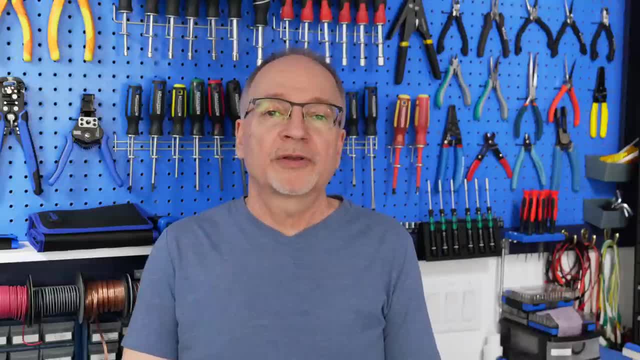 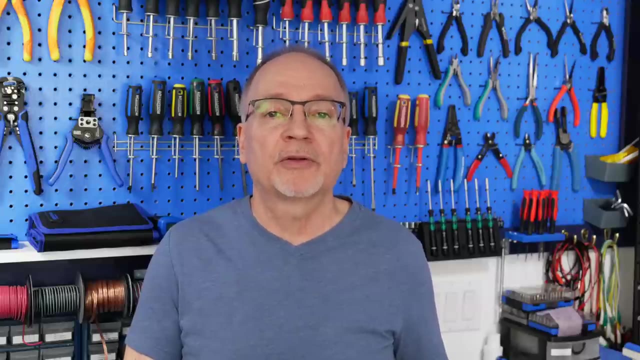 that with the Arduino IDE. Okay, so now we have a zip file which contains a library that has been created by Edge Impulse for our ESP32. And the next step, of course, is to load this into our Arduino IDE and to use one of the handy example files provided. 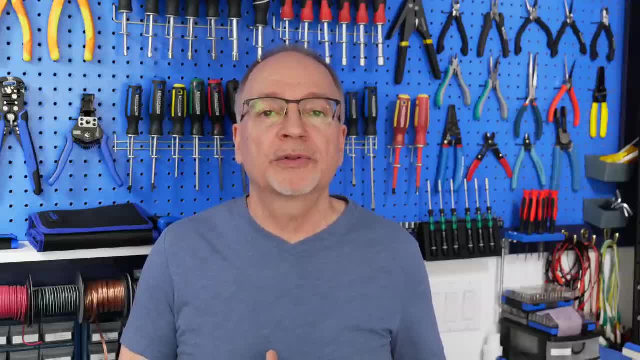 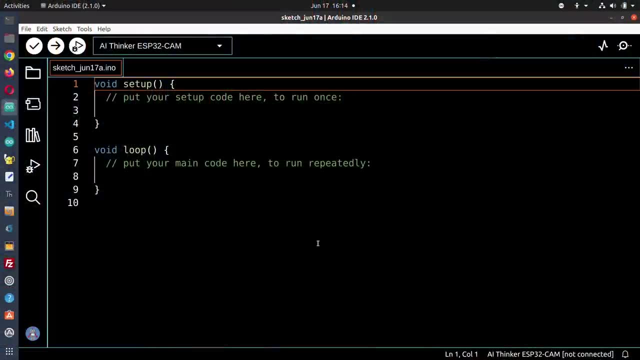 by the library in order to test everything out with the ESP32 cam. So let's go ahead and do that. So, as you recall, Edge Impulse produced a library in the form of a zip file, And we need to install that in our Arduino IDE. 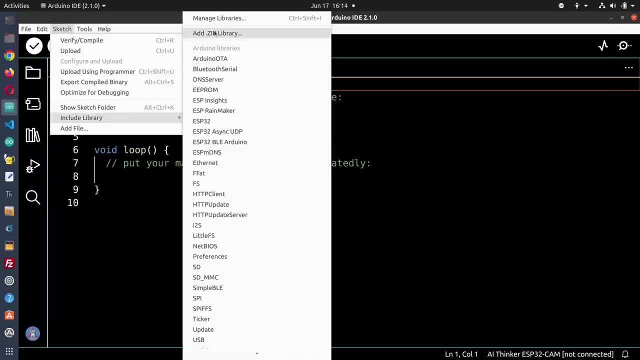 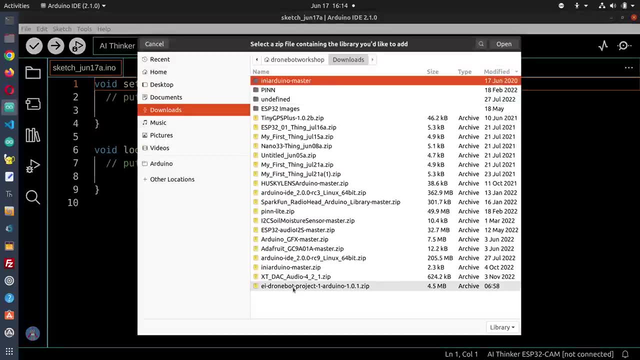 So let's go up to Sketch, Go to Include Library and Add Zip Library, Then go to wherever your library was downloaded to And pick out the library. You'll notice the name of the library has your username in it, And so that's how you can identify this. 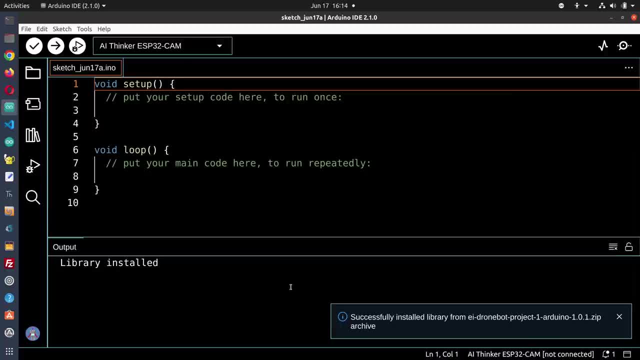 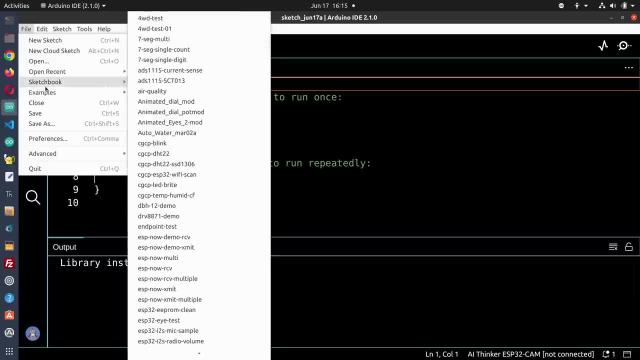 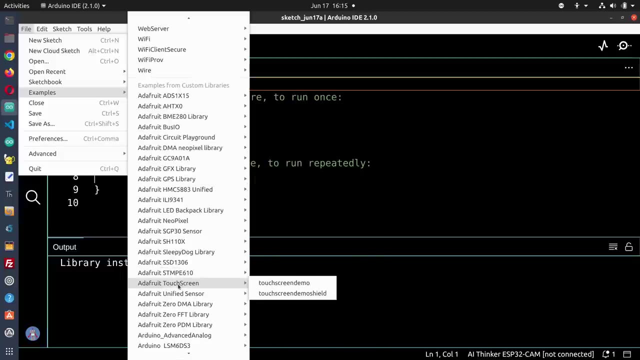 Pick that out And the library has been installed. Now the next thing we can do is go and use one of the example sketches that came with the library. So go down into Examples And go scroll down Examples from Custom Library And look for your username. 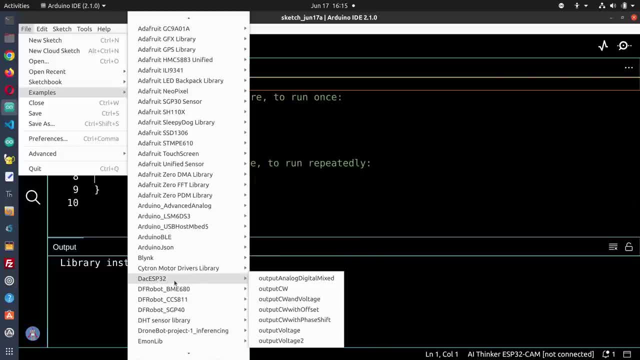 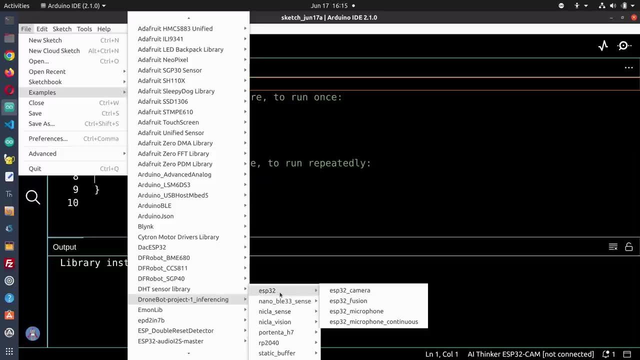 because your library is going to be named after that And here it is DroneBot Project Interfacing, And you'll notice there's a number of different choices here. I'm going to go into the ESP32. And there's a program called ESP32. 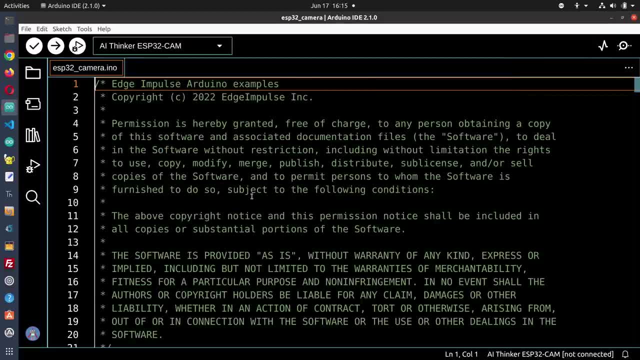 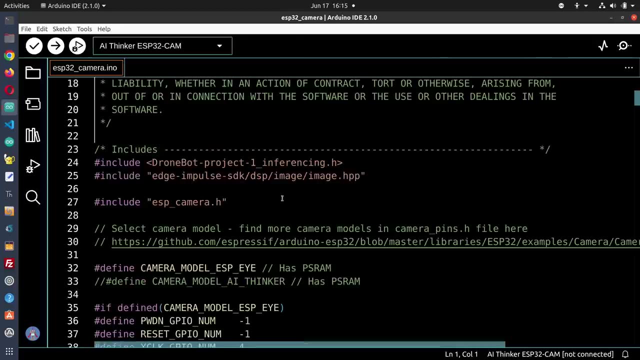 Camera. So we'll load that. And what this sketch does is it uses the camera to identify the objects it's been trained to identify And it prints on the serial monitor the location of that object as it sees it in its field of view. Now I'm not going to go through the whole. 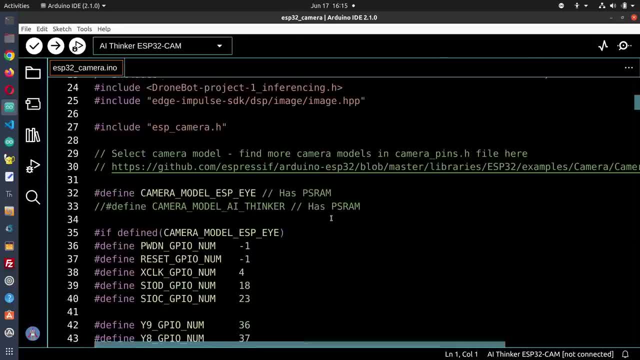 sketch. There's quite a bit here, But there is one line you need to pay attention to, And it's down over here, And this is where you define the type of camera that you're using. Now, by default, it's going to use the ESPI. 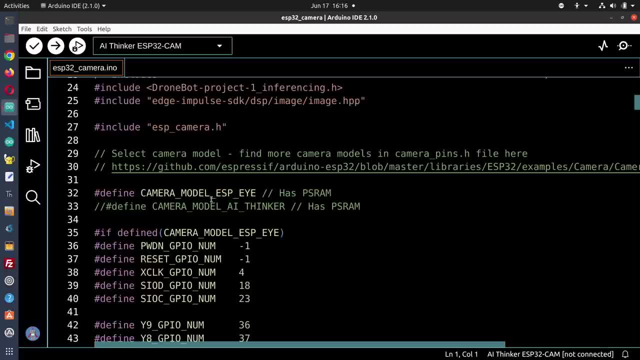 And I'll probably use the ESPI as well, Simply because it's a lot easier to use because of its built-in USB port. But if you want to use the regular ESP32 cam, then you need to remark out line 32 and unremark line. 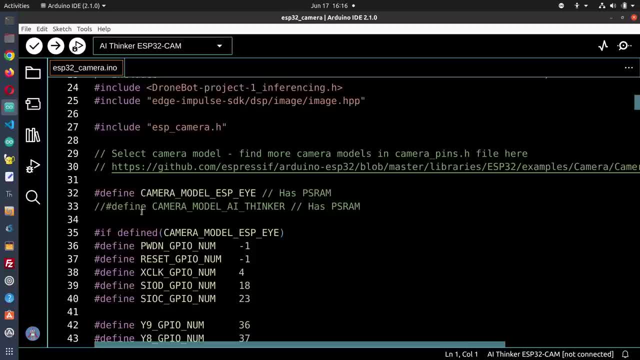 33 for the AI thinker, And that will let you use the ESP32 cam. So all I need to do right now, since I'm using the ESPI, is to load this up to my ESPI camera and we can check it out, And so 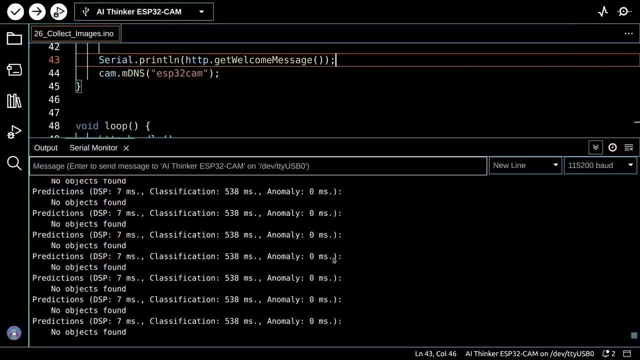 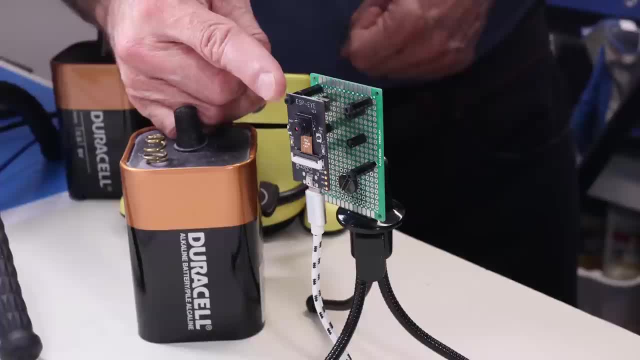 we're ready to test out our ESPI camera and see its object detection capabilities. Now I've got the camera mounted onto a piece of perf board over here And this piece of perf board, you'll notice, has a number of different standoffs on it. They're 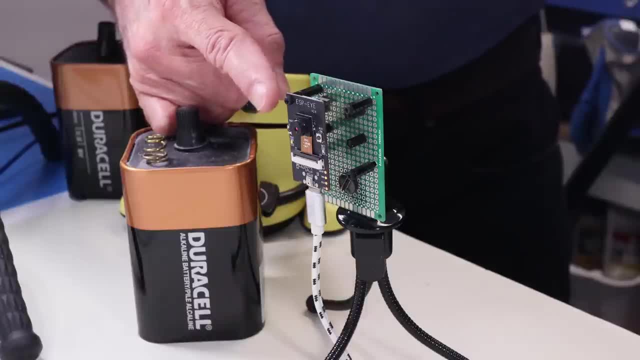 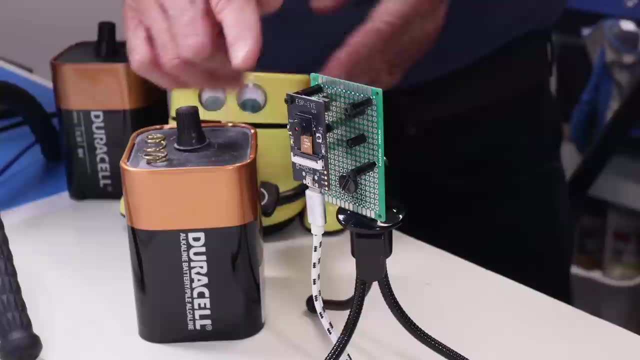 spaced out for Raspberry Pi and Arducam cameras. I've used this perf board before. It's attached to a GoPro adapter, which in turn has a quarter inch thread, And it allows me to put it onto any tripod I want, And I put it onto the same. 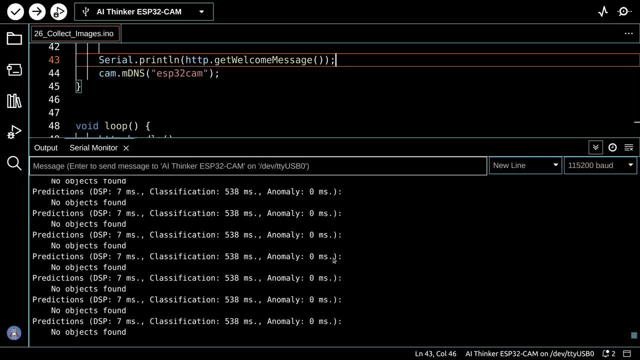 tripod that our webcam was using. I've got everything aimed at my test area And, as you can see in my serial monitor, it's saying there are no objects found. And that makes perfect sense because there are no objects, So let's give it an object. 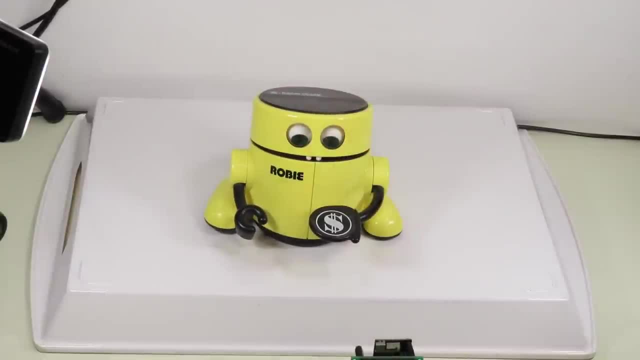 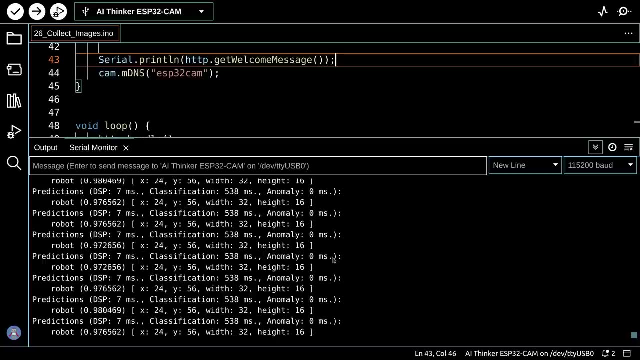 and see if it can find it. Put Robbie there And it seems to have a robot And you'll notice a number right beside the word robot. That's how confident it is that it's a robot And it's pretty confident it's a robot. 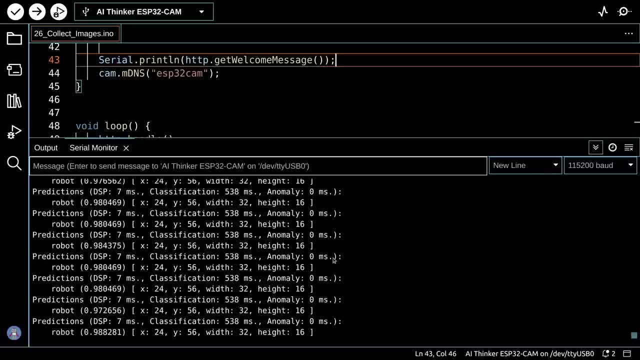 One is perfect confidence, So 0.98 is very confident. We've got an x and y coordinate and that's the top left corner of the bounding box, As well as a height and a width, And that would be the size of the bounding box. 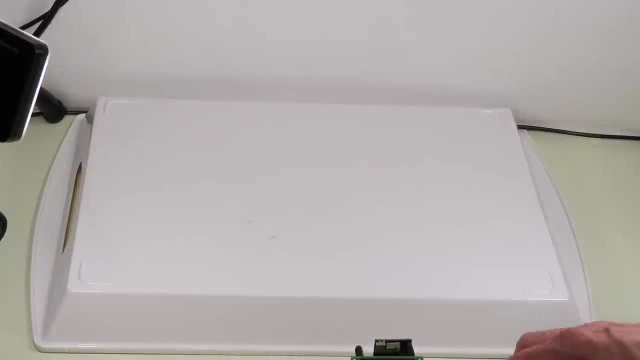 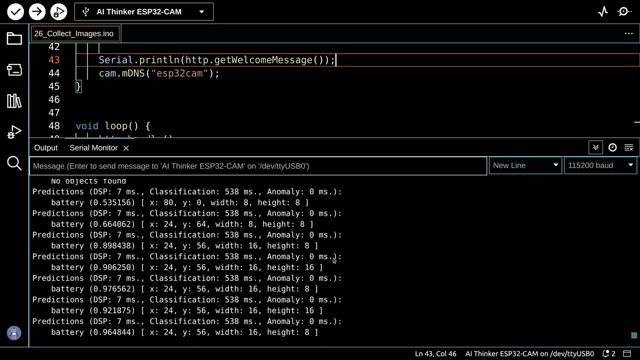 So let's take Robbie out of there And put our other object into here And it's detected it being a battery. And if you noticed, when I first put it in the confidence wasn't as high. but after a couple of iterations the confidence got much, much. 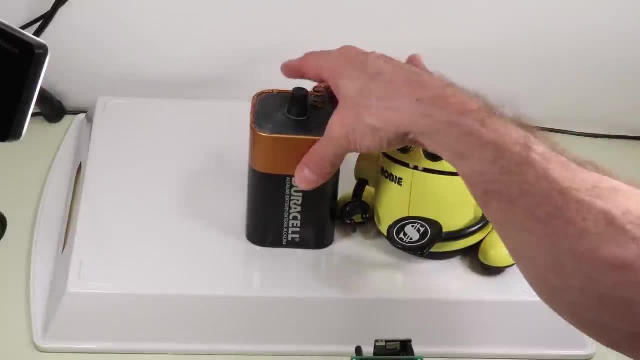 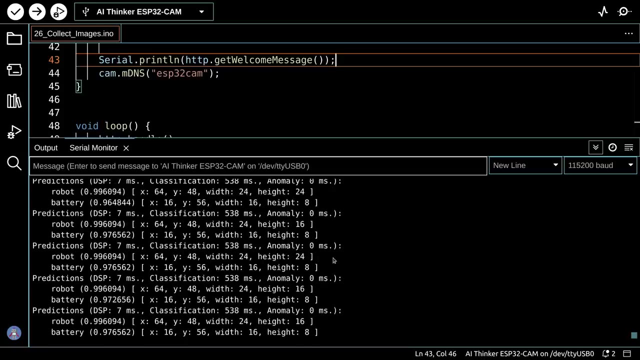 higher. Now let's see what happens if we put Robbie and the battery in. Of course, I can't see the camera's field of view, But it seems to see a robot and a battery, Again with a fairly high degree of confidence. So it seems to be working pretty well. 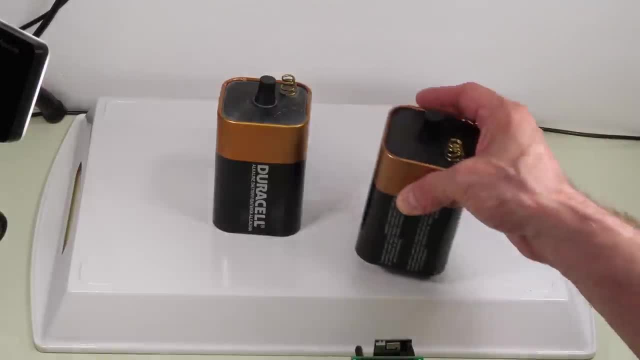 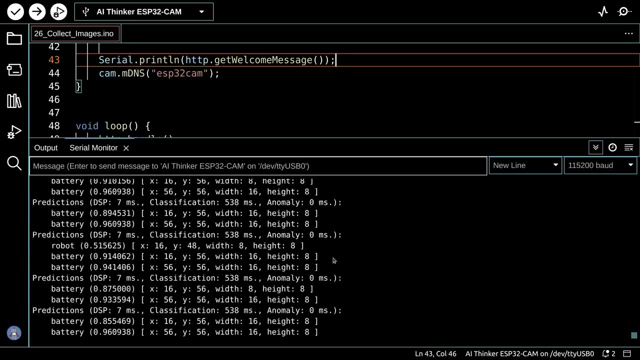 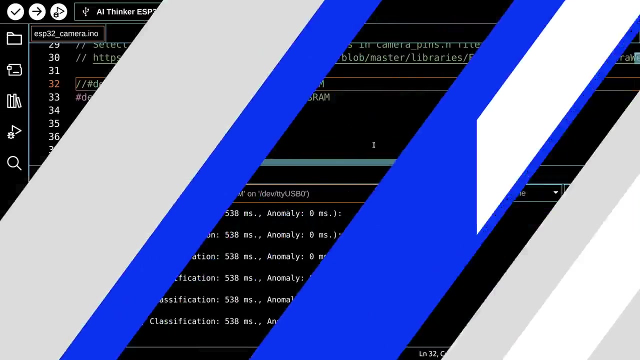 Let's take Robbie out of here And put a second battery into here And it sees two batteries and it gives the coordinates of the two batteries. So our object detection system with the ESP32 seems to be working pretty well. So I thought I'd repeat the experiment using 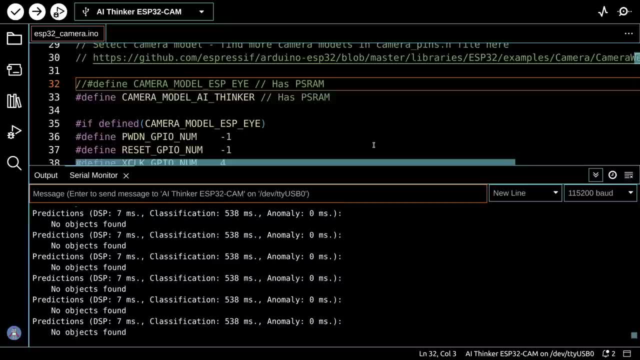 an ESP32 cam, because I figure that's probably the module you're most likely to use. Now, remember, you need to make a small change in the code up here. Line 32 needs to be remarked out, where we've defined the model of the camera. 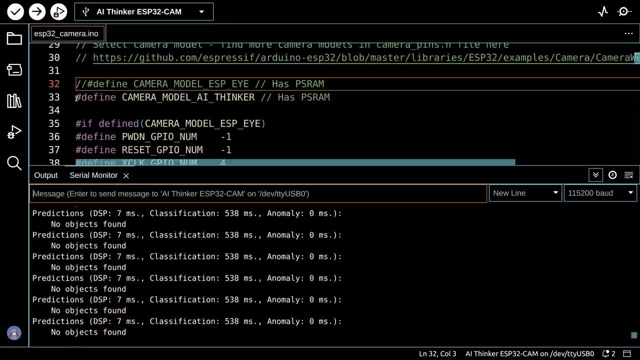 as the ESPI And you need to unremark line 33, which defines it as AI Thinker, And that's the only change you need to use. By the way, I was able to use the same entry in the Boards Manager: the AI Thinker, ESP32. 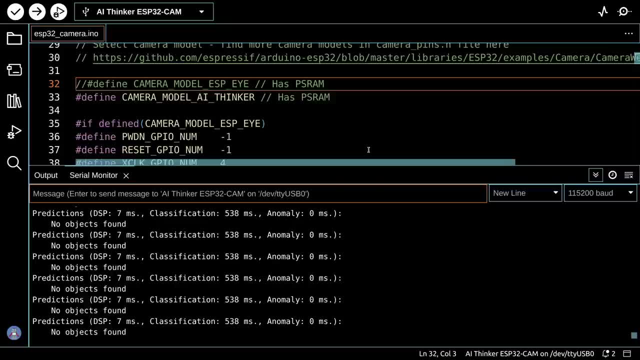 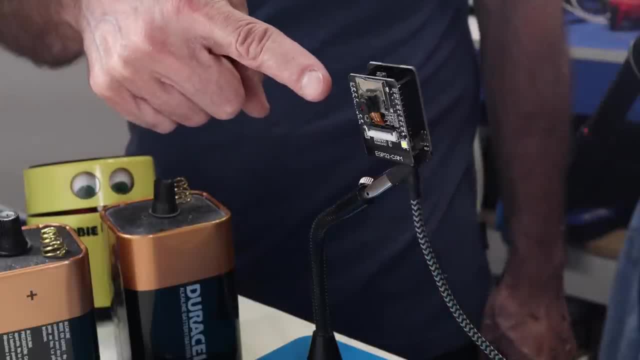 cam for both the ESPI and the ESP32 cam module. Now I've got my ESP32 cam module mounted onto one of those adapters and I strongly recommend using that. It makes the camera a lot easier to use. Now it doesn't have a mounting hole. 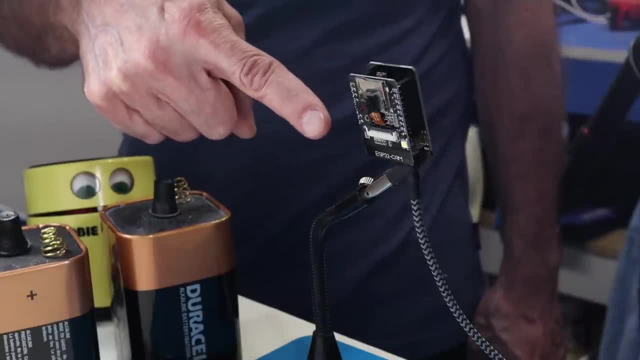 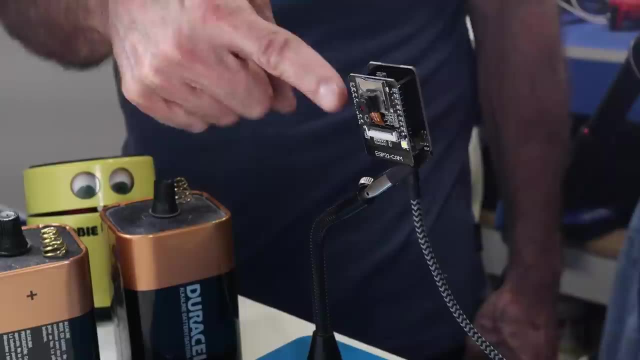 so what I've done is I've taken one of those clips that you use for holding wire when you solder, and I've just clipped that onto the micro USB connector. So that's all that's holding it up. It's not the best arrangement, but it does seem to be working. 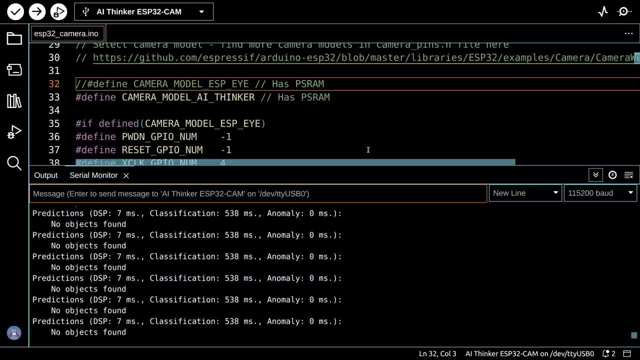 And if you look, of course I see no objects found, because I have no objects And I'll give it an object And we'll see if we can find it. And it does indeed find a battery with a pretty high level of confidence, And so we'll get our friend Robbie. 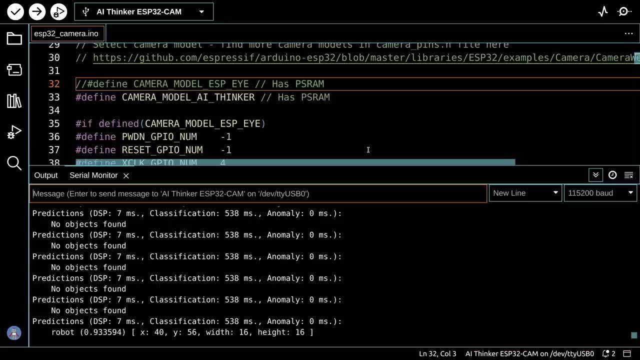 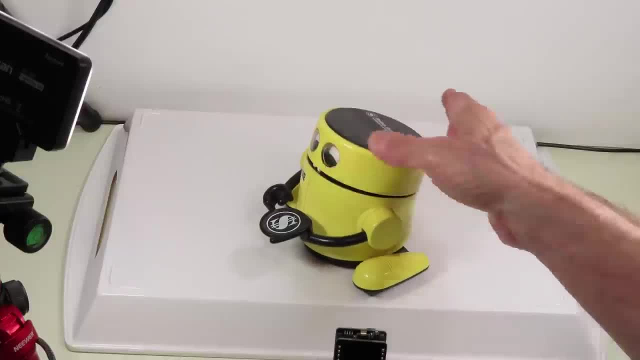 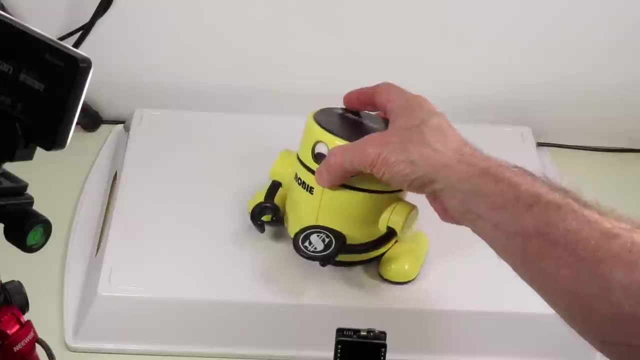 out here And it seems to find a robot as well. Let's turn Robbie to his side and see if it can spot him, And it still has a fairly high degree of confidence that we have a robot here. We'll turn him the other way. 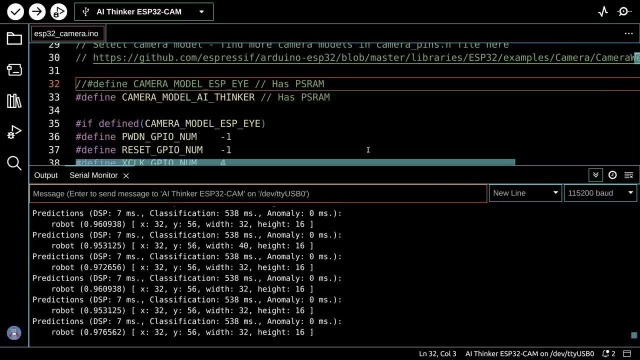 And again it can detect a robot. We'll turn him this way backwards And the confidence is down quite a bit, but it still does detect a robot. Now, of course, a lot of this just happens to be the number of images of Robbie I took, and from what? 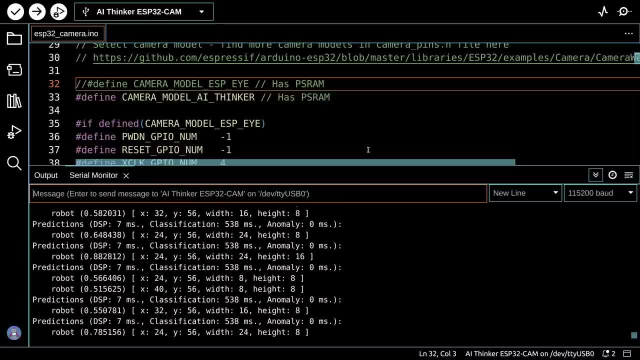 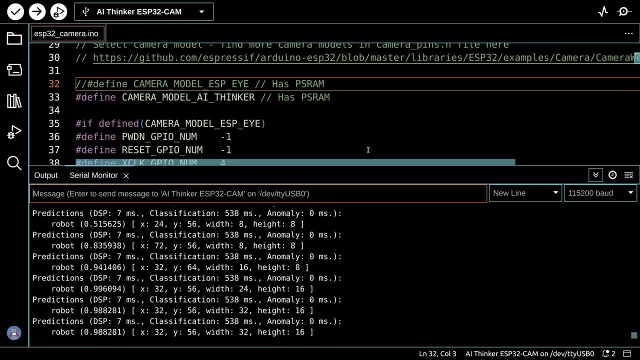 angles I took them at And if I had trained with more images and more angles it could have a higher confidence. But it does seem to be able to detect the robot at just about any angle and it seems to work just as well as the ESP-I. 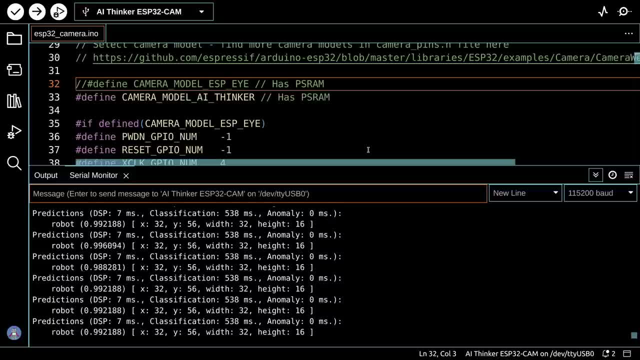 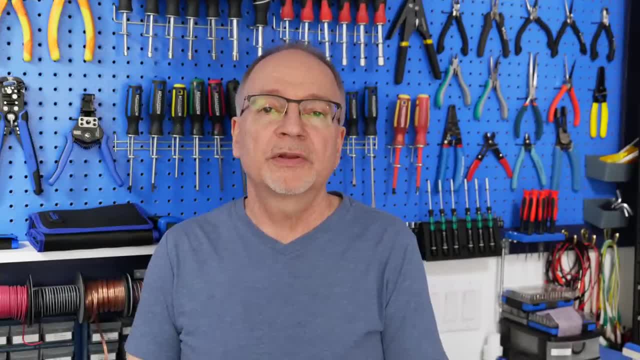 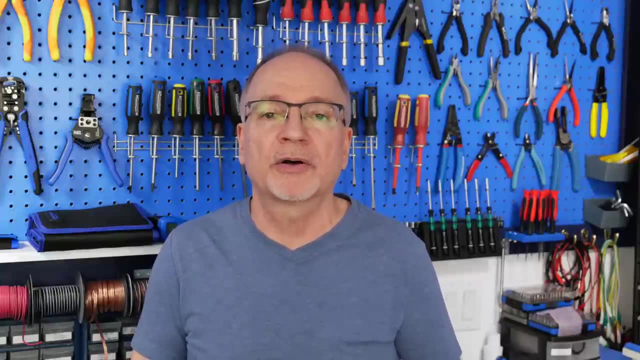 and they both seem to work very well and since this is a $9 module, it's a very inexpensive method of doing object detection. So now you've seen the entire workflow that's required to create object detection with the ESP-32, and that workflow started off with. 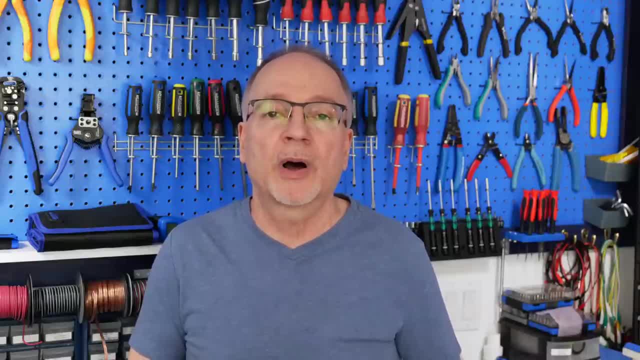 capturing the images. Now, when I illustrated this to you, I used a webcam to capture my images, but, as I mentioned earlier, there are a number of different ways that you can capture images for use with Edge Impulse, and one of those methods is to use the ESP-32. 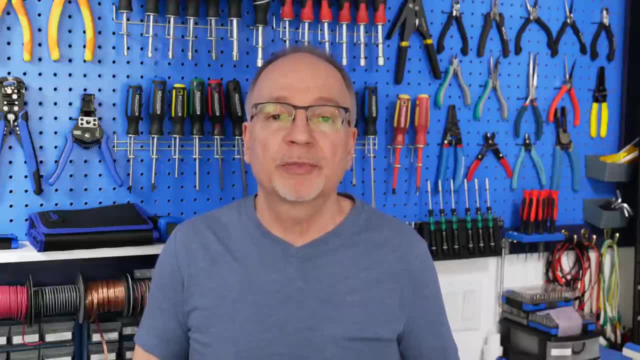 cam itself. In some ways, this makes a lot more sense, especially if you're using the camera in a fixed position, because you're using the same camera to capture your images and train your model, as you're going to be running the model on Now, you 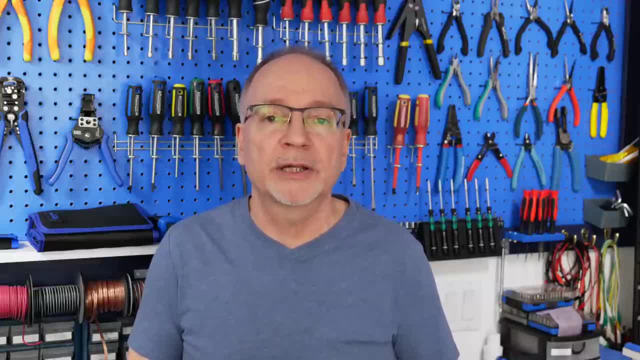 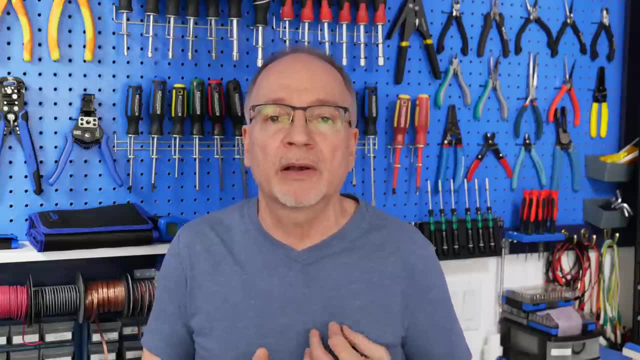 can connect the ESP-32 cam directly to Edge Impulse in the way that we use the webcam. however, this requires using the ESP-32 CLI or command line interface, and it's a bit complicated. There's another way of doing this that I like better, and that's. 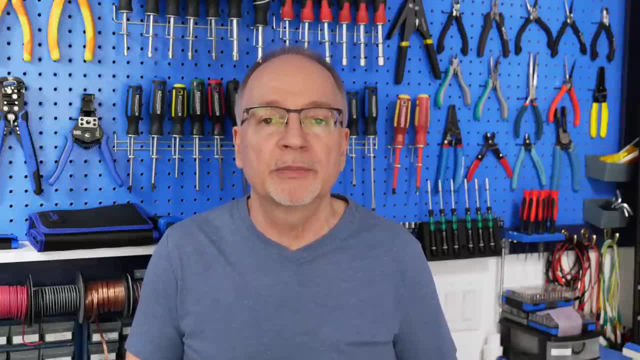 just to use the ESP-32 cam to capture our images and then upload those images to Edge Impulse and after that proceed with the same steps we did before. So that's what we're going to do Now I'm going to be making use of 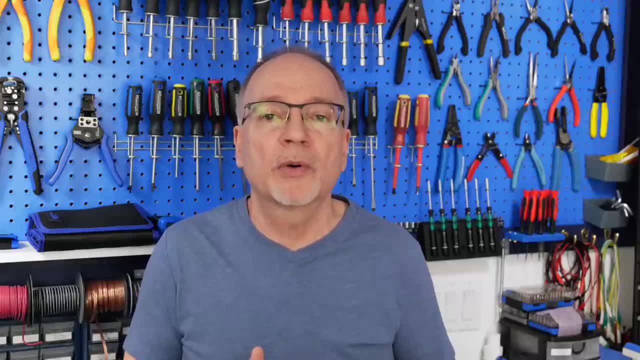 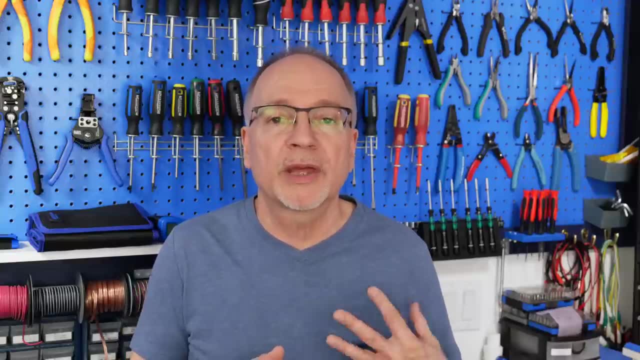 a library from Eloquent Arduino, and Eloquent Arduino has a number of different libraries for use with the ESP-32 cam, including many of them that work directly with Edge Impulse, and there's an example file we can use to capture all of our images. So let's go. 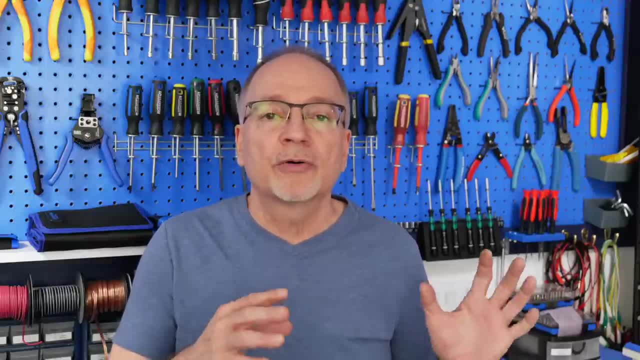 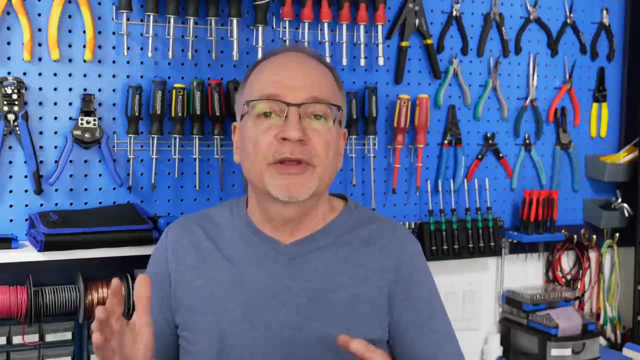 and load that library up and get some images and go through the entire process, and then, when we play back the images, we'll also use some features of Eloquent Arduino instead of the sample code that came with Edge Impulse. Let's go ahead and do that. 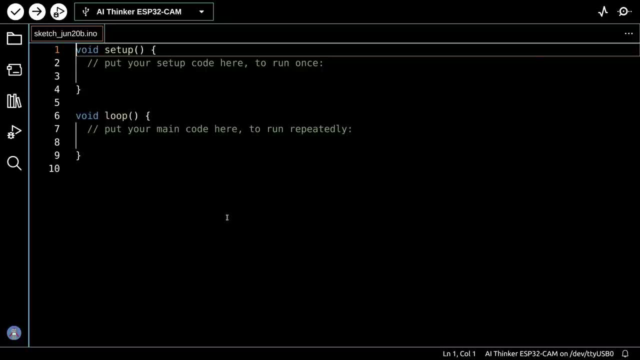 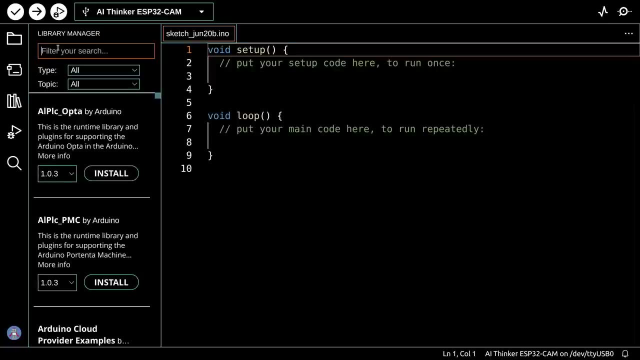 Now the library that we're going to need to install is called the Eloquent ESP-32 library from Eloquent Arduino. So go into your library manager and start typing E-L-O-Q. that should get you down to the number of Eloquent Arduino's. 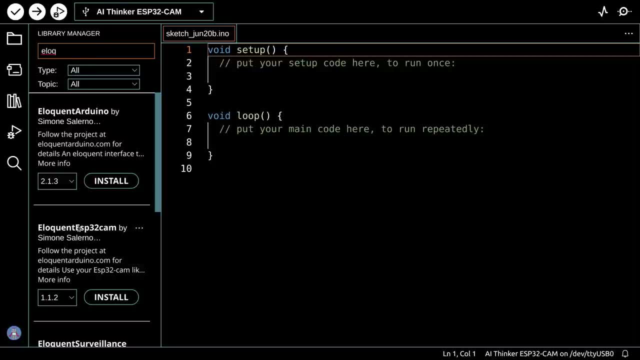 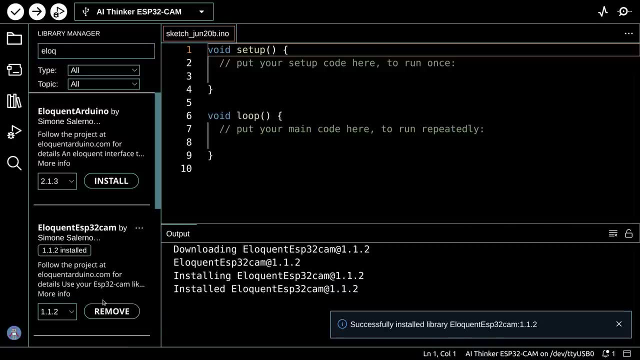 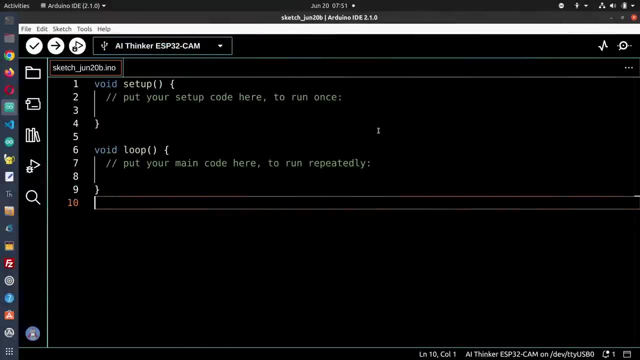 and you'll notice a number of libraries. it's the Eloquent ESP-32 cam library that we're going to install, So click on install for that, And now the library is installed. Now that we have the library installed, we're going to use one of the example sketches included. 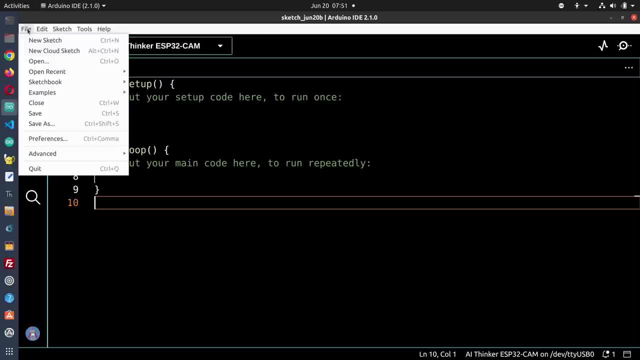 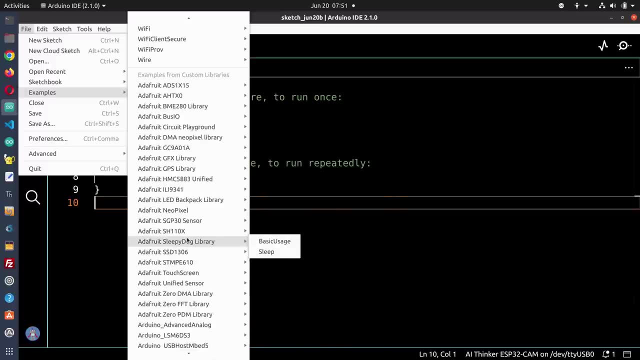 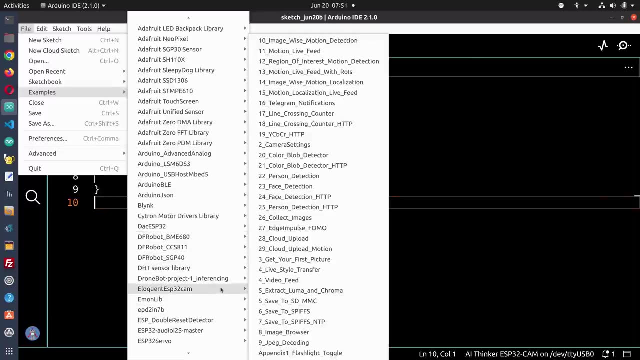 with the library in order to capture our images. So we'll go into file and we'll go into examples and we will scroll down to examples from custom libraries. we'll look for Eloquent ESP-32, which we come to here, and we see a lot of different examples. 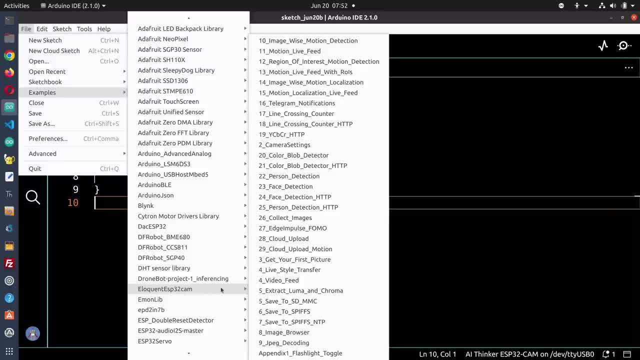 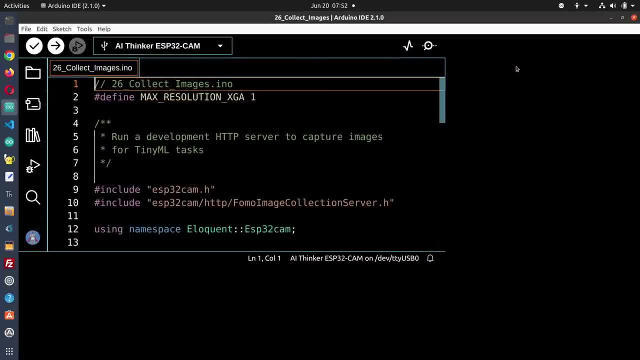 so you can get an idea of all the different things that you can do with this library, And we're going to go for number 26 here. Collect images, So let's make that bigger so we can see it. Now there's a couple of things we're going. 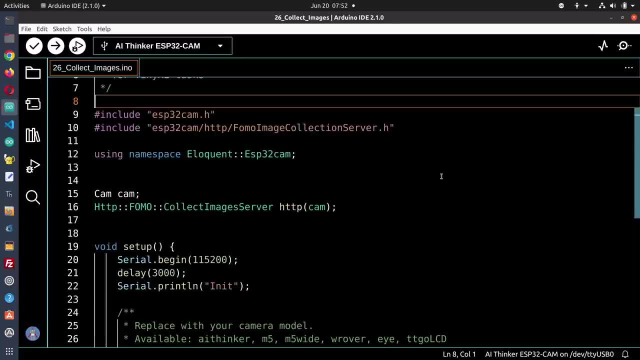 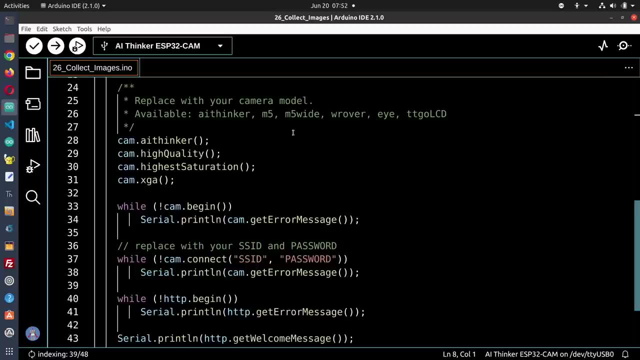 to need to modify on this sketch in order to get it to work. The first thing you're going to need to do is to put your camera model in over here, So you have a number of different types of cameras that you can place in. 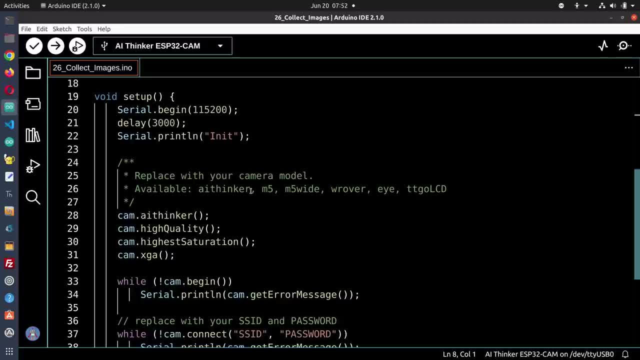 So we're going to probably just keep using the ESP-32 cam and that's the AI thinker. So this is correct for us over here. but if you were using, for example, the ESP-i camera, you would replace this with i over here, etc. etc. Now 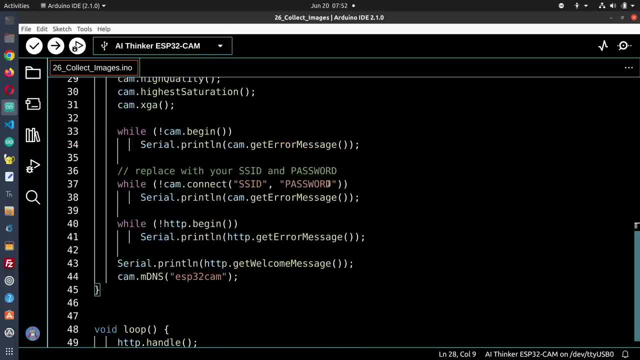 we also need to add the SSID and password for our local area network so that we can connect. So I'm going to modify this sketch and we'll load it up to the ESP-32 and we'll check it out Now, after you load the sketch onto the. 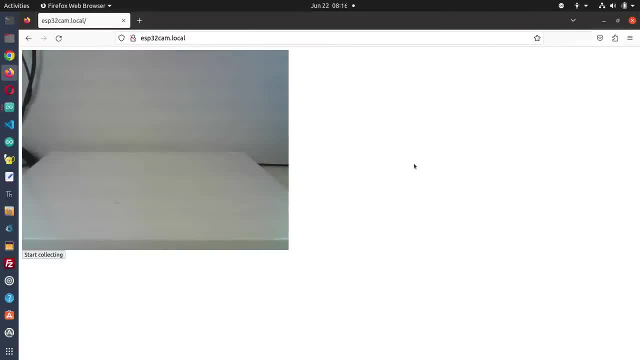 ESP-32. if you look in the serial monitor, you'll see an IP address after it connects to your local area network, assuming you gave it the correct credentials, of course. You can use that IP address in a web browser to go to the screen that I'm on right now. 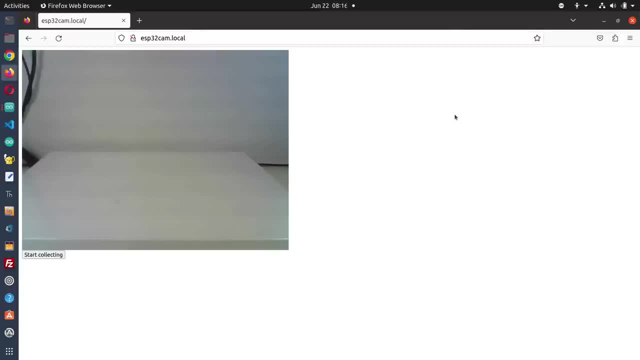 or you can just go to esp32camlocal and, assuming that your router supports mdns, that'll also bring you to the screen and it's easier than remembering an IP address. Either way, we're looking at an image right now of what the ESP-32. 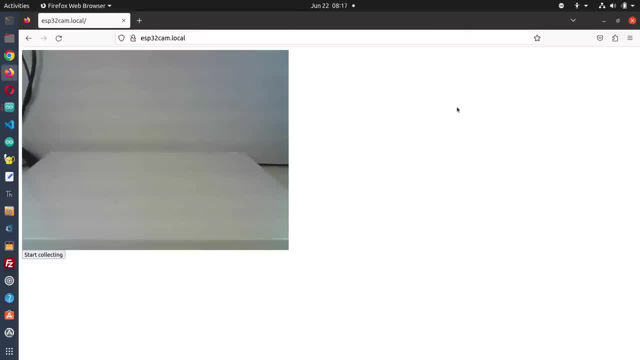 camera sees, and it's a square image that's been designed that way on purpose. Now we're going to do something a bit different when we do our collection of images today. First, we're going to take an image of nothing, in other words, an image of the background. 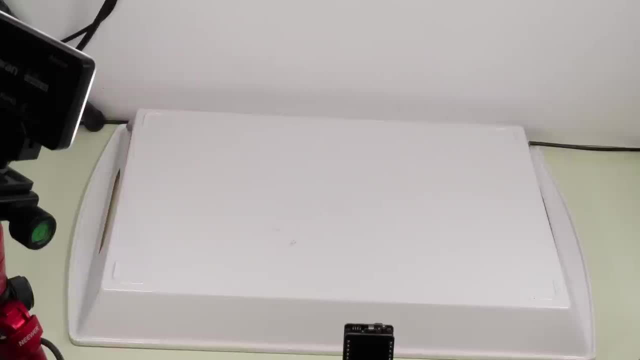 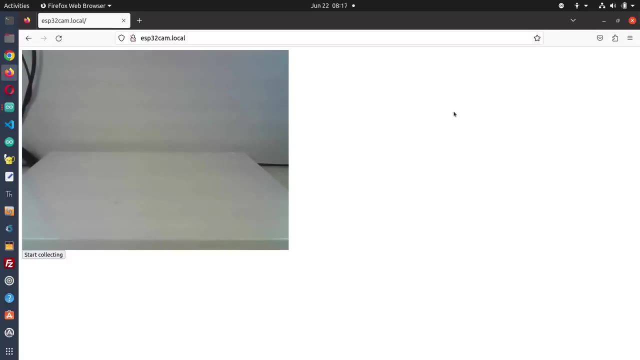 and we're going to use that during training to eliminate the background from the other images. It's a technique we didn't use last time, but it can sometimes increase the accuracy of your object detection. So you'll see a little button here that says start collecting. 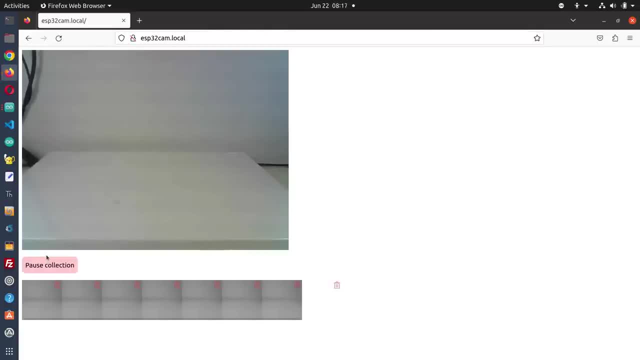 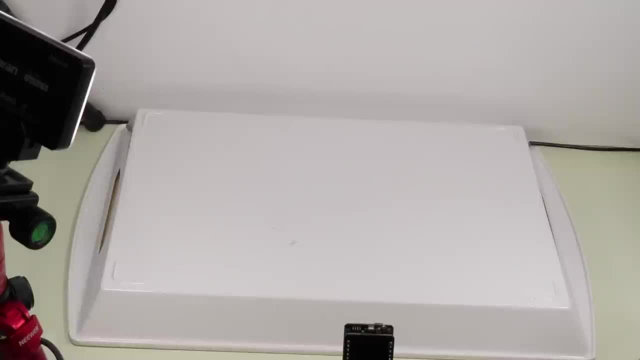 I'm going to click on that button and it's making a collection of images right now. it's just continuing to collect images and, of course, this is an image just of my background. I probably don't need too many images of the background because it's never going to change. 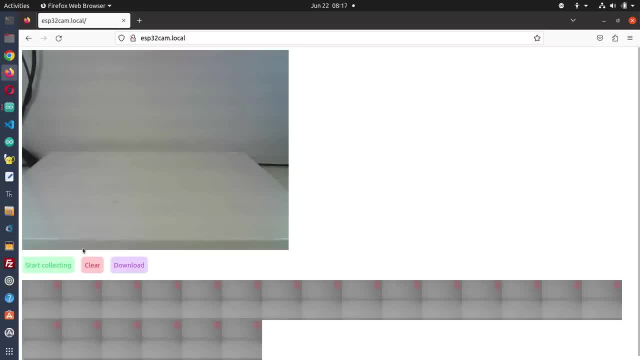 so I'm going to pause the collection and I get a couple of buttons here. I can hit start collecting to continue collecting more images. I can clear all my images or I can download my images, which is what I'm going to do right now. So let's. 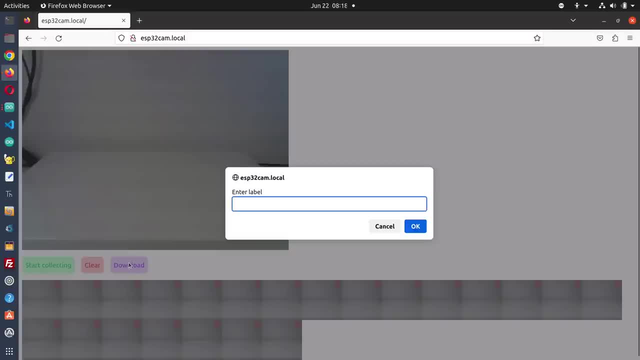 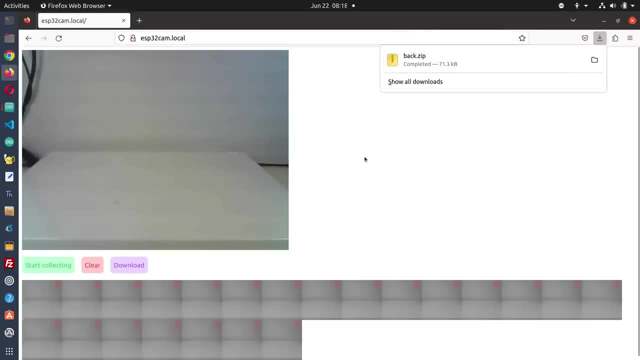 just download the images. I'm going to give them a name, I'm just going to call them back. that's my background. and it downloaded a file called backzip and that zip file will have all the images that I just collected. So now I can hit clear and I can. 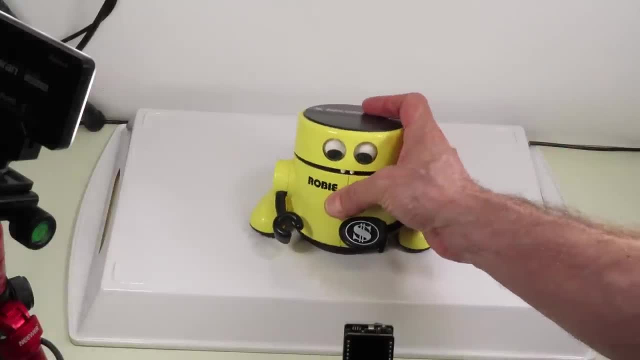 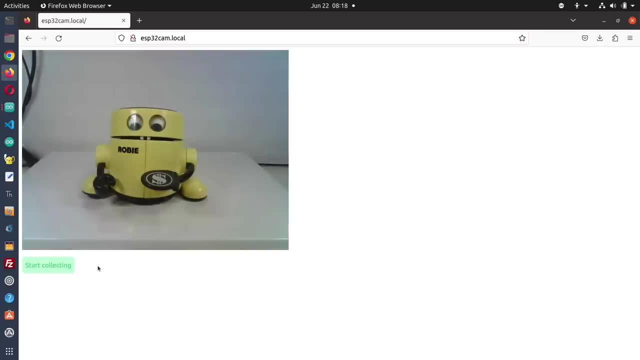 put an object on. so we'll go for Robbie over here and we'll position him now. you'll notice a little lag sometimes in the image. that's normal, don't worry about that, and we can do start collecting. so let's collect some images of Robbie and I'll pause my Robbie collection. 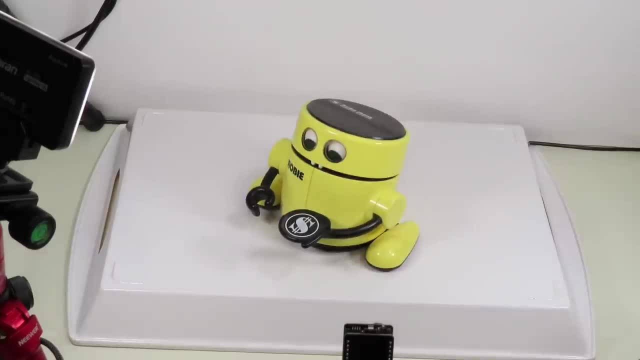 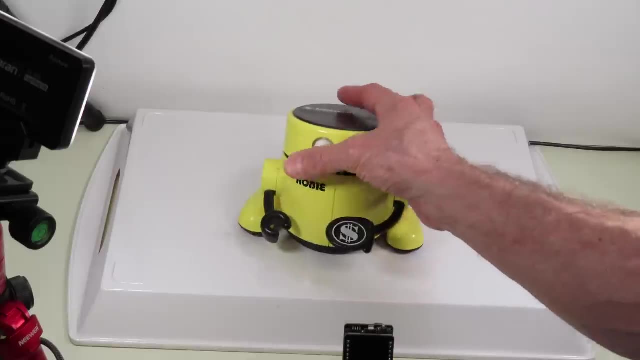 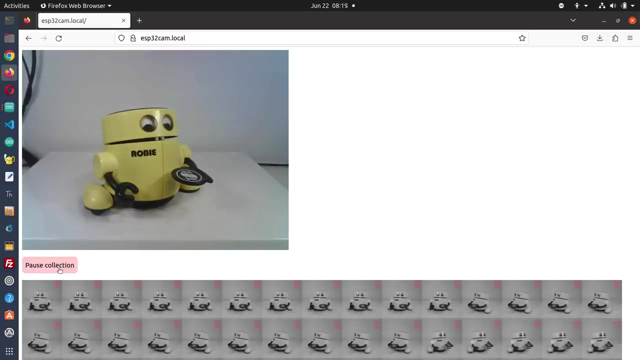 and I'll move Robbie a little bit and we'll start collecting again and once again I'll pause and I'll move and I'll just continue to do that in order to collect images of Robbie. and the collection is still going on. I have to scroll the screen down to see it. 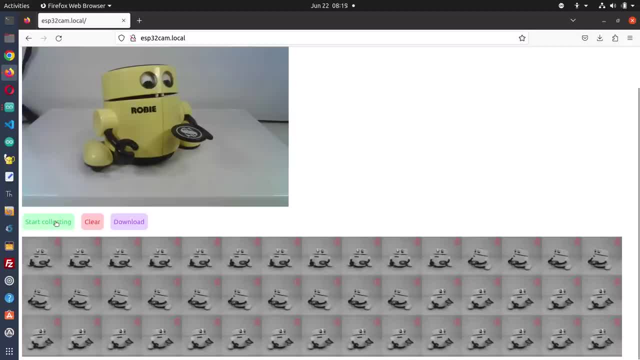 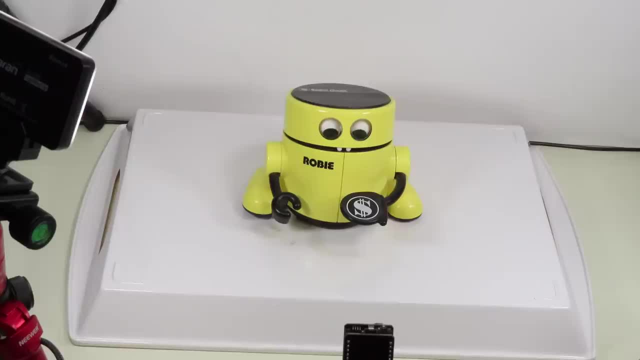 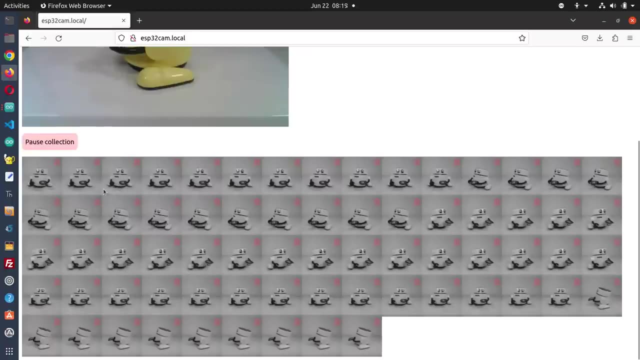 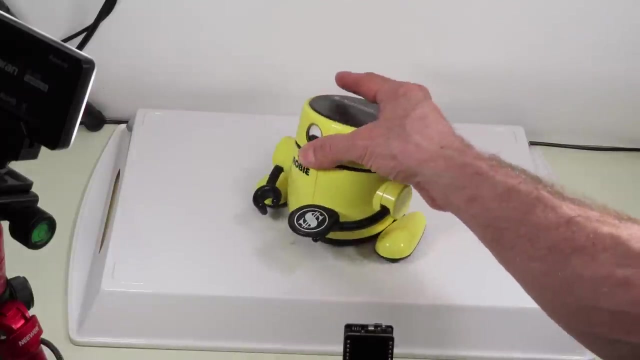 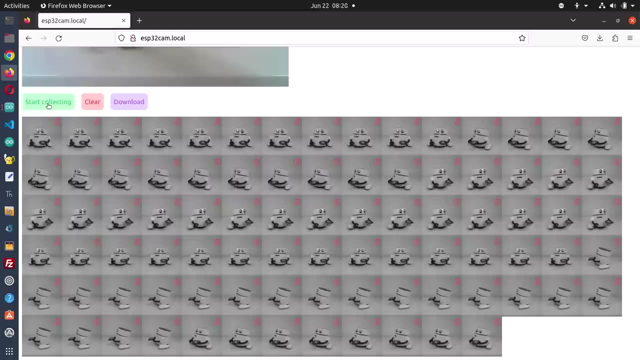 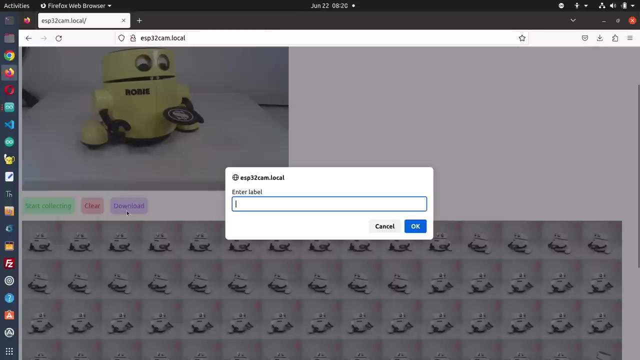 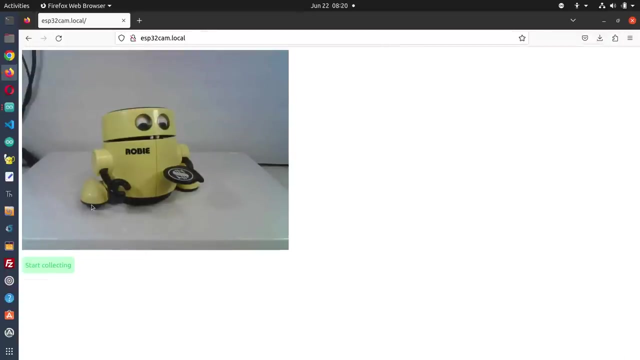 and pause that. give it a more distant image of Robbie, and you'll note that it's collecting black and white images of Robbie too. that's intentional, and I think that's probably enough images of Robbie, so let's download them and we'll get Robbiezip and I'll clear everything to. 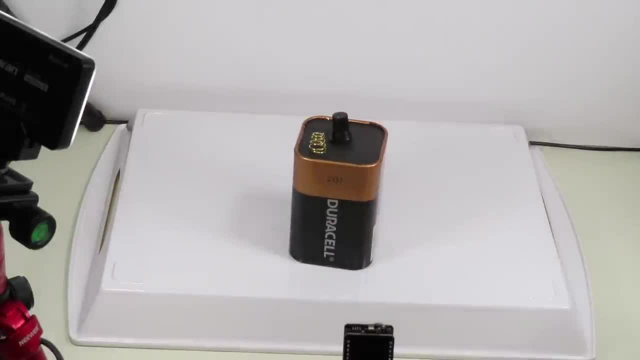 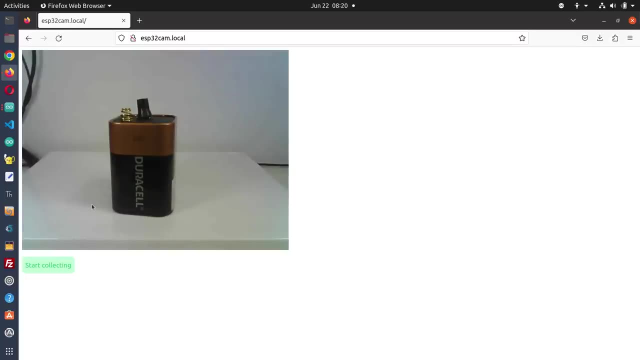 Robbie out, put my battery in and repeat the process for that, and so I won't make you watch me do the battery. it's exactly the same thing, but the gist is that what we're going to do is collect images, and they'll all end up in a zip file. 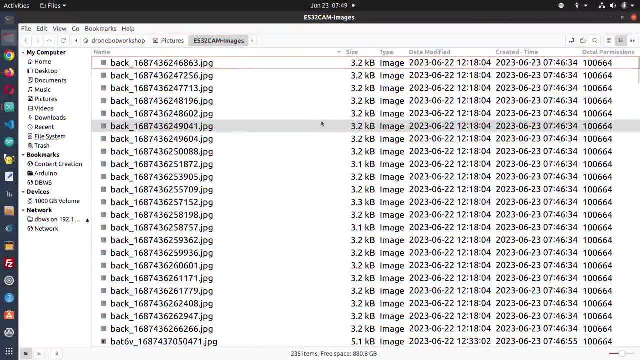 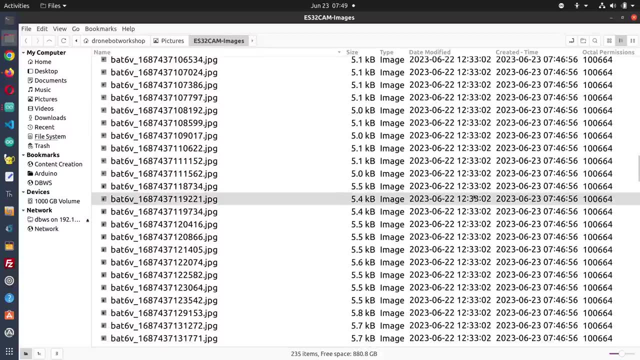 so I downloaded the three zip files that were created for me by the utility and I extracted the contents of them all into one direction. now you could extract them into separate folders if you wish, but because I labeled all of my files differently, I can tell which ones are the. 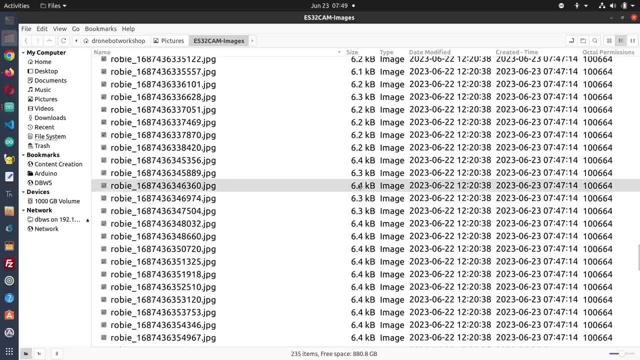 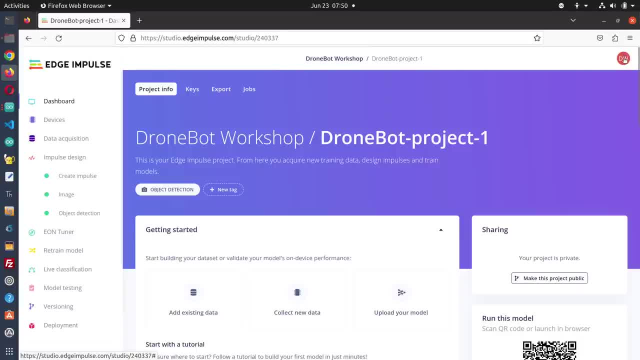 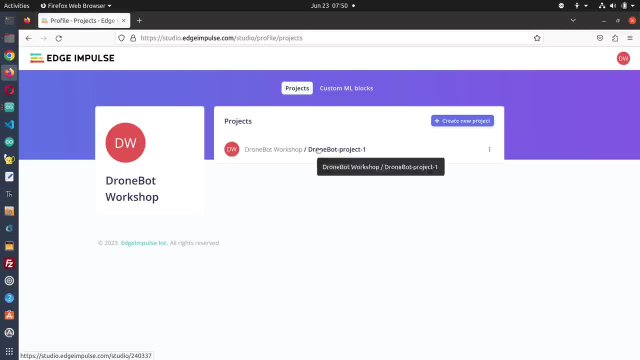 batteries, which ones are the backgrounds and which ones are Robbie? and so now I'm going to go into Edge Impulse and in Edge Impulse we're going to create a new project. so go over to your own profile logo and click on projects and you'll see the one project that you have. 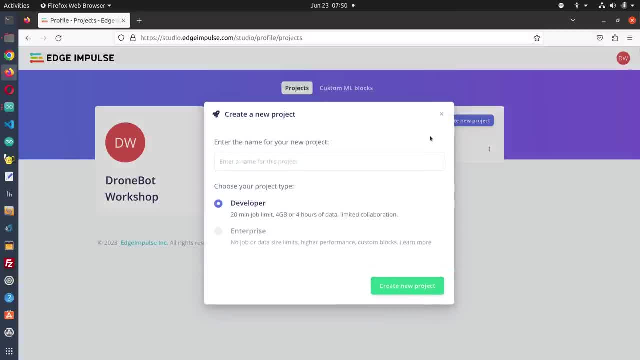 right now, do create a new project and we'll have to give the project a name and that's good enough, and it's set as developer, which is the type of account we want to use, and we'll create a new project and we're now in our new. 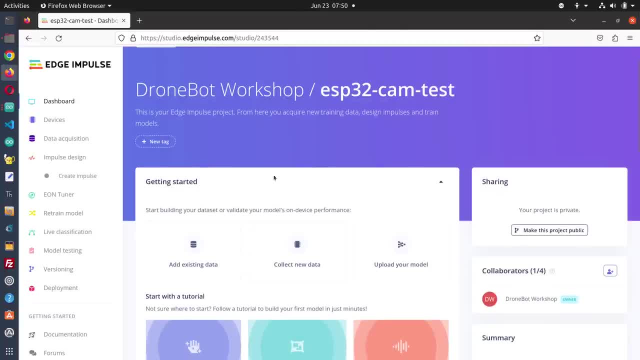 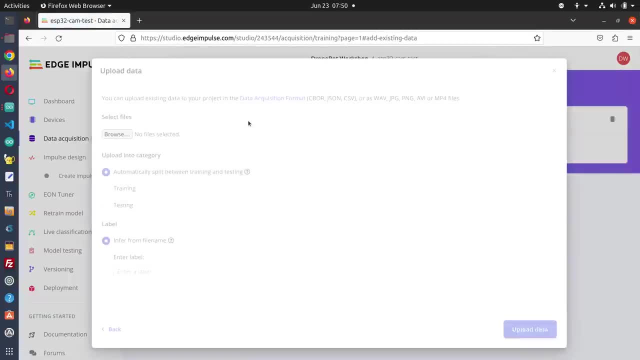 project and we need to add some data to the project and, of course, that data is going to be the pictures that we just took. so let's do add existing data and we can do upload data. we'll have to navigate with the browse to where that data 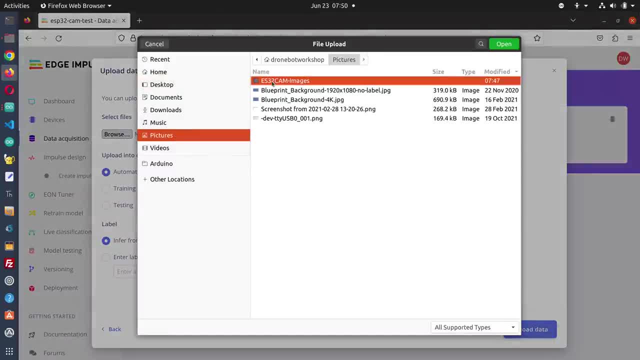 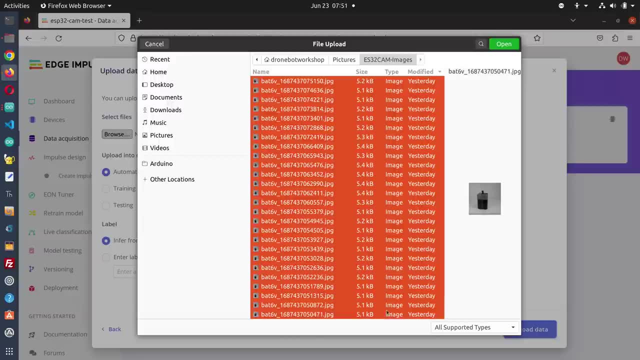 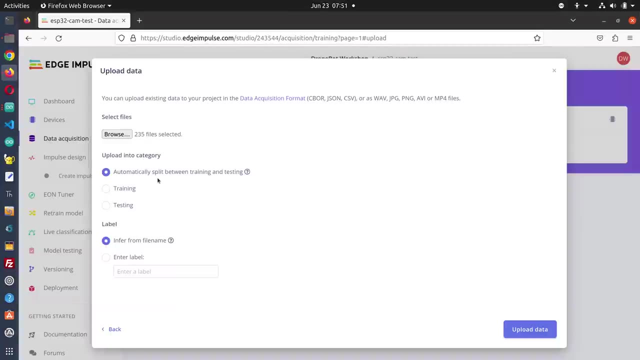 is and I put mine in the pictures in my ESP32 cam images directory and I'm going to take everything in this directory and I'm going to open that and I've got 235 files selected. I'm going to leave automatically split between training and testing. 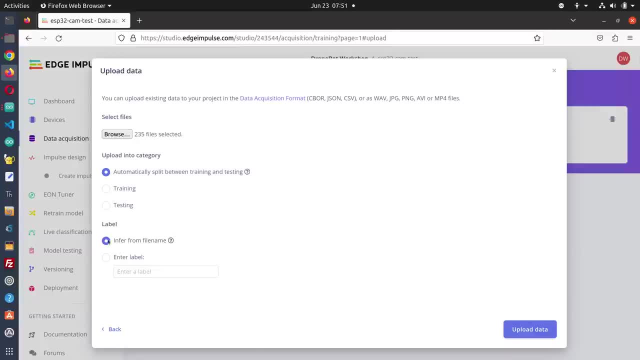 you can set them as training or testing images. otherwise, and we're going to label them and we're going to infer the label from the file name. so every file name started off with a distinct label. so there should be three different labels. we get and we're going to. 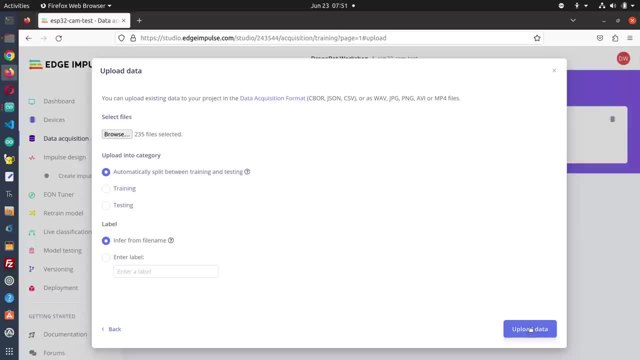 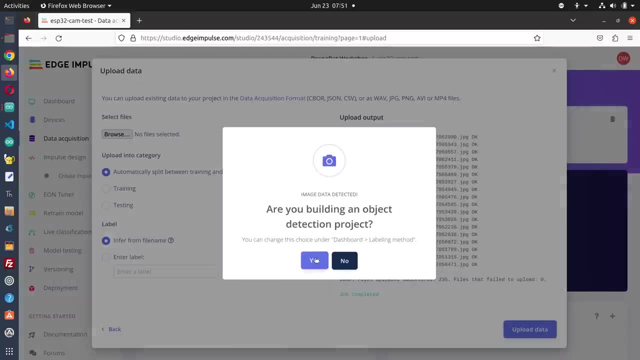 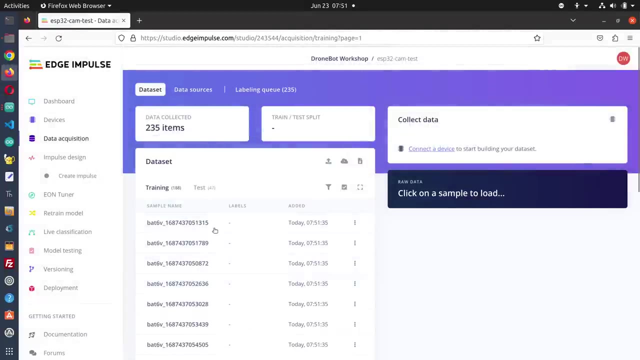 upload the data now. don't confuse that with the labeling process, with the bounding box. that comes next and it asks if I'm building an object detection project because it detects its images. and I say yes, I am building one and we're complete over here, and so now we have a number. 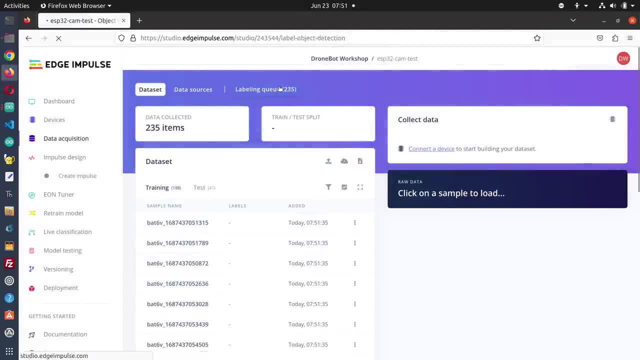 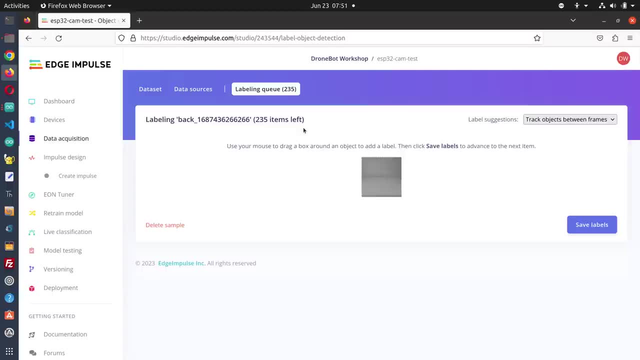 of pictures and of course, we've got to go into our labeling queue. so we'll go into the labeling queue and we're on the first image. now. this is very important, remember I did a number of images of the background. I don't want to assign any kind of 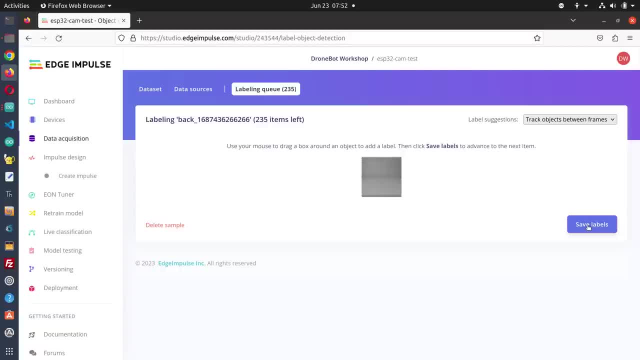 a label to these. so I'm going to do save labels without actually entering a label here and, if you'll notice, the number that I have left to do is incrementing. so, although they look the same- because they're basically the same picture- we are saving labels. 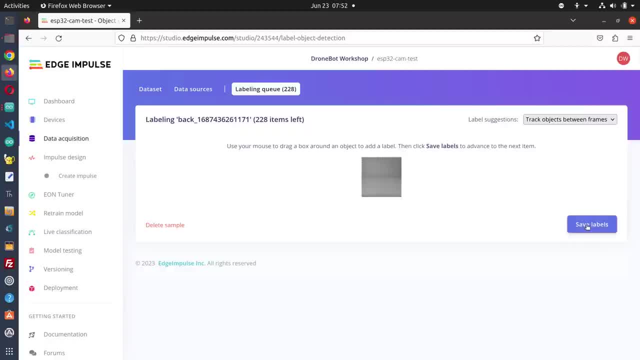 we just got to wait until we get to the first image I took that actually had either the robot or the battery. I think alphabetically it'll be the battery. here we go. it's the robot. I was wrong, and so now we have to draw a bounding box and of 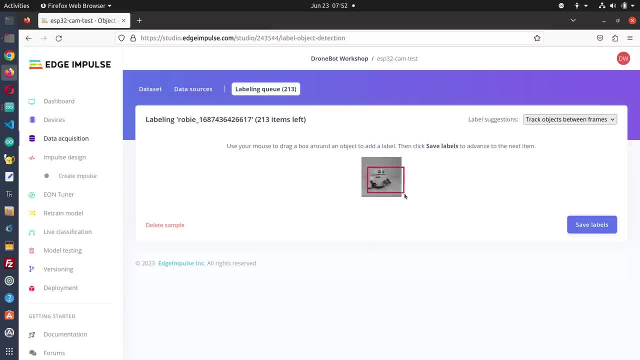 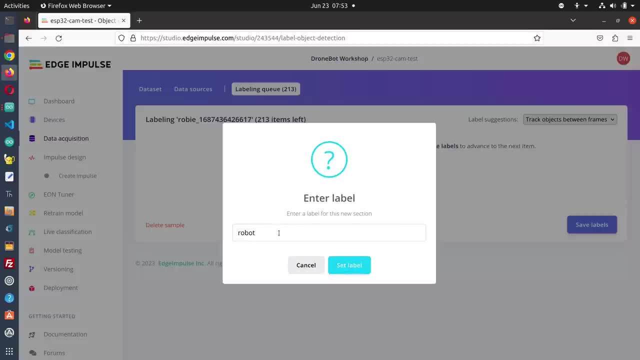 course it's a very small image, but try to do the best you can and we'll draw a bounding box around Robbie and we're going to have to enter a label for this now and we're going to label him robot and we set the label and the bounding box. 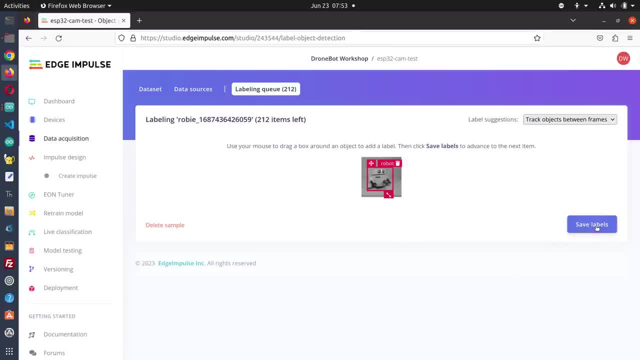 is there and we save that label. and now we've gone down. this is the next image. you remember the way I took it. we're going to get a sequence of images that are all the same and we just go and save the robot label for Robbie. now, of course, I've got. 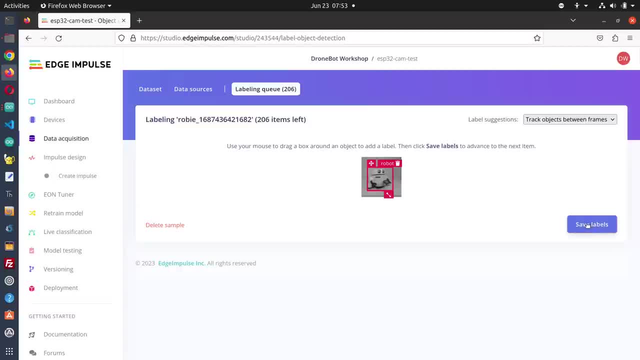 quite a few images of Robbie, so I'm not going to make you watch me do this, but essentially I'm going to go through this until I get the images of the battery that I'm going to go up over here and I'm going to change the label by clicking on that little garbage. 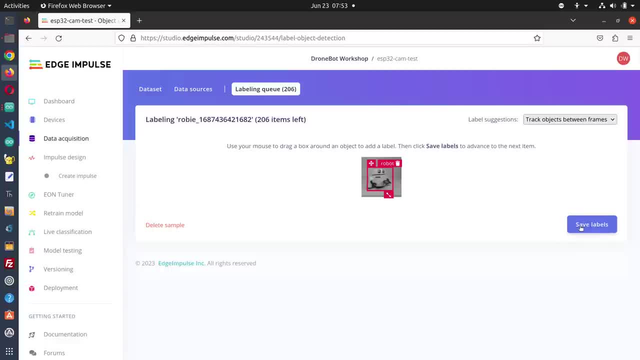 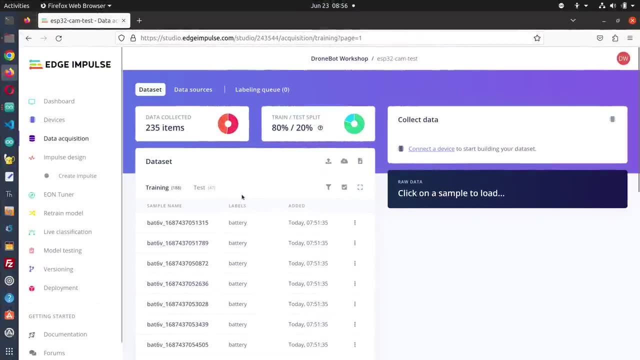 can over there and label those ones battery and continue to save the labels, and so I'll finish doing that and I'll meet you back here. alright, I've gone through all of my images and, as it says here, I have 235 of them and it split them into a. 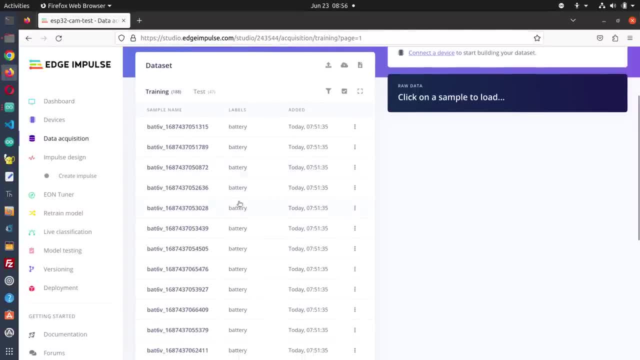 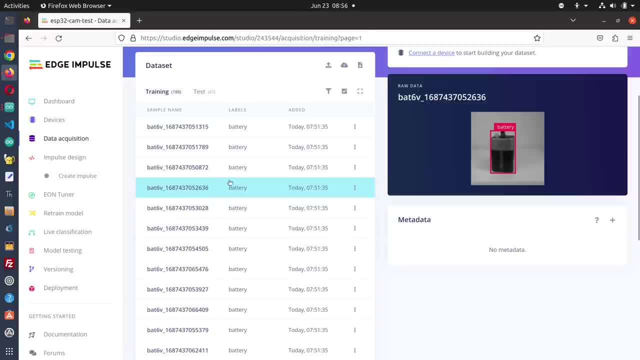 training and test ratio of 80 to 20. now I can go back and edit the images if I wanted to, but I think they're pretty good. remember, I have a number of background images that have no label assigned to them. so the next thing we need to 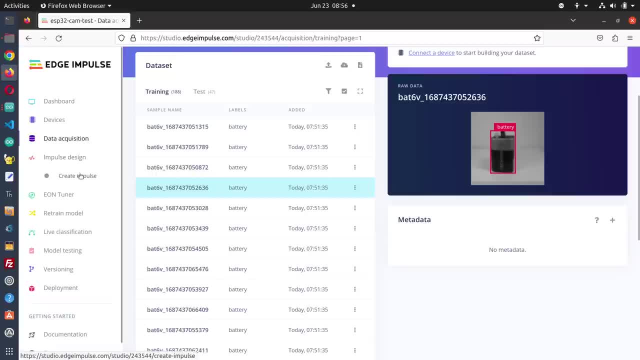 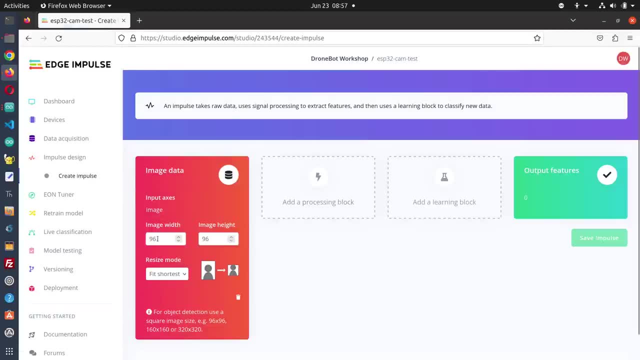 do is design our impulse. so, on impulse design over here, I'll go to create impulse. and you remember this screen from before. now, the images are currently 96 by 96, but eloquent arduino actually recommends that you make them even smaller, 48 by 48. so I'm going to do. 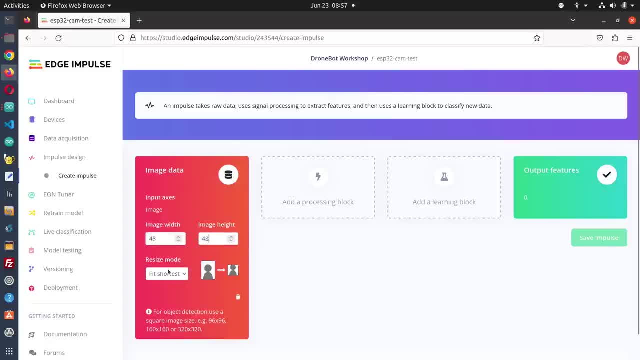 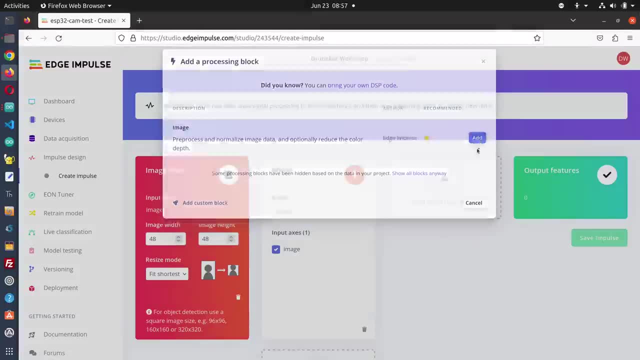 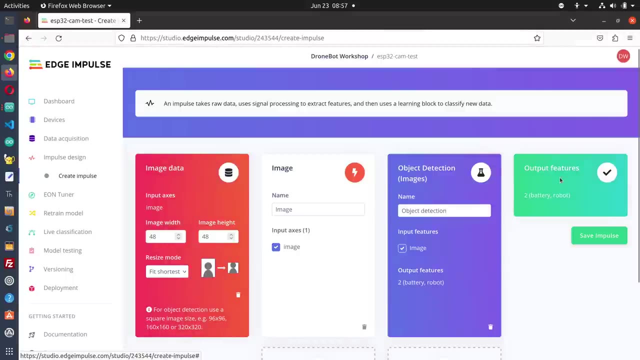 that and we'll keep the resize mode. it fits shortest. we'll add the processing block and the only one it really has for us is an image processing block, and we'll add a learning block and we'll add the one on the top, object detection, and the output has. 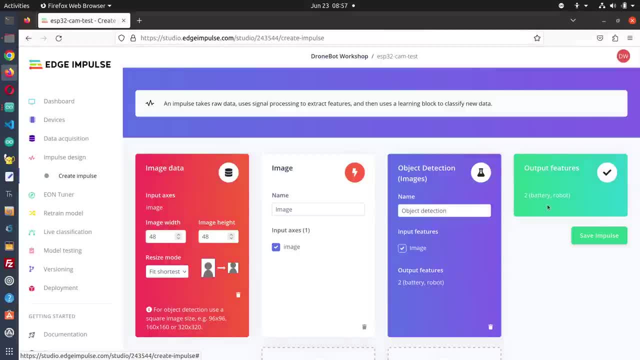 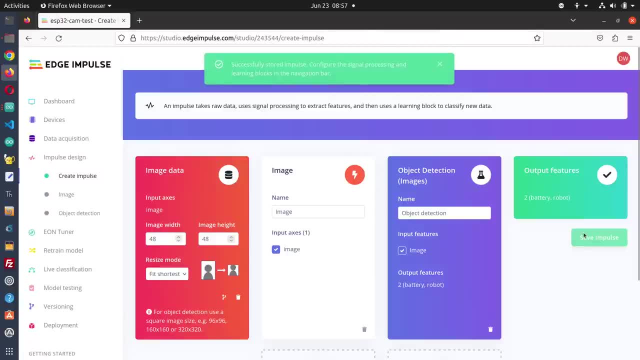 two features: a battery and a robot. so remember I had three sets of images, but the background image does not consider the feature. so now I'll go on and I'll save the impulse. and the impulse has been saved and you'll notice some other options have opened up over here. I'll go over to. 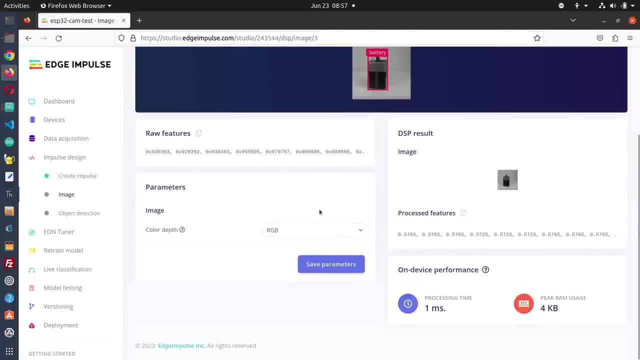 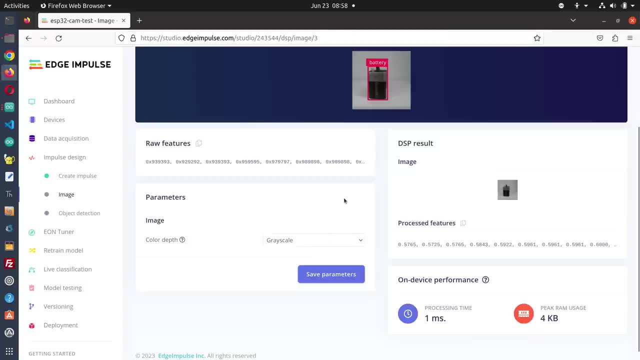 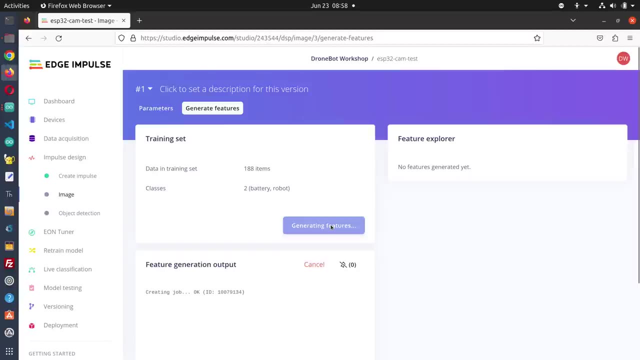 image right now and I'll look at the raw features in the image. I want to set the parameters to gray scale, because these are obviously not RGB parameters, and I'll save those parameters. and now the next thing I want to do is generate features, and this may take a few moments. 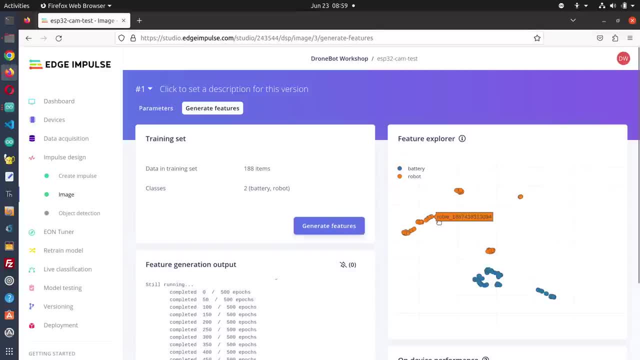 okay and I have my features generated and it shows me the feature explorer for the battery and the robot. now it's not quite as good as the one that I had with the webcam. as you can see, the robot kind of spread over to a few different places. 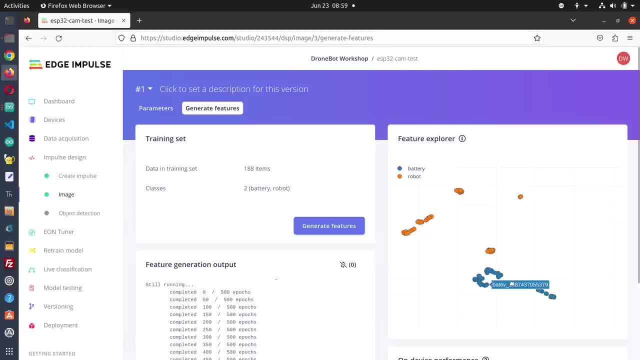 the battery is all pretty well together, but even that is in two different groups, and this just lets you know how unique it can find everything and, if you wanted to, you could create more images and continue to do what we've done so far in order to get that. 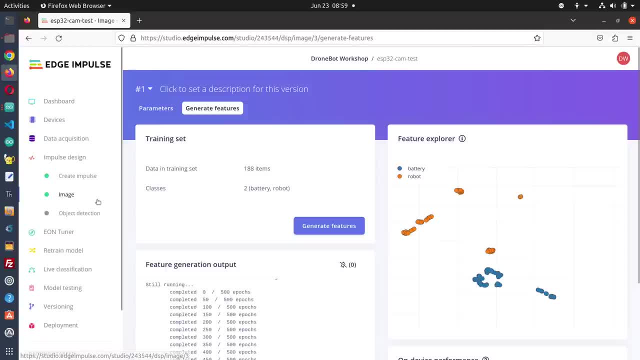 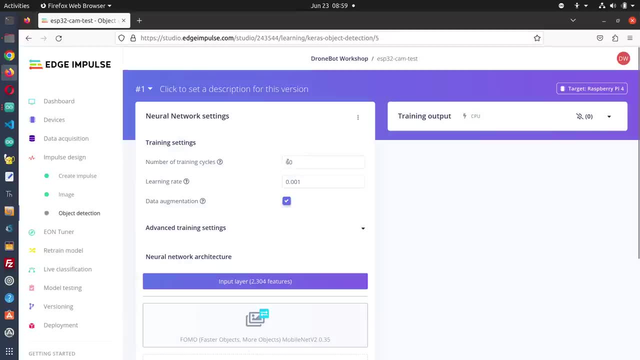 a bit better, but this should still work. so we're going to continue and go to the object detection tag. now again, eloquent arduino recommends you change a few of these settings. they say that you should set this to 30 training cycles, and point 0.005 is what they 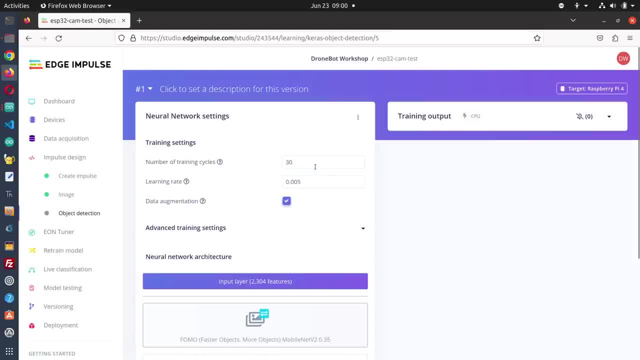 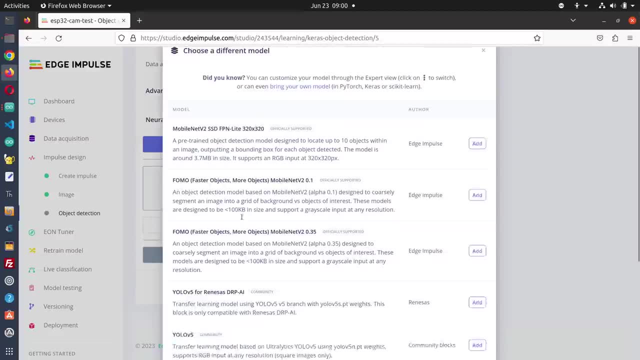 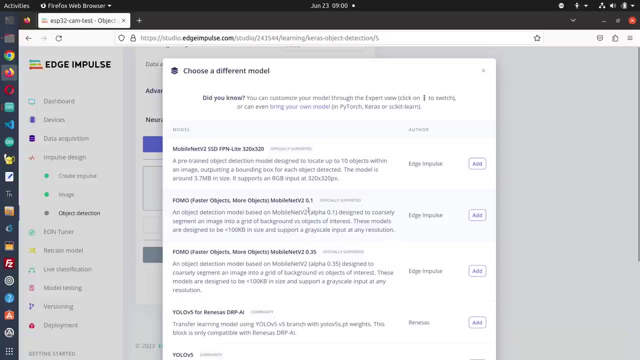 recommend for a learning rate, and you can experiment with these different settings if you wish. now you can choose. you need to choose a different model over here, because there's only one model that works with the esp32 as before, and it's this one here, the fomo one, the faster. 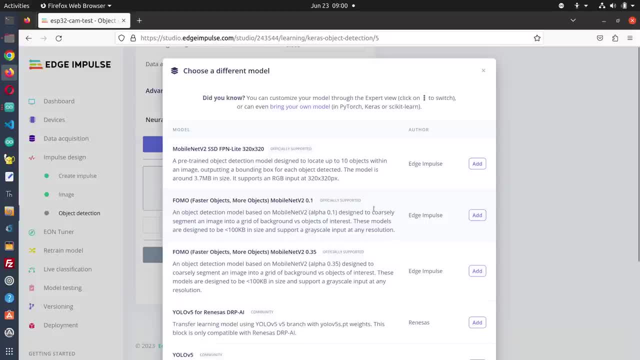 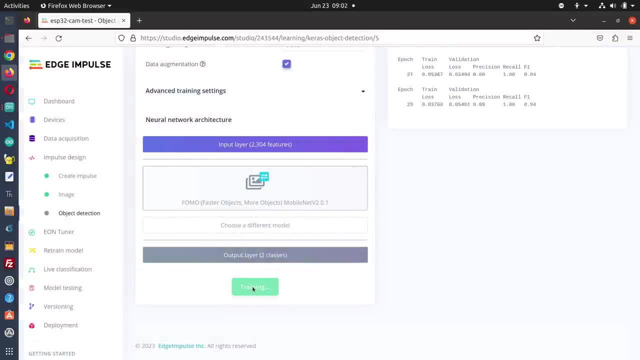 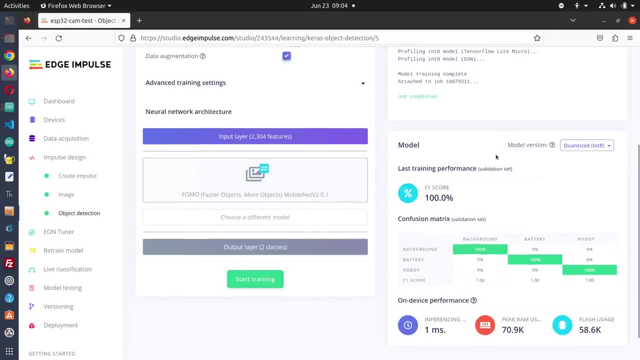 objects more object: mobile net v201. and so that's the one we want to use and we can start training that and here we are, finally completed. that took about 3 or 4 minutes and we've got a great score over here of 100%. 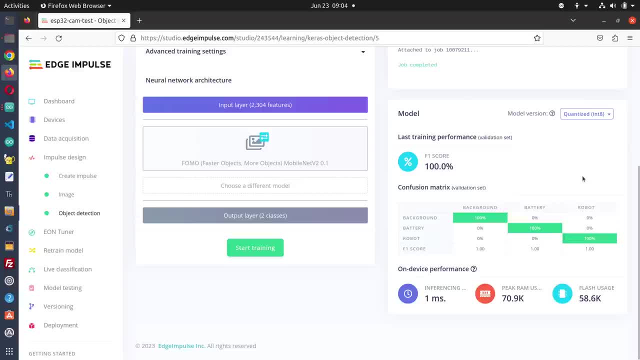 100% on our background, our battery and our robot. so it seems to really have done a very good job. and if you take a look at it, it tells you peak ram usage of 70.9k and flash usage of 58.6k. 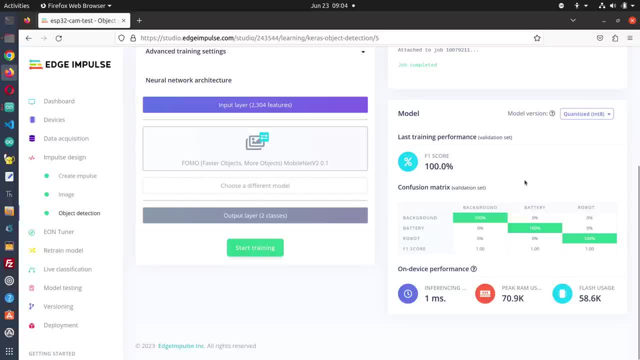 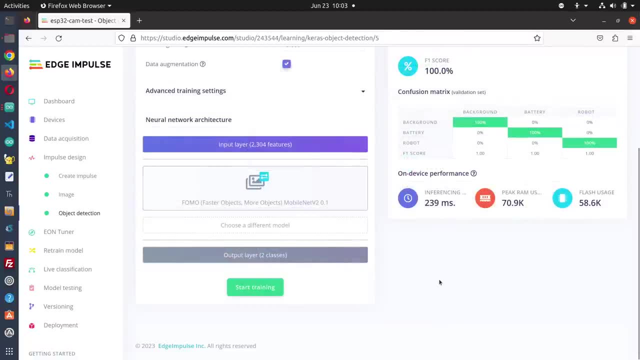 so it's a very, very tiny model, and the next step, of course, is to deploy it. now, the final step that we need to take in edge impulse is to deploy our model, and of course, we want to do that in an arduino library, so we'll go. 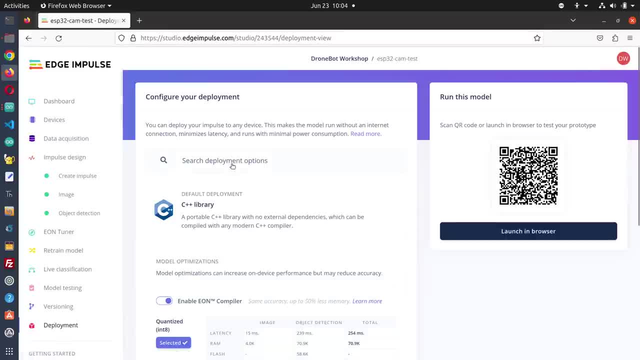 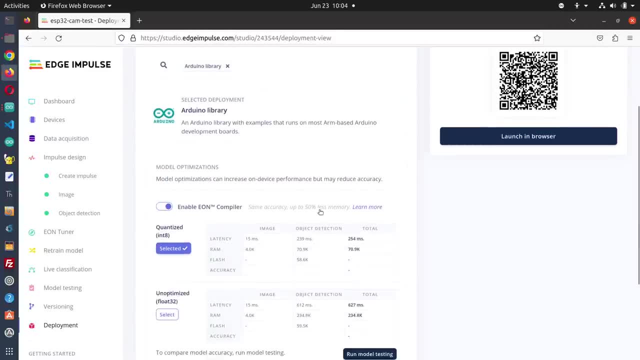 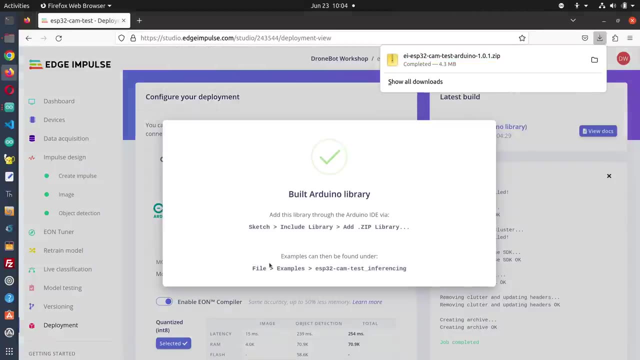 to deployment, and in deployment we'll search deployment options. just click on that and the first one is arduino library. so we'll select that. we'll leave everything else as it is and we'll click on build and the build is completed. it has downloaded another zip. 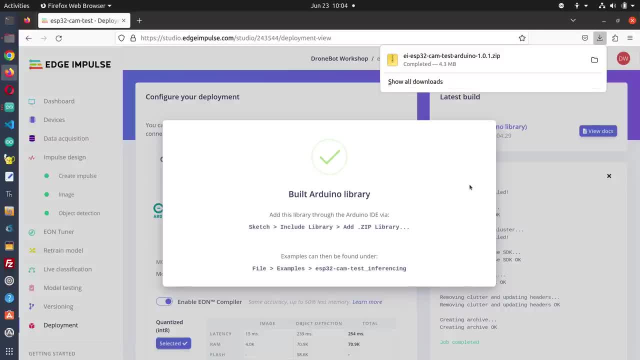 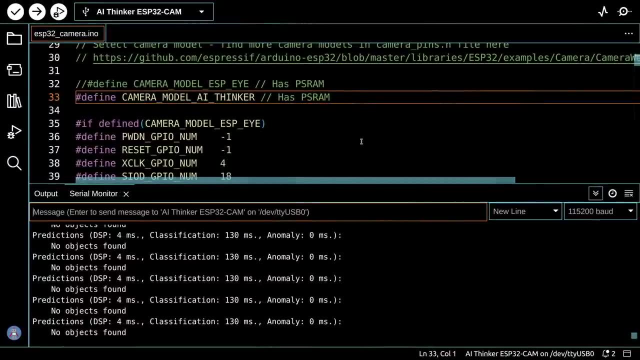 file with the library in it and we're ready to use that in the arduino ide. so i performed the same procedure with the new zip file that i downloaded from edge impulse. i imported it as a zip library into my arduino ide and then i went. 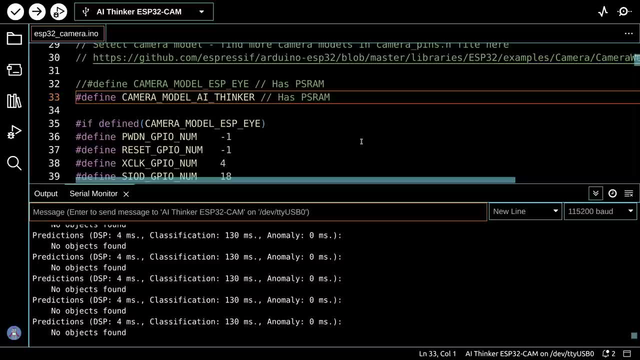 into the esp32 camera example. now, since i'm using the esp32 cam model, i had to change line 33 so i could define the ai thinker, and remarked out line 32 for the espi. i compiled it and sent it up to the esp32 cam, which i still have. 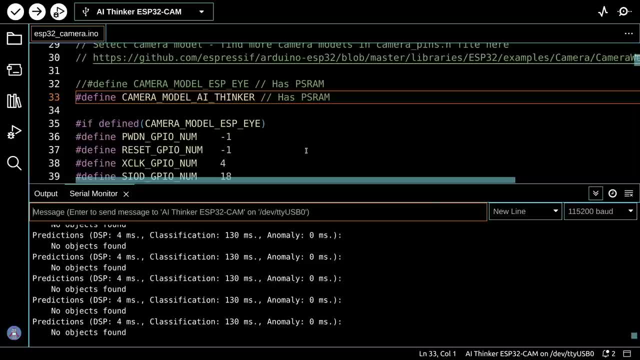 mounted the same way on the wire clip and it's saying: there are no objects found. because there are no objects to find, and so we'll put robbie in what i hope is the field of view and we see a robot with some reasonable confidence. confidence is pretty. 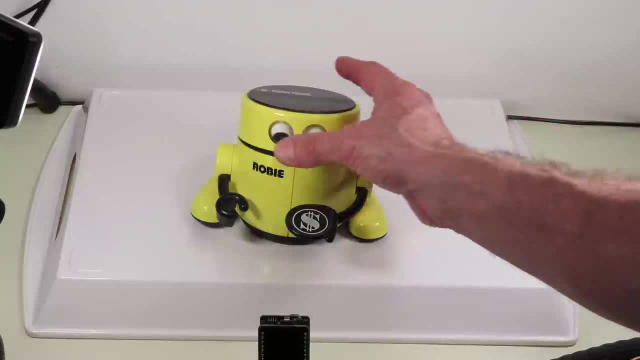 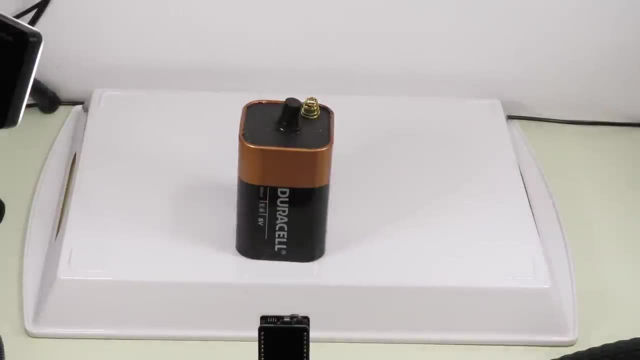 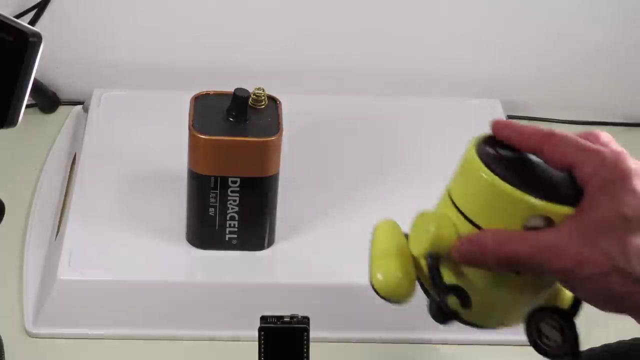 high- it's almost around 90 and we'll remove robbie and put our battery in there. and it's also pretty certain it has a battery and see if we can get both of them into the same picture. and it sees a battery in a robot with reasonable 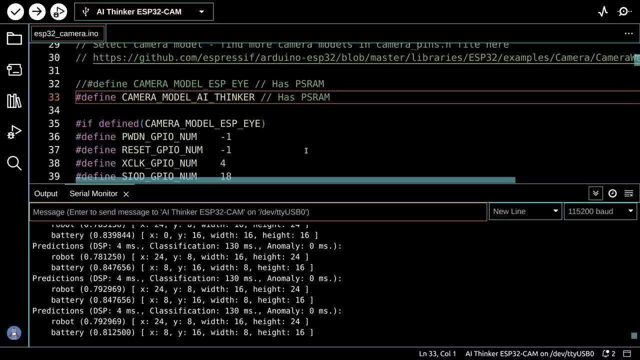 confidence a little bit lower on the robot, but pretty impressive when you consider the size of the images we used. we ended up using 48 by 48 at the very end and we used the esp32 camera in this case for both the image training and for the final object detection. 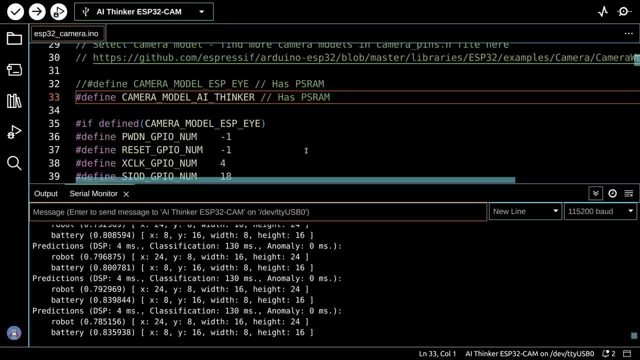 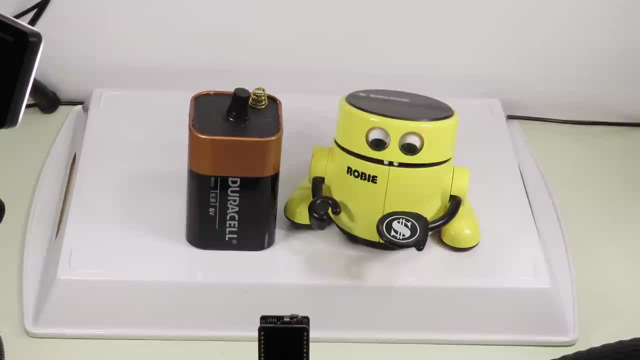 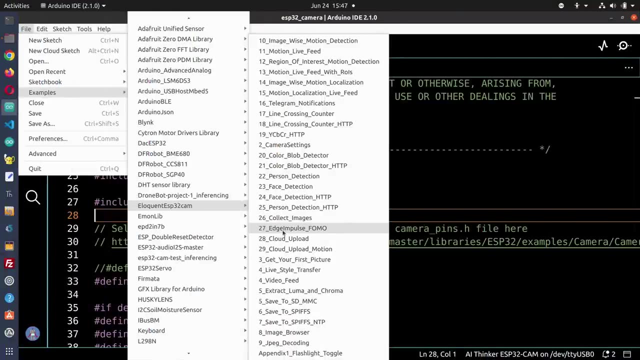 so it should work pretty well, since the setup is so consistent. so, as you can see, you can perform reasonable object detection with an esp32 camera, avoiding the high cost of other object detection options. now there's another way that we can view the results of the object that we built. 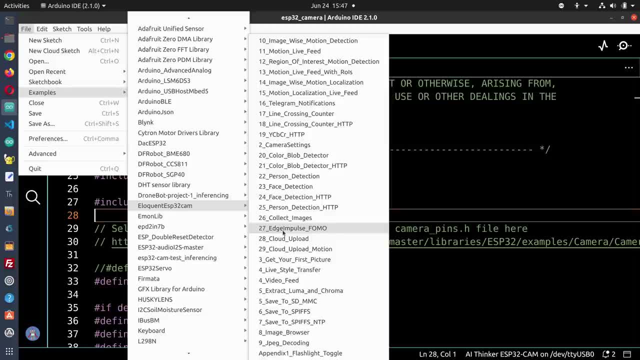 and it's a bit easier to code, for it comes with the eloquent esp32 cam library and if you look in your example sketches you'll see one that says edge impulse fomo. fomo is faster objects, more objects. it's not a fear of missing out. 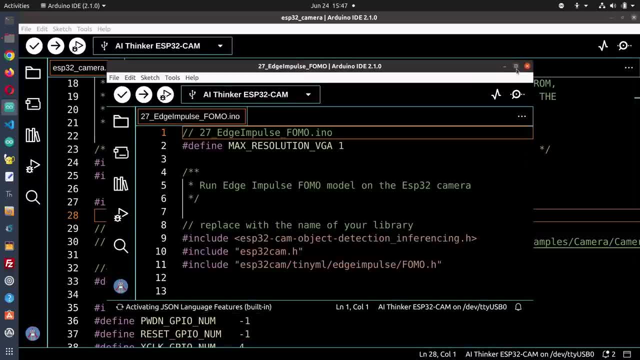 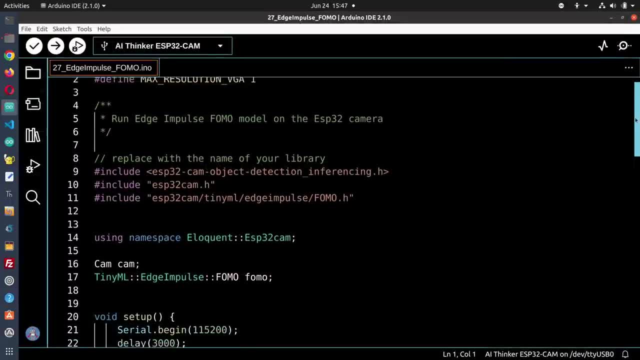 and if we take a look at this sketch, this sketch does exactly the same thing that the sketch that was given to us in the library. we got from edge impulse, except it's a lot easier to work with. if you take a look at this sketch, you can see that. 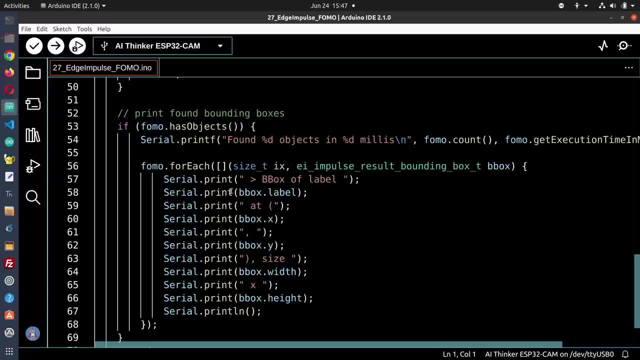 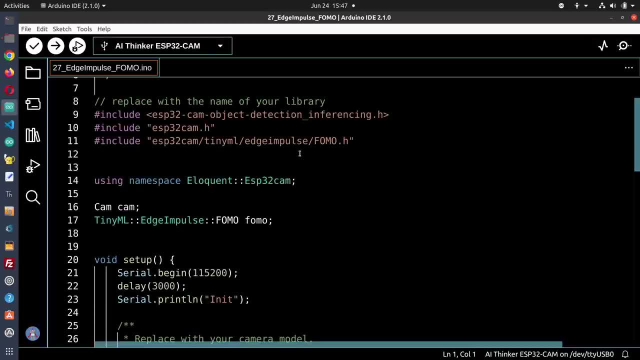 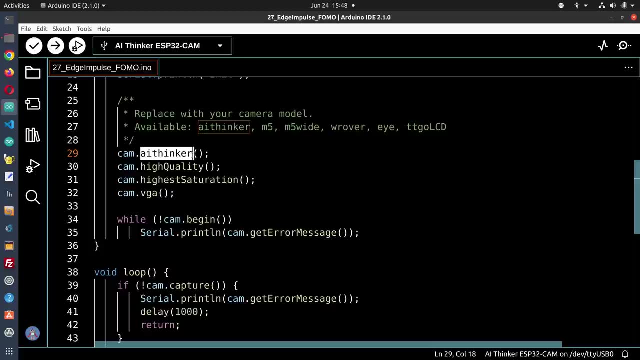 when we go over to the serial print. it's very, very easy to get data out of this and you can see there's a lot less needed to set up your camera. you literally load a few objects over here, you specify what type of camera you have. so this is the ai thinker over here. 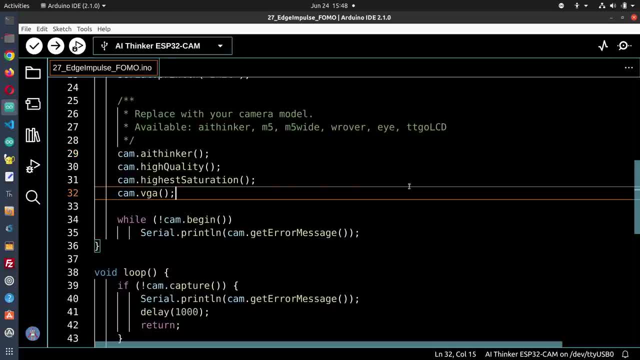 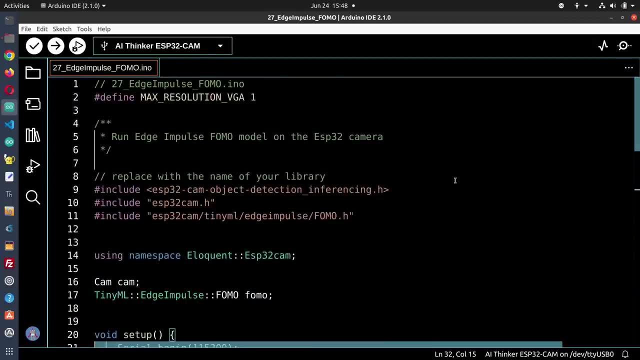 you can also replace it with one of these other types of cameras. you can set things like the quality, etc. and it's very easy to use, and that's one thing that this library makes things it's easy to use. now you do need to modify this, of course. 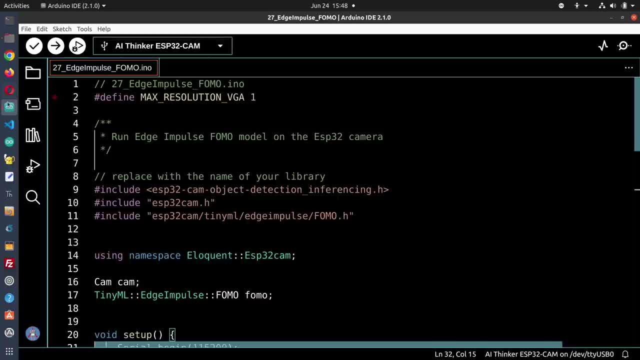 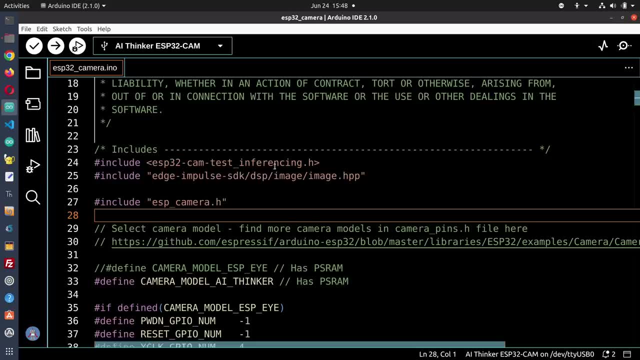 in order to work with the data that you just built, and what you need to do is to go into the sketch that you got from edge impulse- and i'll go into this one here, the esp32 camera one. and if you take a look at that first library, 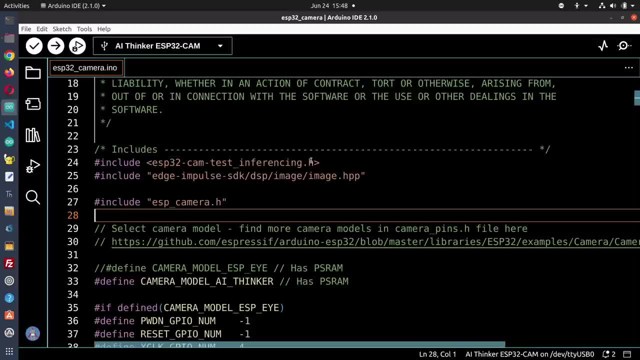 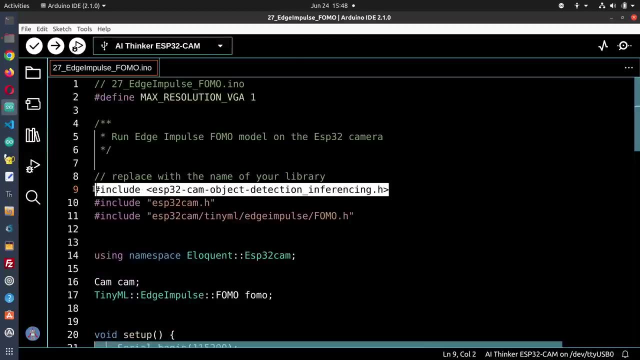 they're including. this is the custom library that has the data that you created for the object you built, and so the best bet is just to copy this entire line over here and then go back into the other sketch and replace the top line here with the line that you just copied. 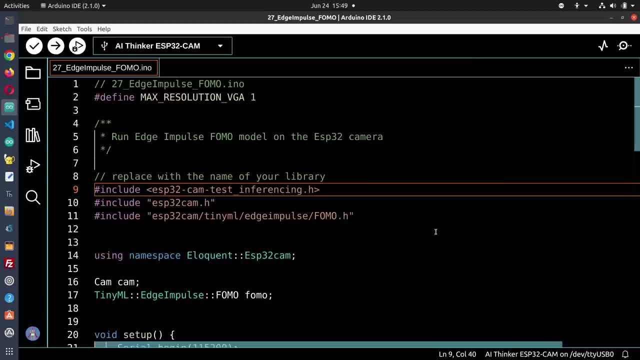 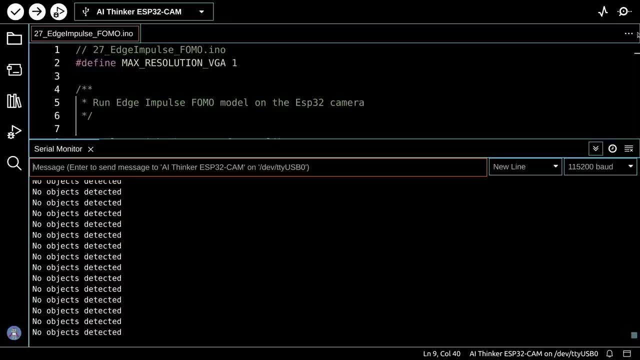 and now it'll contain your data so you can compile that and load it up to your esp32 cam and give it a test. and so i'm running the eloquent arduino code on the esp32 cam and it's using the object model that the esp32 cam 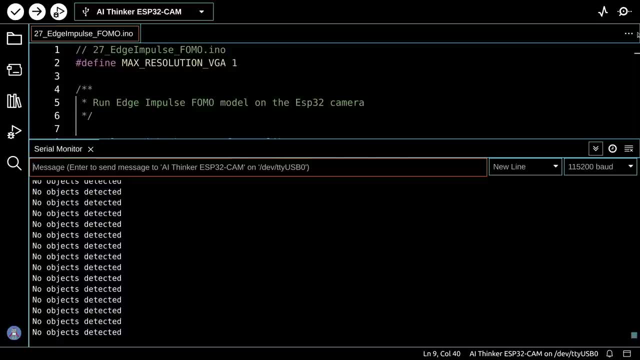 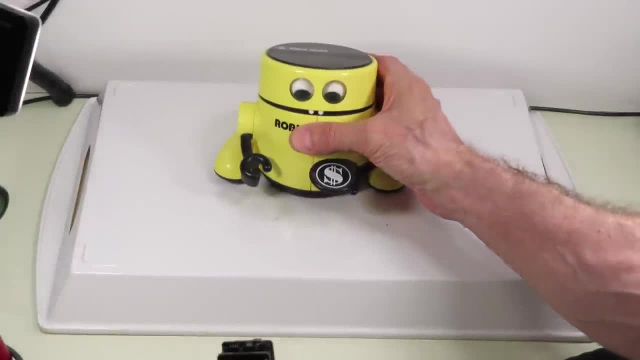 was used to train in the first place, and so the serial monitor is telling me there are no objects detected, which makes perfect sense, of course. as there are no objects, let's put an object in its field of view and it sees a robot, and it's telling you how quickly. 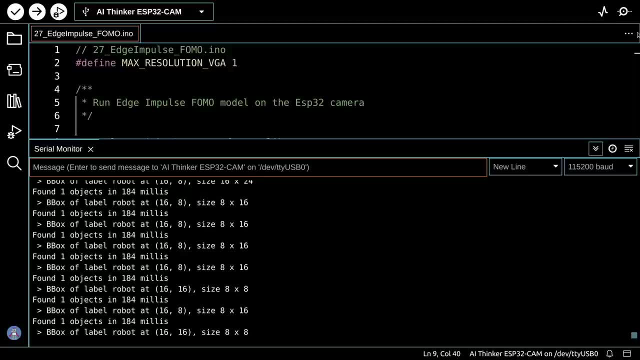 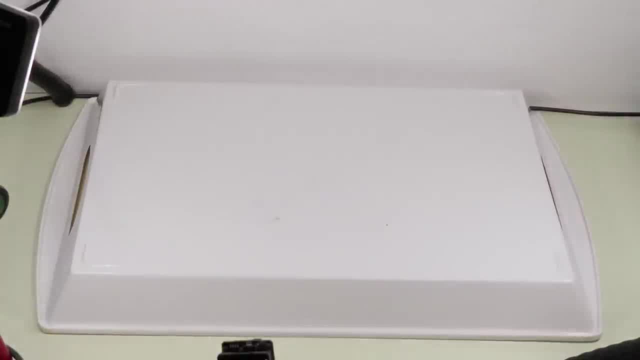 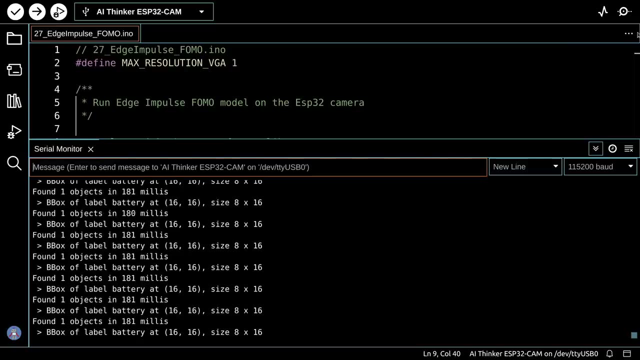 it did it 184 milliseconds. pretty good, gives you the location of the bounding box as well as the size of it. i can take my robot out and replace it with my other object and it sees the battery. that seems to work pretty well and we'll see. 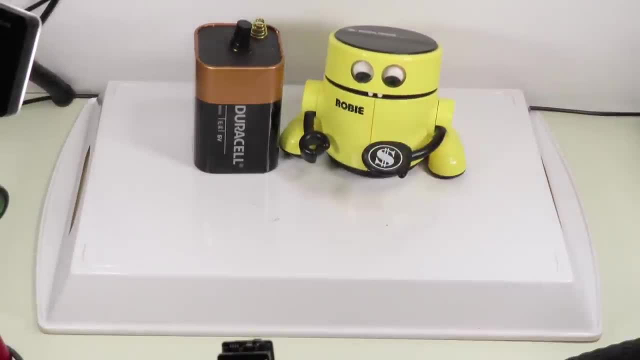 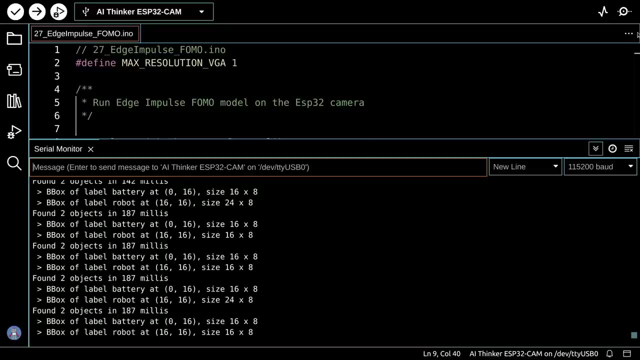 if we can see both of our objects, and it sees both the battery and the robot. so this does seem to work pretty good and if you looked at the eloquent arduino code, it's a lot easier to use than the code sample you're provided with from edge impulse. 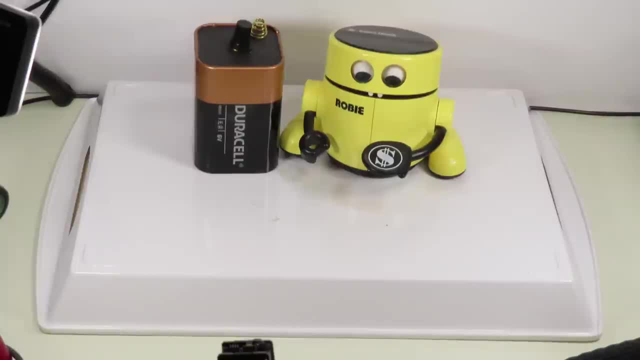 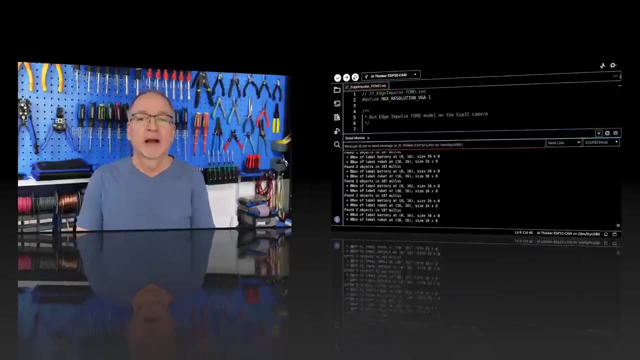 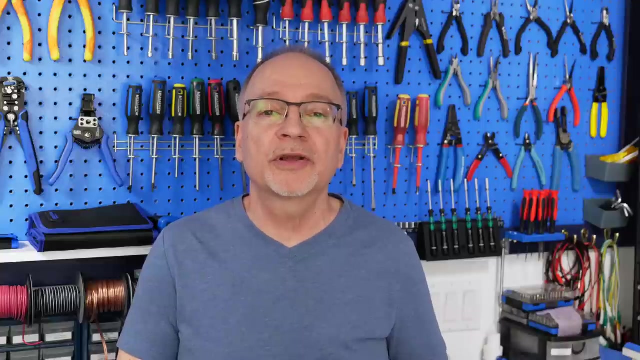 but by using edge impulse and perhaps the eloquent arduino library as well, you can build some pretty impressive object detection projects with the esp32. okay, that wraps up our look at object detection with the esp32, and i hope that it has inspired you to start using object. 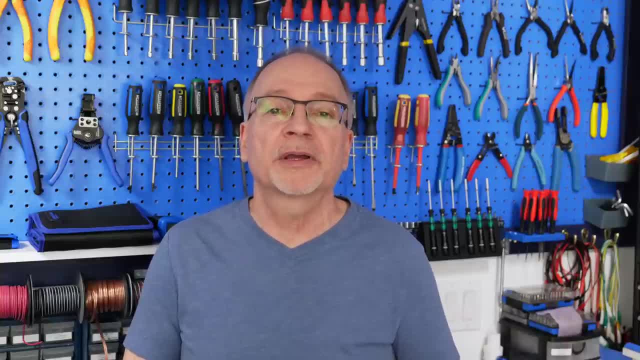 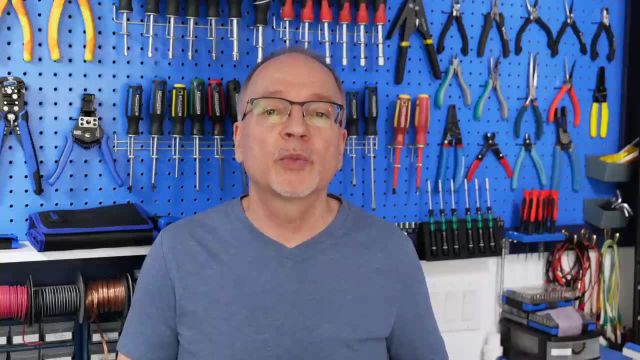 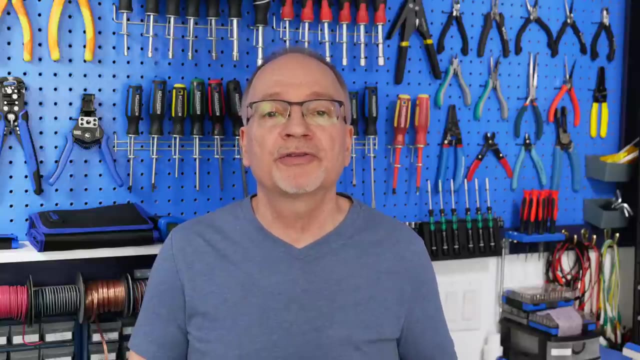 detection in some of your own projects. another thing i think it should inspire you to do is to learn a little bit more about using edge impulse. remember, edge impulse doesn't only work with video signals. it can also use audio signals and even analog signals, so there are a lot of interesting. 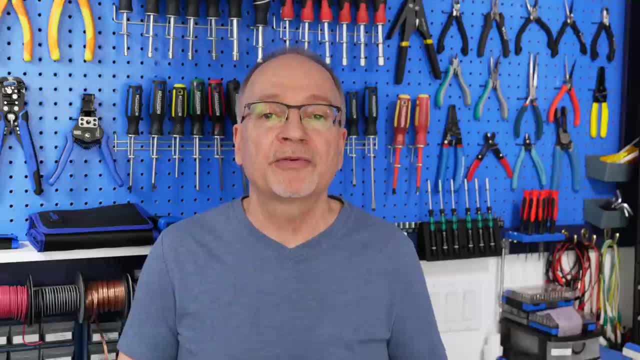 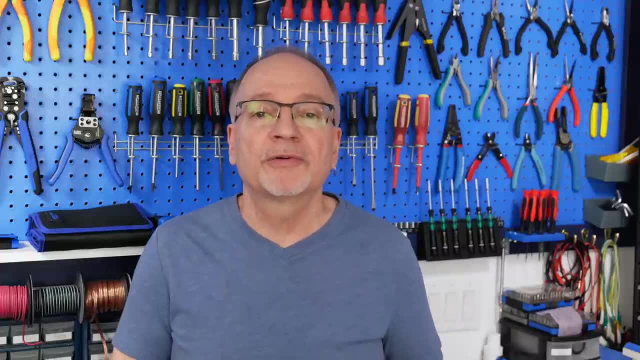 applications that you can use edge impulse for, and the free account that you have can accomplish quite a few things, so it's a good product to check out now if you want some more information about doing object detection or using the edge impulse if you want to get the step by. 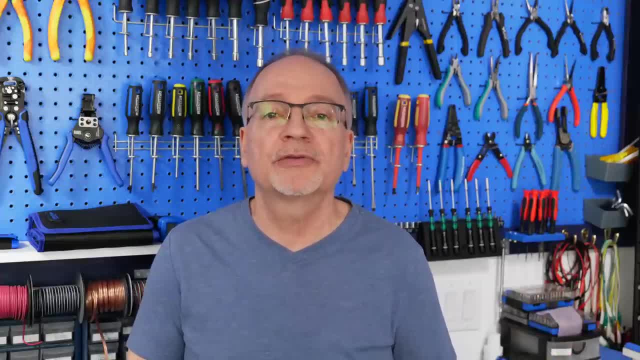 step process. you can just check out the article that accompanies this video on the dronebotworkshopcom website and of course, there's a link right below the video to the article when you're on the website. if you haven't yet, please sign up for my newsletter. just my way of. 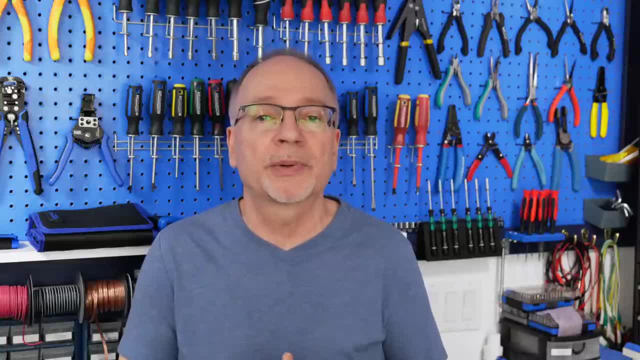 occasionally letting you know what goes on here in the workshop, and all i need from you is your email address for that. and if you want to discuss object detection or anything else to do with microcontrollers or electronics, head over to the dronebotworkshop forum, where you'll find a bunch of 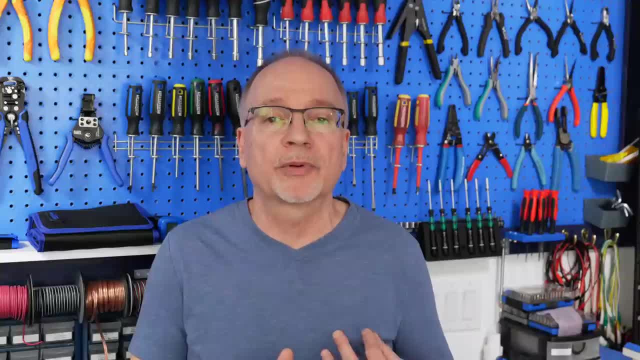 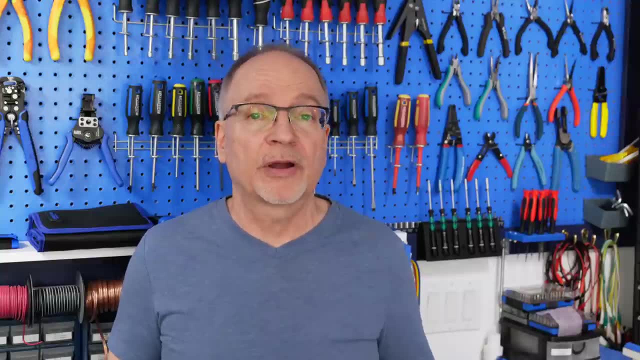 people who will help you out with any problems you're having with your projects and would love to hear about the things that you're working on. and finally, if you haven't yet, please subscribe to the youtube channel. i make videos about electronics and microcontrollers and if you enjoyed this,